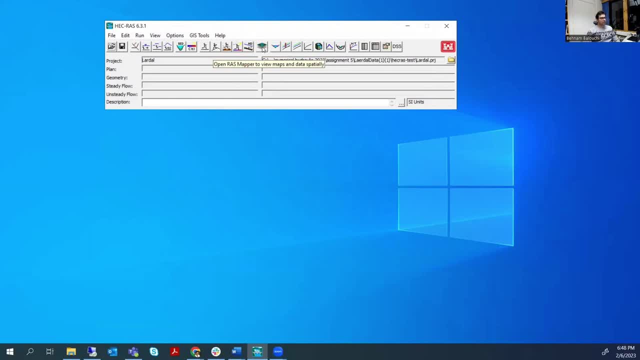 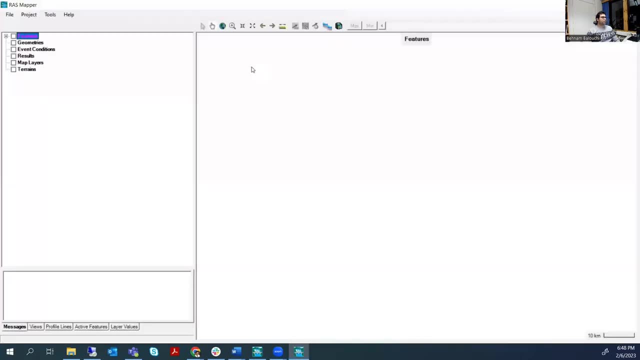 So for a starting we should go to the last mapper, after also checking the unit as we discuss about it. The unit should be SI. So here For 2D modeling, we should introduce terrain and first, as you see, we have a message to add the projection file here. 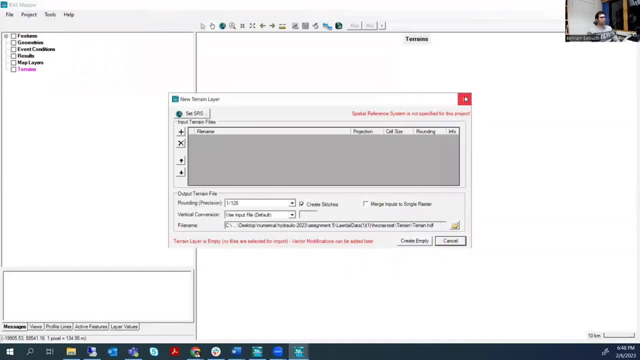 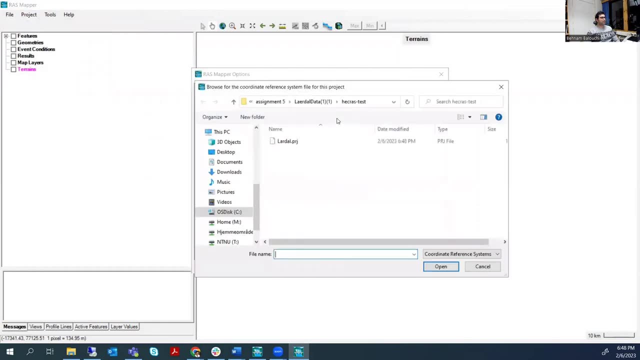 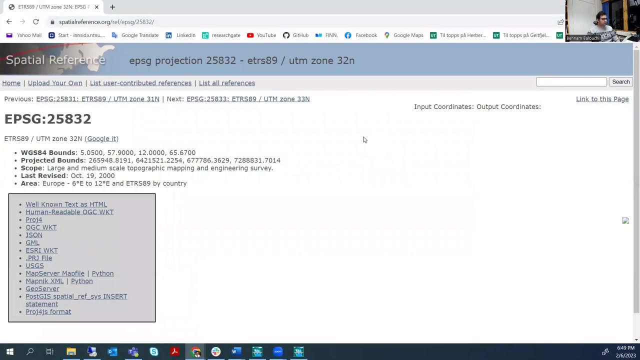 We can have the projection file or you can go to the just projects, that projections. This is the projection that we have and you can see the zone is 32 and, as I mentioned before, you can also find any projection file. If you have any problem with your projection file or if you want to search for your projection file, you can just go to this website, a special reference, that orgy, and then search your name, for example. 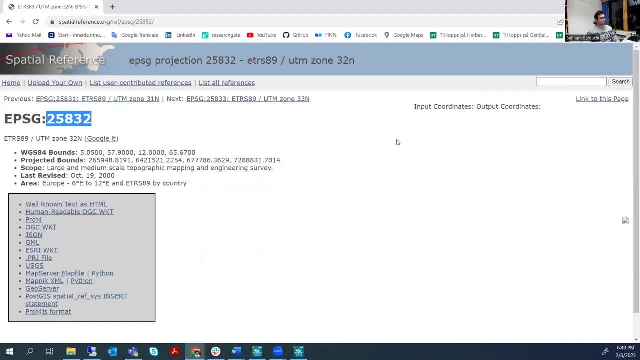 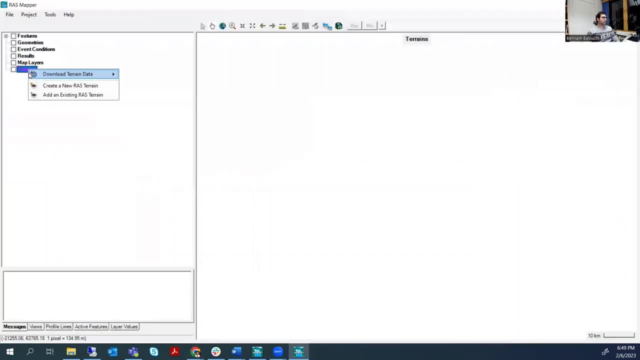 Or if you have this number, you can search It. Or if you have the UTM, for example, this one, you can search it And you can find then. you then go, you can find a new projection file. then go to the terrain, create a new restrain to introduce your TIFF file. 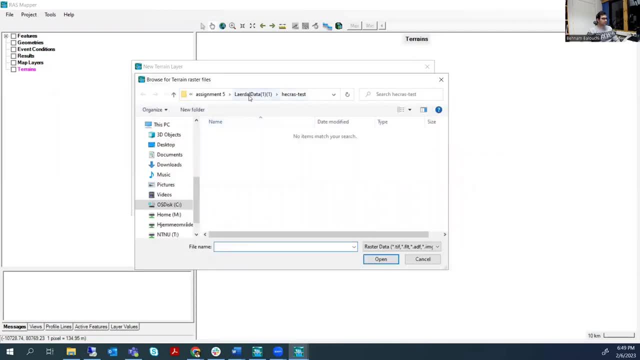 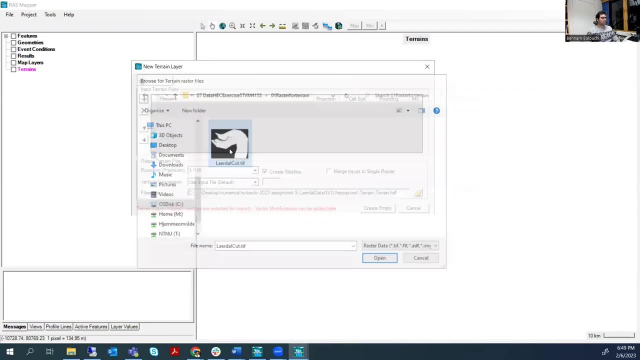 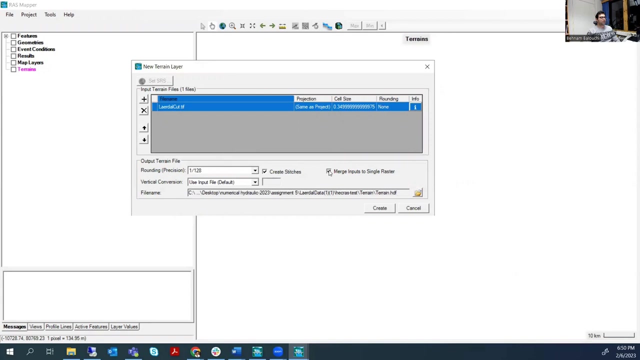 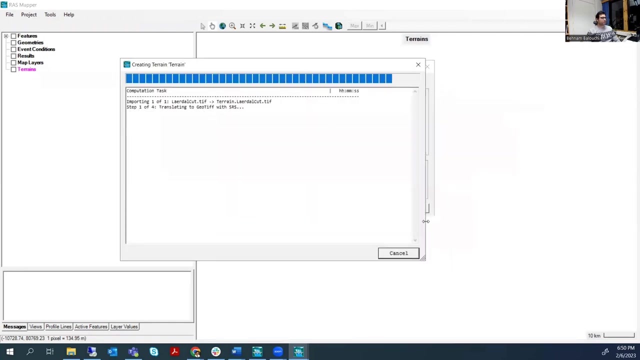 Here you should go to the last and come here You have a TIFF file. If you have more TIFF file, you should add all of them and then take the merge Input to single, single, single raster, then create it. It takes a little time. 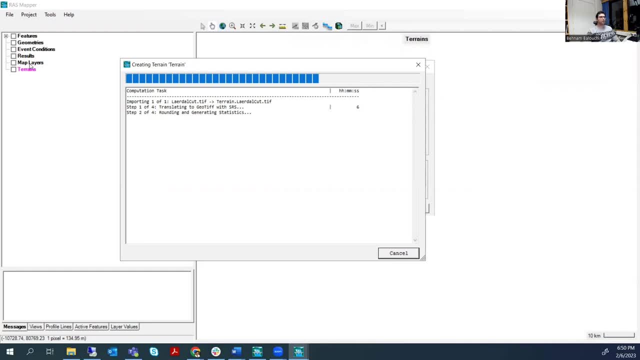 Then after that you can go to the map layer and you can add the Google Image or Google satellite and also add other points that you have or other layer that you need And, as I explained before, in the geometries you can see the geometries, input and your mesh and in the results, after you run the model, you can see the results. 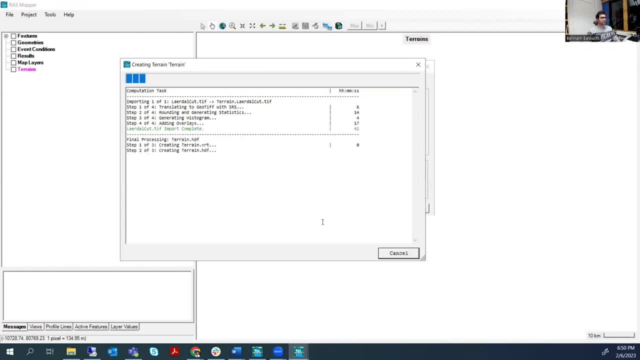 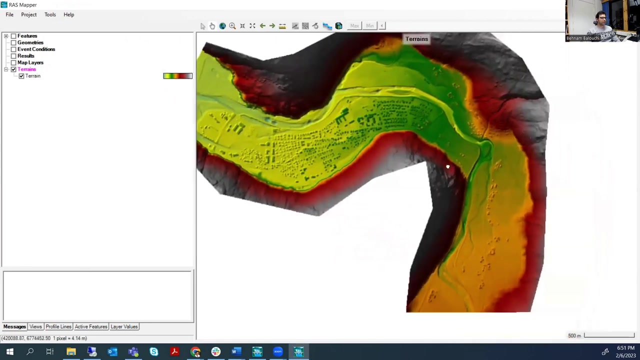 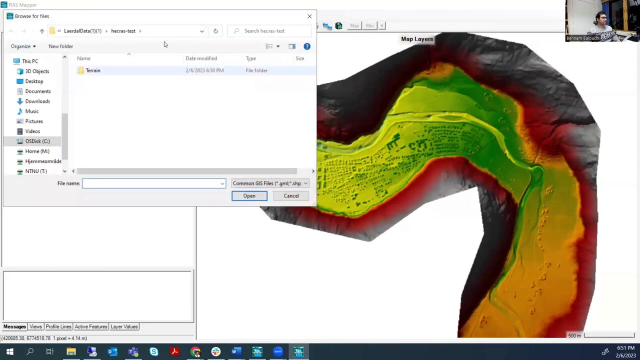 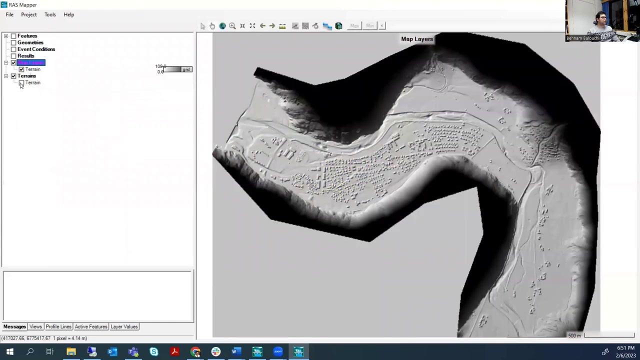 So now it's Finish, Okay, Okay, And you can see the viewer that we have. So then I'm going to the, For example, add reference. If you want to Add the same train As the terrain that you have, you can add a layer here. 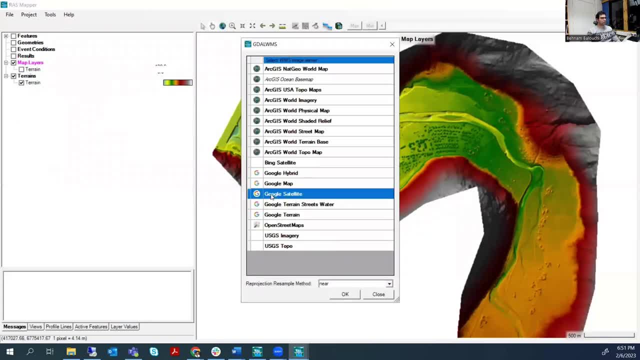 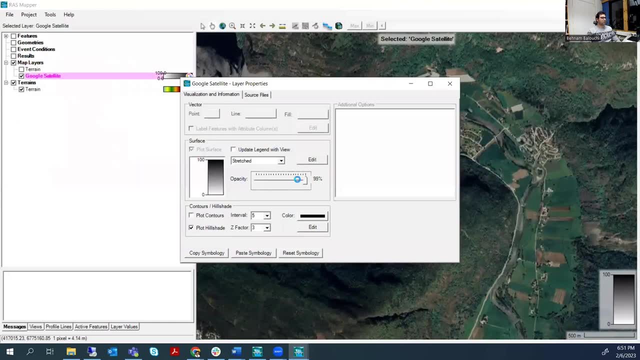 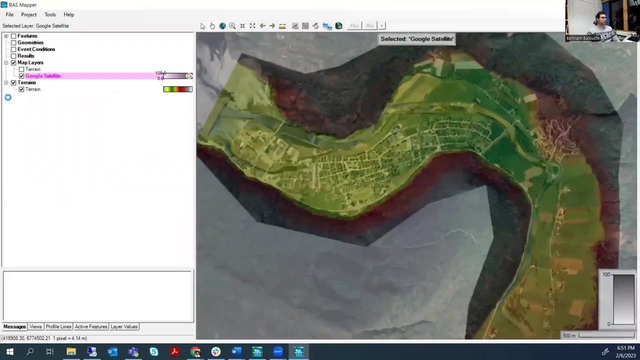 Or if you want the image, you can go to the Google satellite, For example, and then add. You can see it in the options. you have some options like capacity. you can Change the capacity. You can see the overlay of the images. 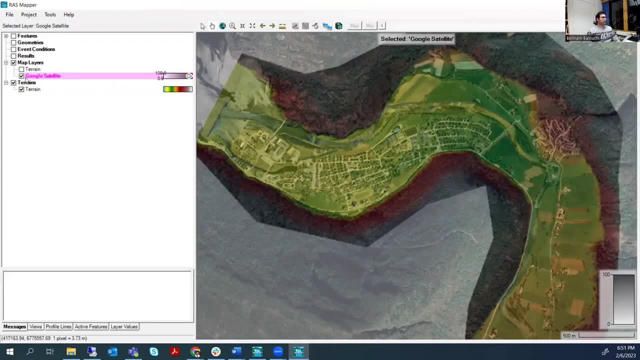 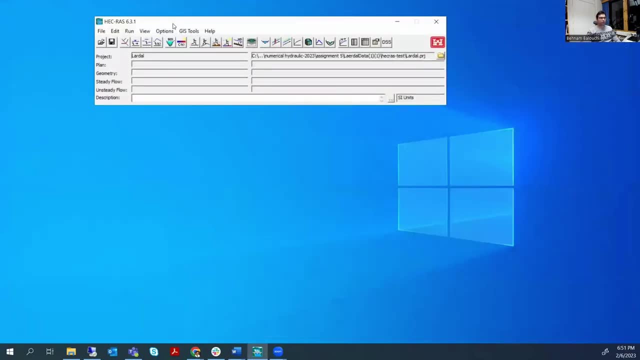 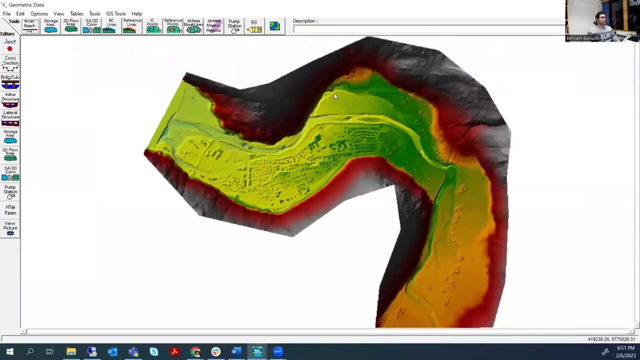 And then save And exit. then for introducing the To the fellow mesh, we should go to the geometry here Or edit geometry. Now we should introduce a 2d fellow area, So we click here and introduce the area that we want to model, the area that we think it's affect from our flood or from our maximum flow that we have. 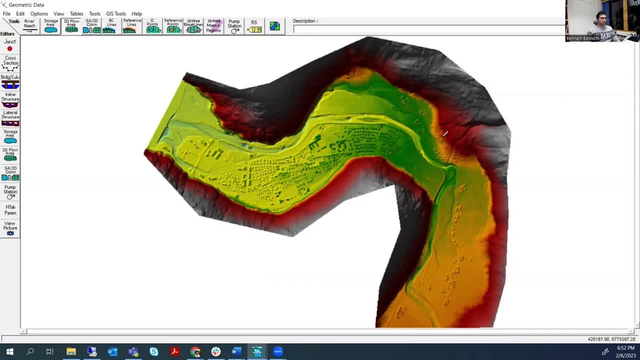 So, for example, I like to model From here, So, So I try to Make a Zoom like these, And then, as I want to be a Short one, then I just make like this. it depends on you. For example, I make it a big one now. 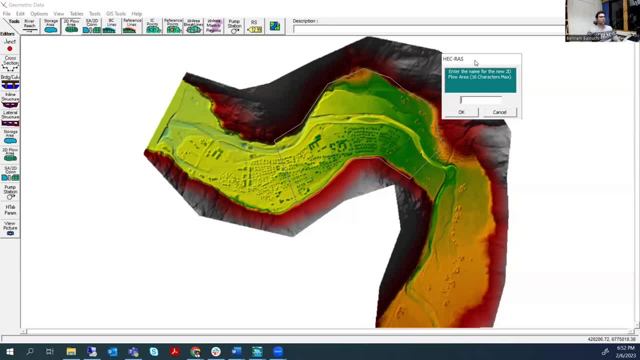 To be sure and also fast, But you can use the real And accurate data. So now it's a geometry, For example. I just wrote the geometry, Or I can Write it like, and then Okay, if you are coming here to the. 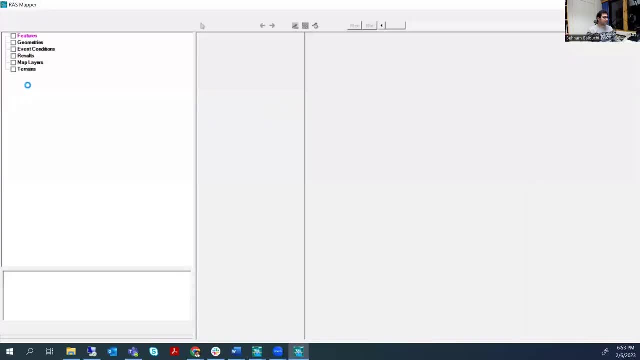 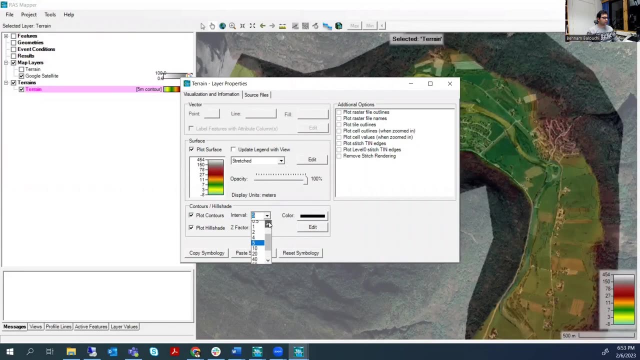 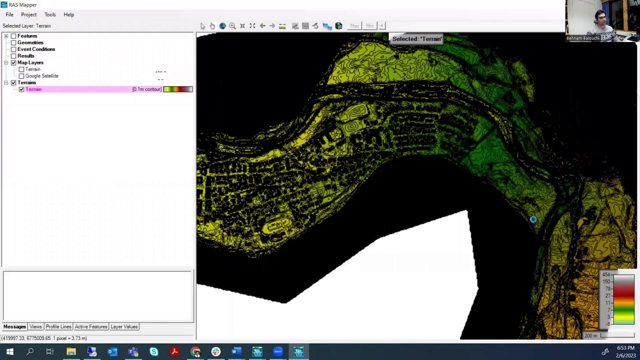 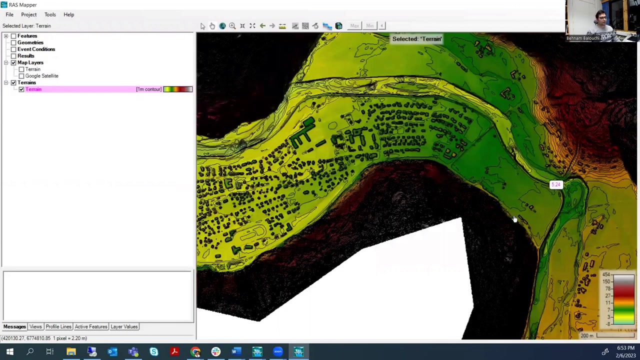 Press mapper. You can go to the plot contours and make it as Something like this: Now you can see the Area that you have. I think We should increase it a little. Yes, now you can choose the center line of the river, if you want, or the banks, easily. 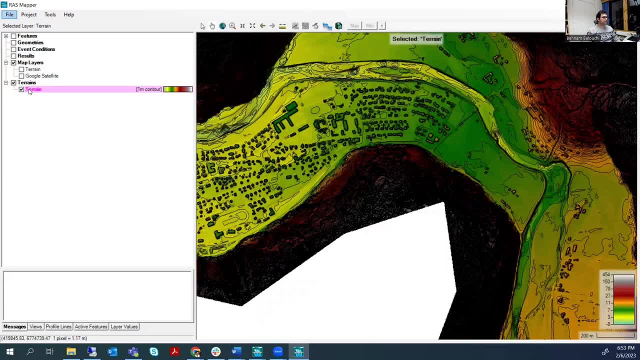 By this. but as we don't need it, then I turn it off. but when you want to draw a bank or any line, I recommend to. But as we don't need it, then I turn it off. but when you want to draw a bank or any line, I recommend to. 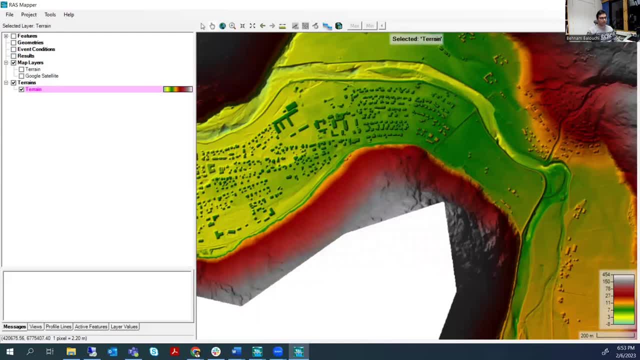 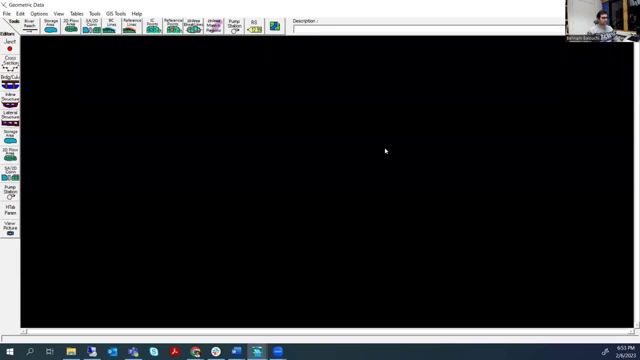 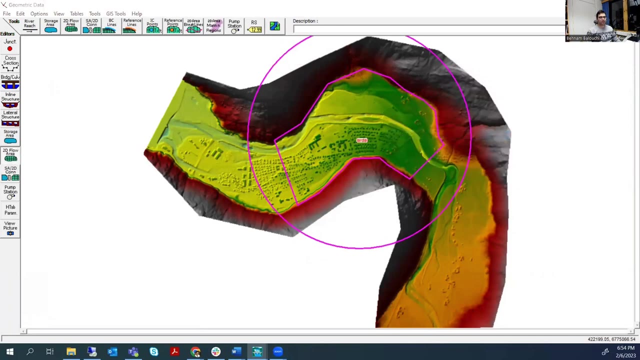 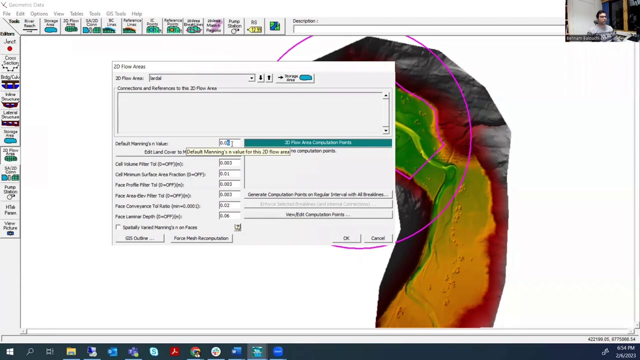 But when you want to draw a bank or any line, I recommend to Turn the control lines on. And then we left click and go to the edit below area. Here you can see the money and value. we should calibrate this value or we should. 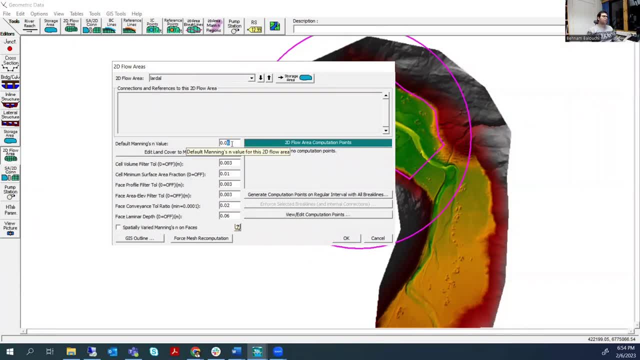 Measured or compute the best value of money roughness that we have. We can use the Money and value as you can see point zero six or point zero four. It depends on the case that you have And for your mesh. 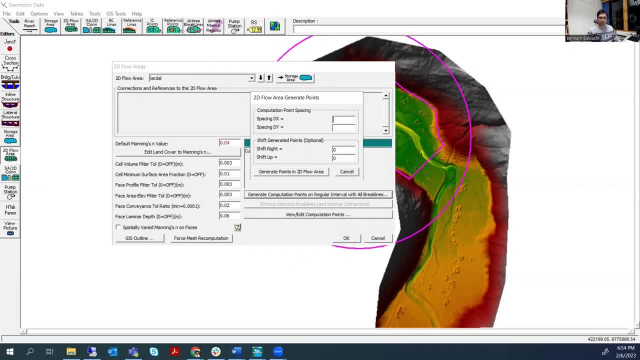 We should here introduce the mesh. I just use it ten by ten. Again, it depends to your accuracy and your model. You can increase it or decrease it, But as I want to be fast and almost good results, so I keep it as ten. 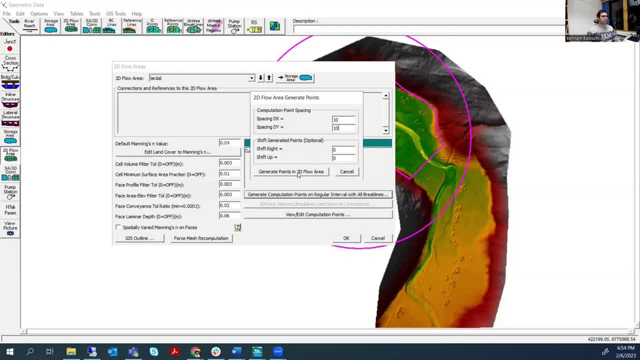 But as I want to be fast and almost good results, And that's the water surface, Şıkkı, Fiko, The, And then the important things: force mash computation. Here you can see the information about Dimash And then OK, so now you can see the mesh. 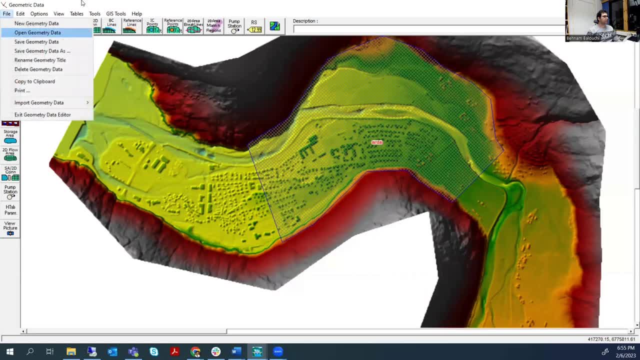 Here. So then we should introduce the boundary condition lines. You can see BC lines here For the boundary condition lines. you can get these area, for example, as we know the river are here. Just look at how I introduce it. So it's the upstream boundary condition. 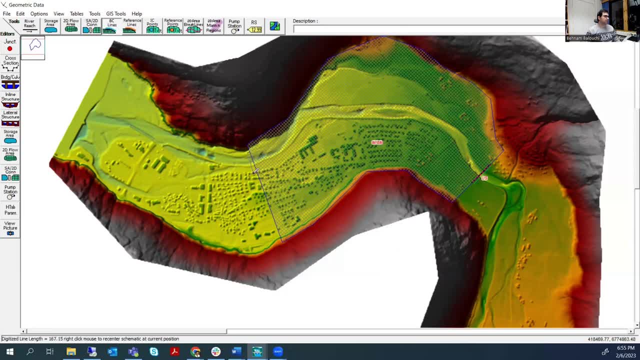 And we need another one, So it's a downstream. If you think you have water also here, then you can also introduce it as a downstream that area. We have here more important options like 2D area break lines. I will talk about it at the end of the video. 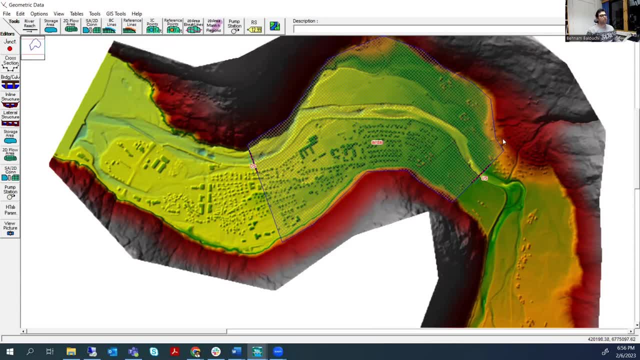 And also the 2D mining regions, If you want to. If you have Mining layer- for example, you measured mining roughness along the river in various locations that you can see- Then you have a mining layer and you can introduce the mining layer to the model. 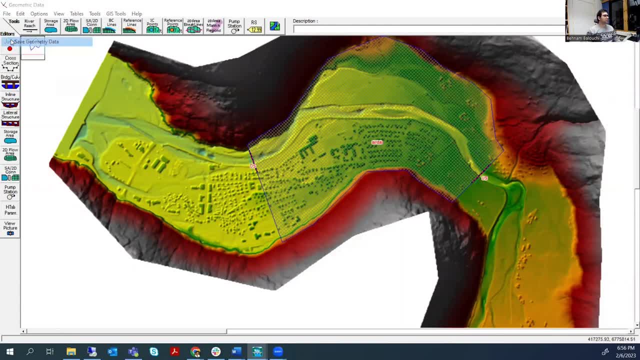 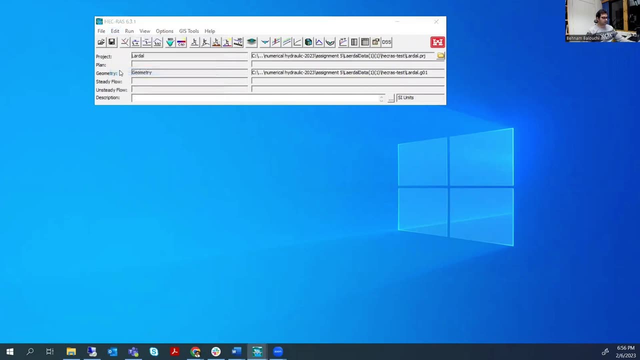 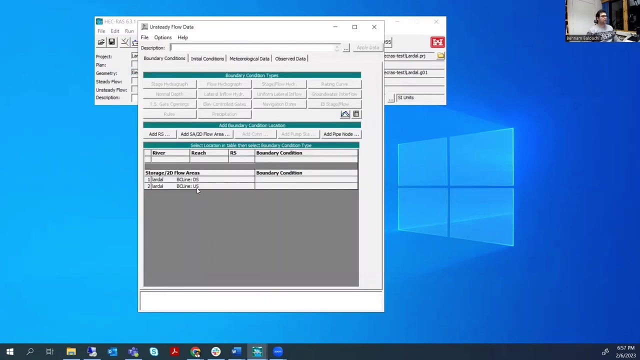 And it's really increased the accuracy of your results. Then I save the geometric data. You can name it like geometry And then OK, Then close it. Now we should introduce The On a study below data. so we are Here and we can see we have a upstream and downstream data. 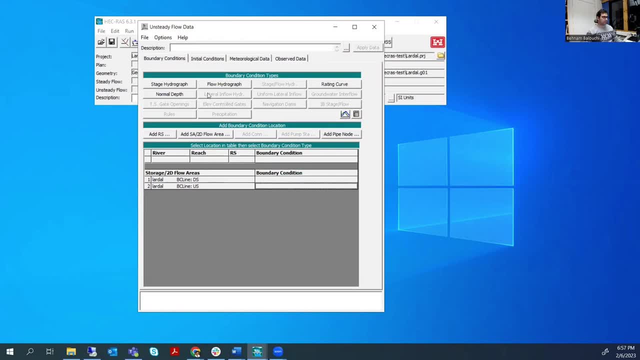 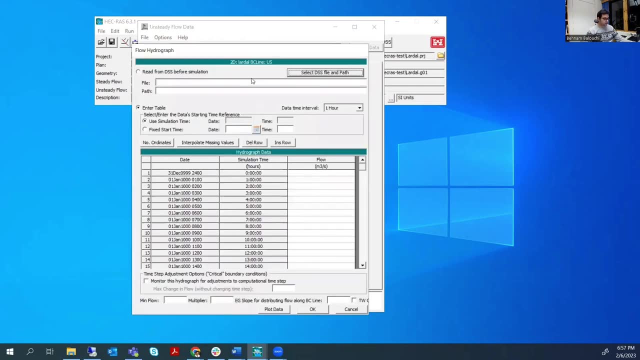 For the upper stream I. it depends on your project, but we can introduce a fellow hydrograph as we have a discharge hydrograph For the upper stream. it depends on your project, but we can introduce a fellow hydrograph as we have a discharge hydrograph. 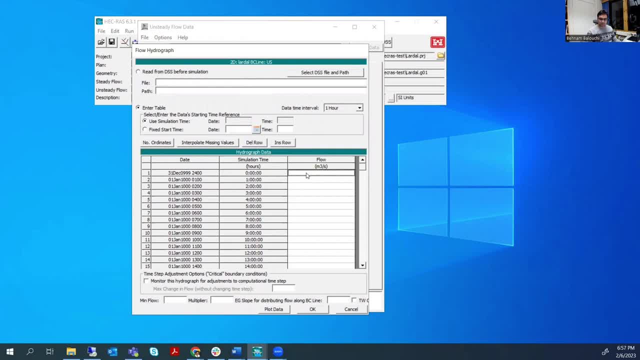 So we need to introduce a fellow hydrograph, as we have a discharge hydrograph. So here we can start from A 65- 65. So we run it for the discharge of 920.. And then Here we need to introduce the. 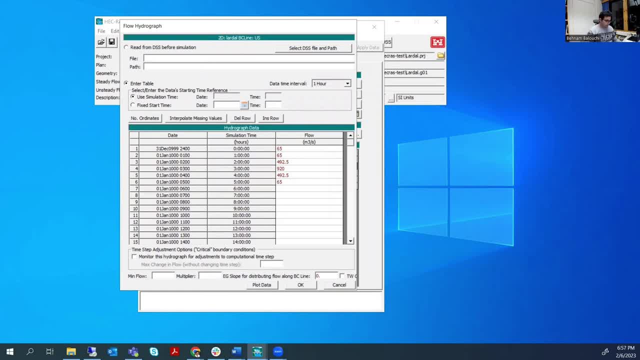 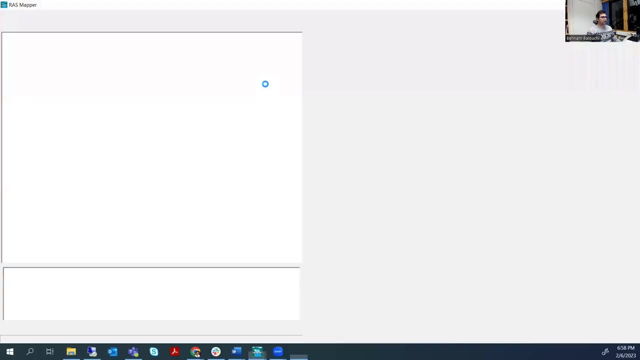 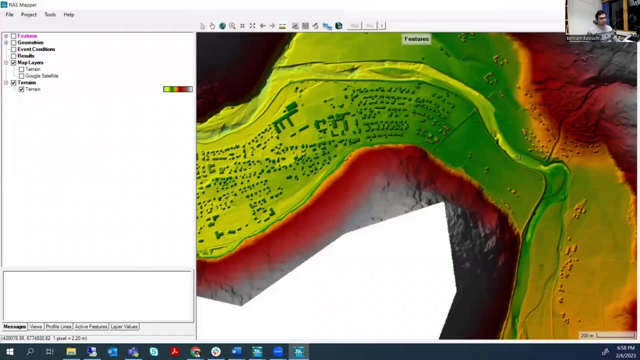 a slope. so we assume the slope is 0.01, or you should compute it from the rust mapper and then, okay, if you want to see the slope, you can come here. so this is your river, just go to the ruler and then. this is a easy way to show that. 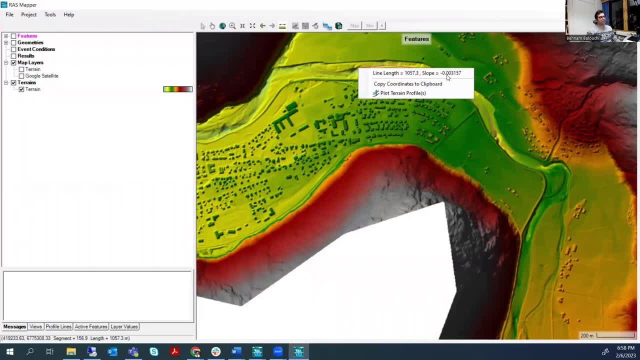 but you should be careful, it's not. you can see the slope is 0.003, but it's not accurate because i just draw it without any details. if you want to draw it, you should, and also you should take along the rivers to see the slope that you have. so but one easy. 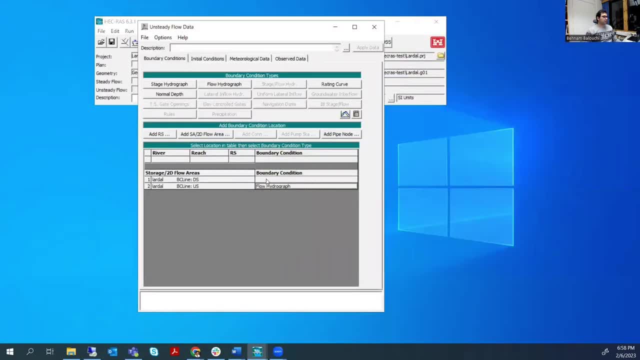 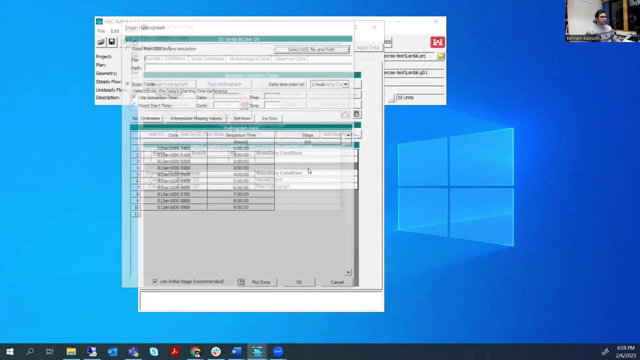 way. is this okay here? then then for the downstream, you can have a normal depth. if you choose the normal depth here, you should introduce the slope that you have, or you can introduce a stage hydrograph. so here we have a message that you introduced normally. do you want to change it? yes, we want. 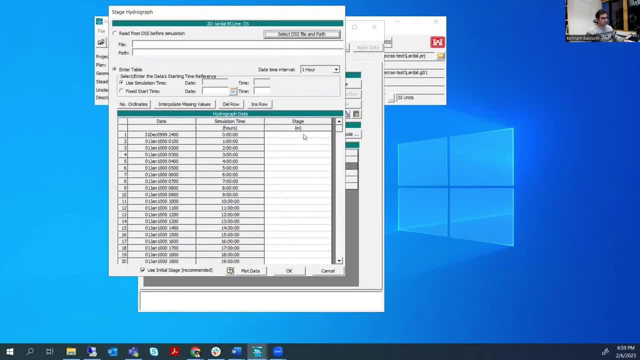 to change it to the depth and then for the depth, you want to have it as a 1.24, so 1.24. i just copy paste it for some values. you can assume that your water level is constant or you should introduce a normal depth. 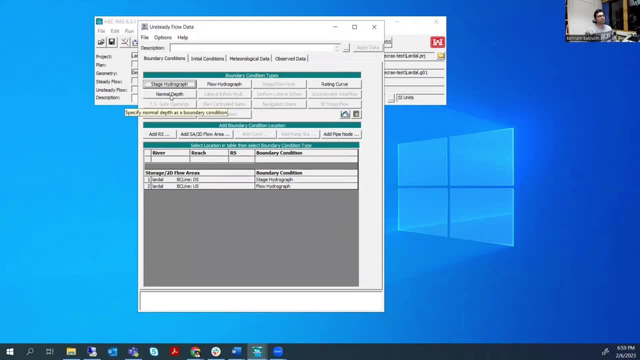 I recommend to use the normal depth if you don't have a specific data, because according to the changing of the discharge, the water level downstream should be changed. It depends to the case that we have- if we have a backwater, for example. 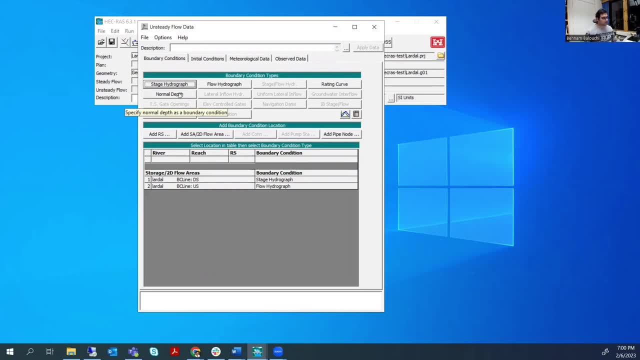 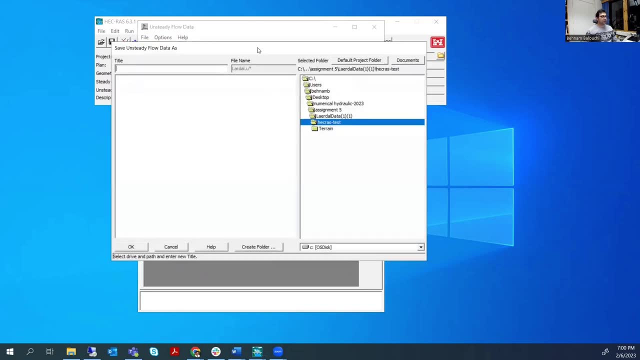 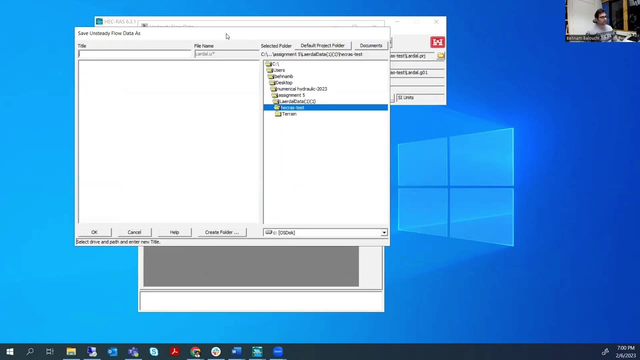 downstream we have a sea or ocean, it's maybe we have a backwater. So we should be careful about these data because after running the model then we should calibrate the model. And calibration- we should have some measured data from the field. 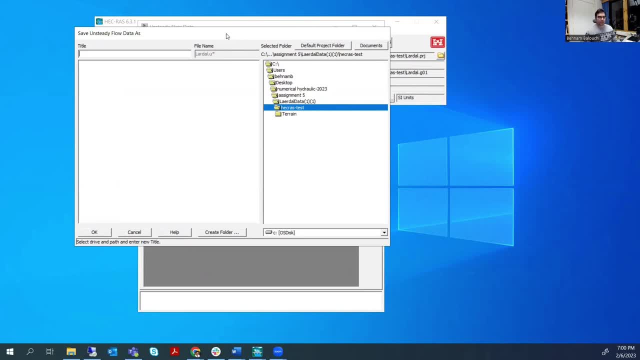 I don't use any measured data from the field in this example, but you should find the measured data and calibrate your model by matching or having a good agreement between the measured data and your model data. So I write it as a Q of Q. 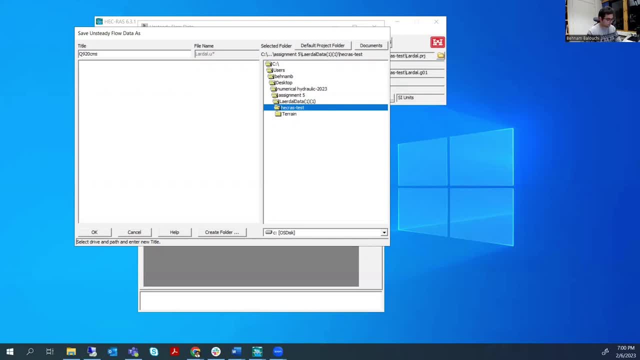 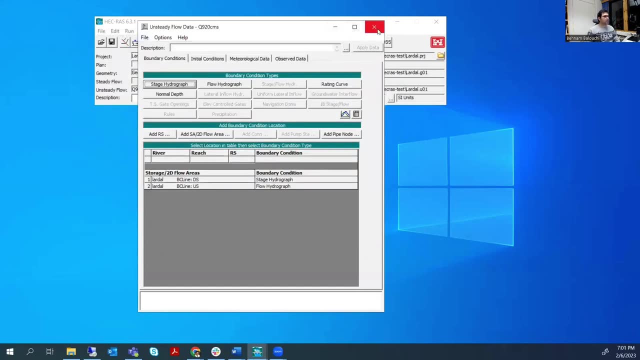 920 and then okay. So if you have an initial condition, you can add the initial conditions here. but we don't need it now And I will also explain for you how to make a hydraulic warmup, which is so important And especially when you don't have an initial condition. 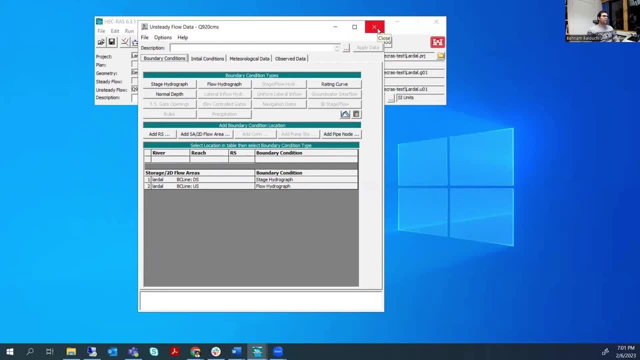 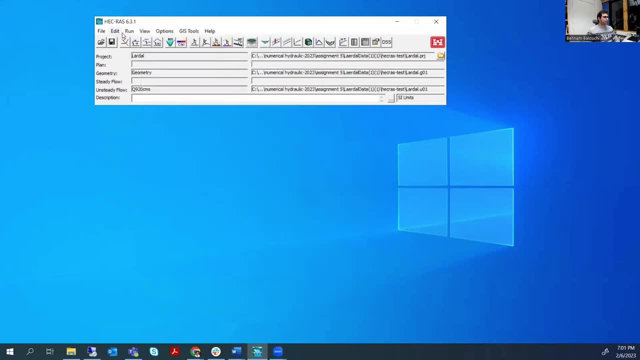 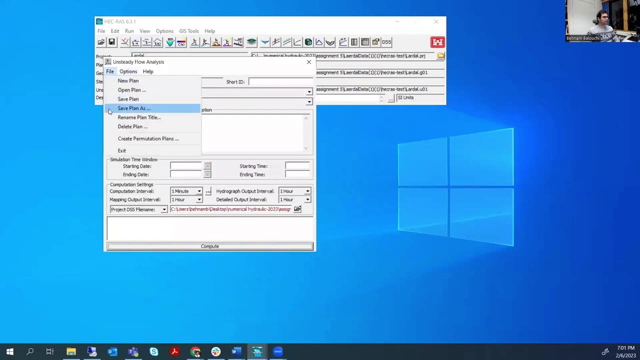 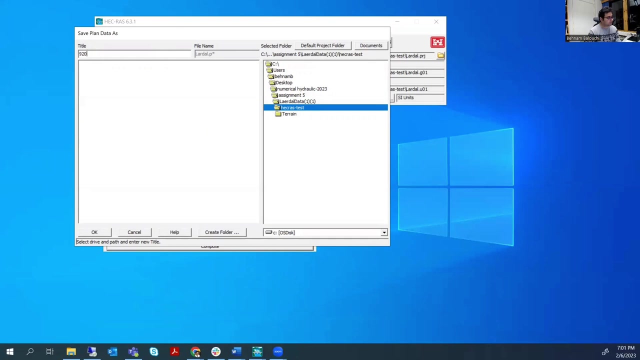 then it is really helpful and necessary And really really, really necessary. when you have a sediment in your model, Then we can go to the unsteady file savers, as we have the previous one. So it's 920, so Q. 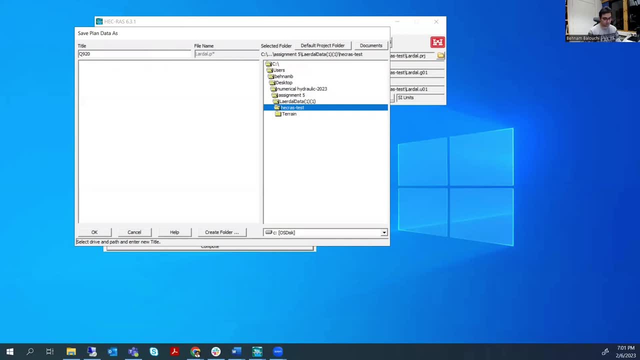 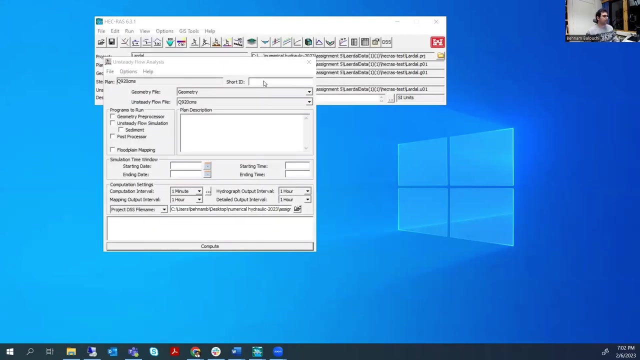 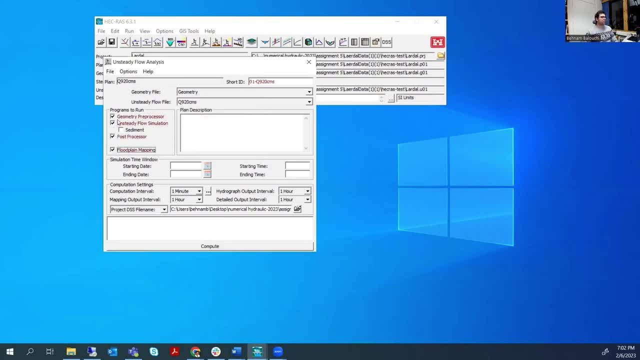 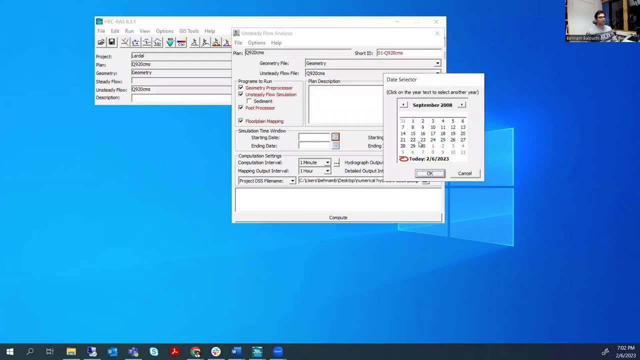 and then, as we don't have a sediment, we just take these things and it is really important to match the data, or the date that you have here, with the geometry, with the unsteady data that you have. so I choose it. today time is zero and then again, today time is six. we can go and check here on. 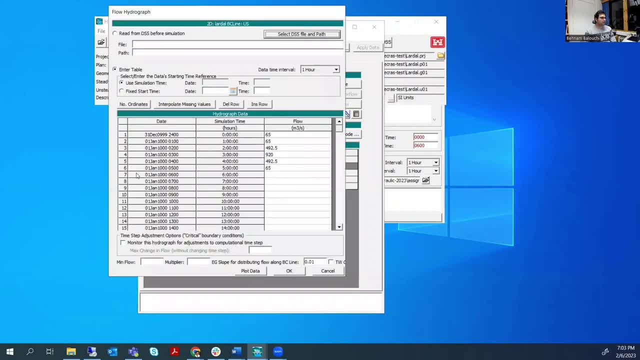 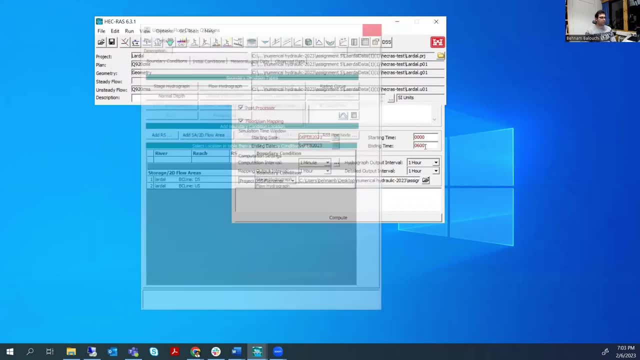 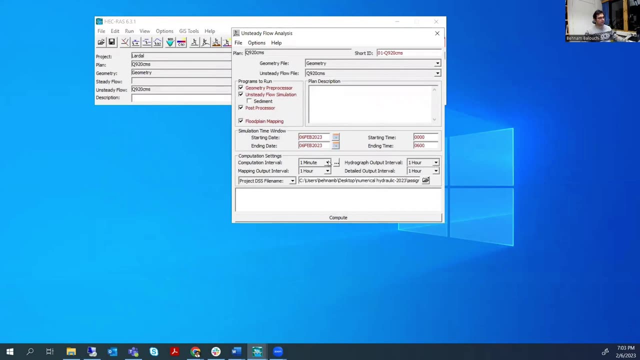 a steady fellow data, I took it off. we have, like the time of 5, 5 am, so just look what's happened. I can also change these things one second: five minutes. so this is the computational interval. Delta T. this is the mapping output interval: five minutes. 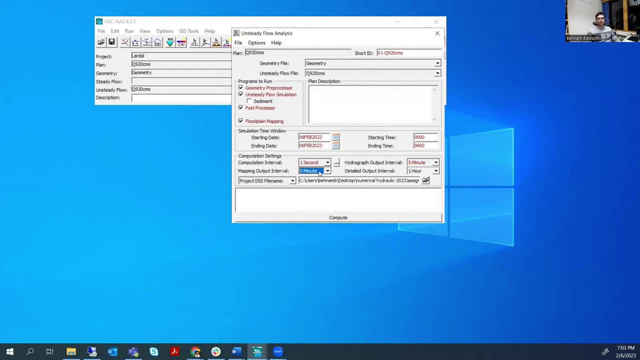 and its effect on the time, because it's overwrite or write the result. so if you make it less or make it higher its effect, the time of your modeling and hydrograph output interval we can use as the input, one that we introduce to the model as one hour, but we just keep it like that. 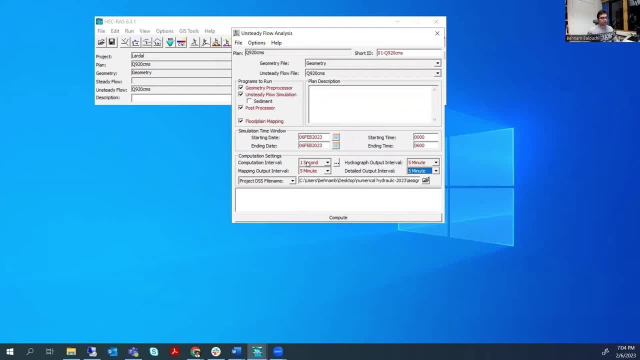 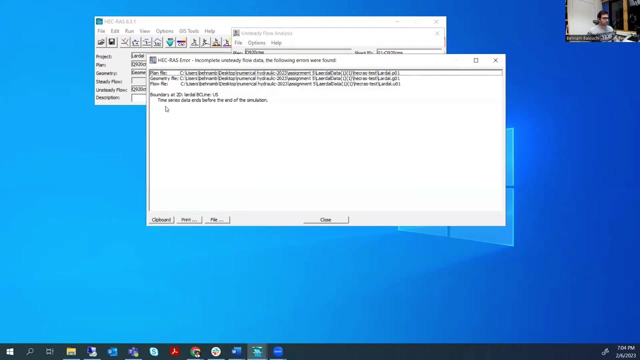 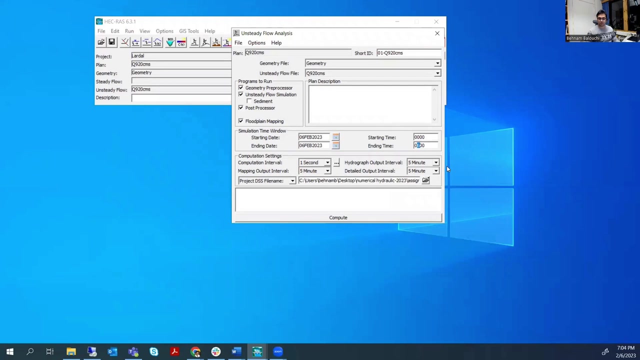 and the computational interval, which is so important for the stability of your model. we can keep it as one second and then we push the compute. so now you can see we got the error, as I told you, because the time of the simulation here it's not matched with the input data. so we should change it to five and then, if we run it, it's. 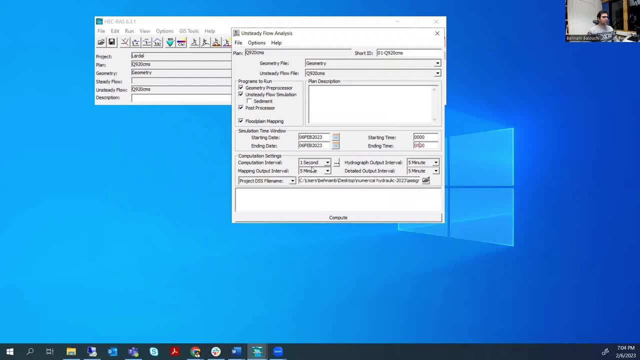 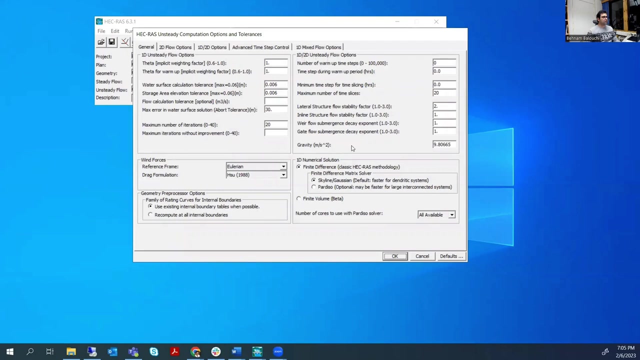 run, but i would like to explain you about some important options that we have in flow modeling. if you click here or if you are coming here- computational computation options- in options you can see this is for 1d- unsteady. this is for 1d- 2d- understeady. you can see the 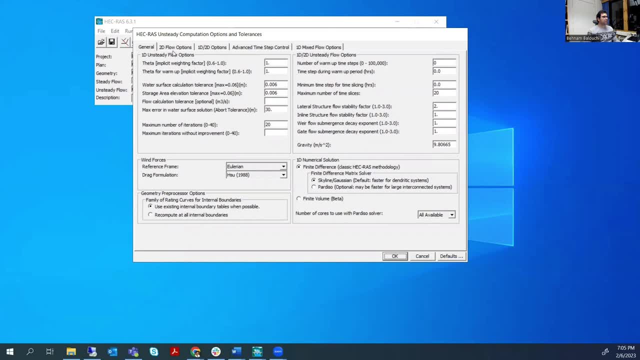 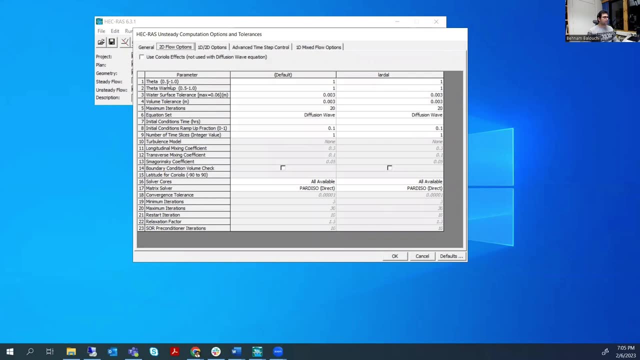 gravity and other parameters. we also have them here. i explain them here- which are more important. these are some values which we don't work with them usually, but you can go to the. i really recommend you to go to the hecress manual, or hecress reference, and read the manual. 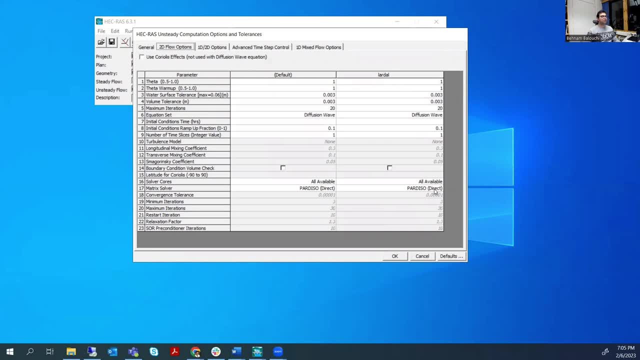 and then you will see what you need to do about the parameters, but some of them which are important, I explained to you. for example, you have values equation diffusion wave, which generally gives you more accurate results, but it is not recommended. if you have a sediment modeling, you should use most probably SWE ELM. it's also faster, but it depends. 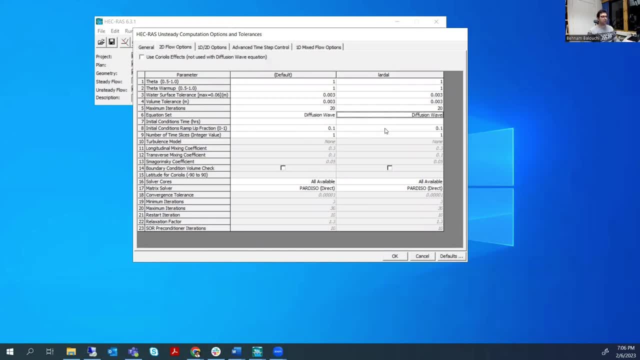 to your case and you should calibrate your model and see the data. but I give it as diffusion. the maximum iteration it's 20. it's the maximum number of iteration that you can have. if you decrease it you may have maybe faster modeling, but instead you'd also increase the instability and also some other. 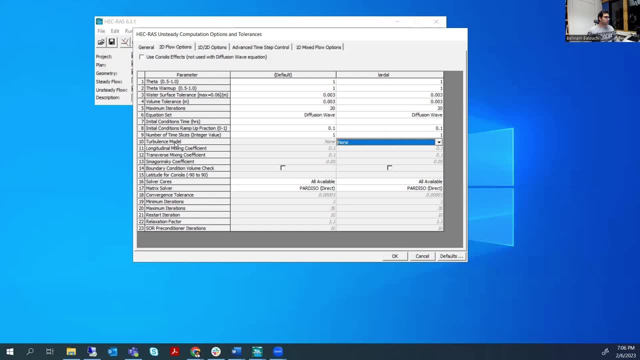 variables that you have here. so if you want the turbulence model, you can use the conservative or non-conservative in the reference. you have some recommendation. for example, if you use the SWE ELM equation, it is recommended to use the conservative form and there is for. 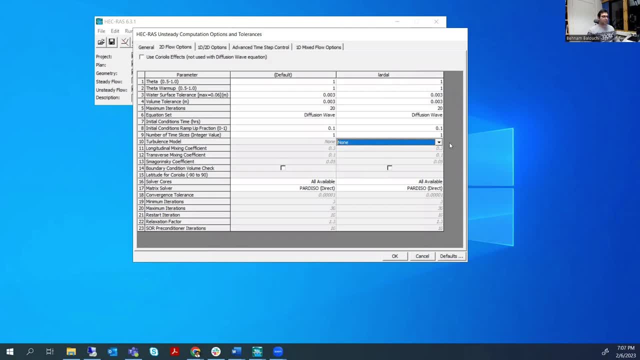 example a table in a HECRS manual that explains these things very well to you: an initial condition and initial condition ramp up fraction. i explain to you later. for example, you can put this one as 20 and this one as a 2. just keep this as a 10. 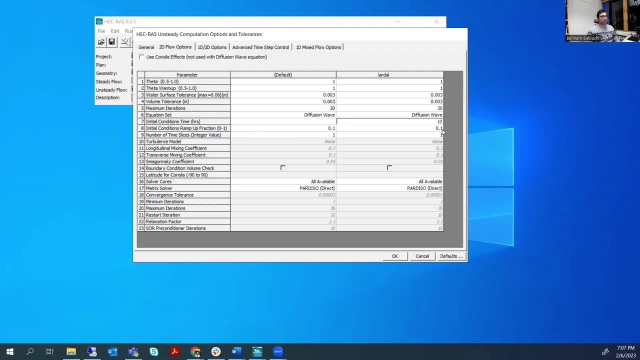 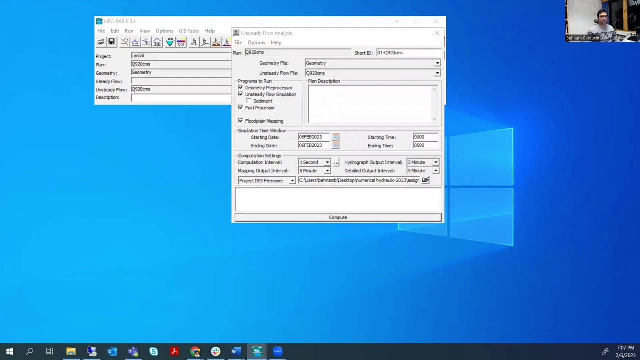 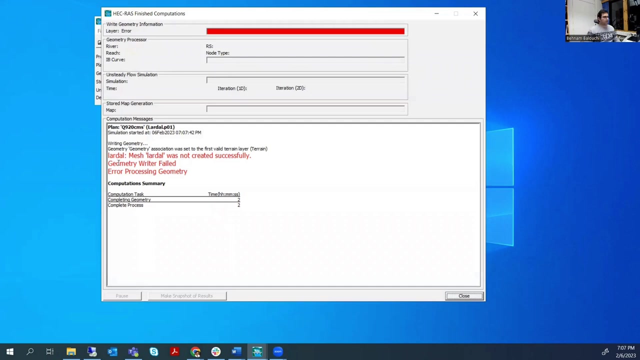 and this one is 0.1. it can be till 0.5. i explain you what is the definition of this. and then okay, and then compute. so we have a error here, an usual error. you can read it, it always errors. give you some information. 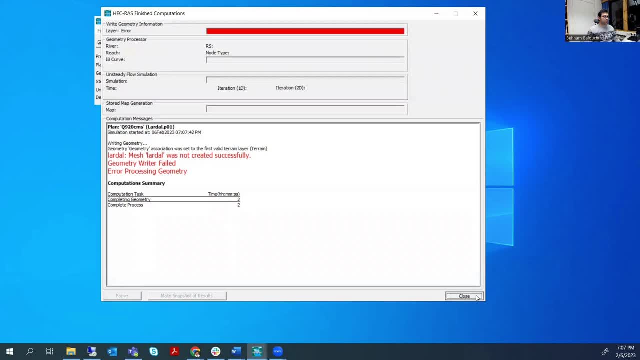 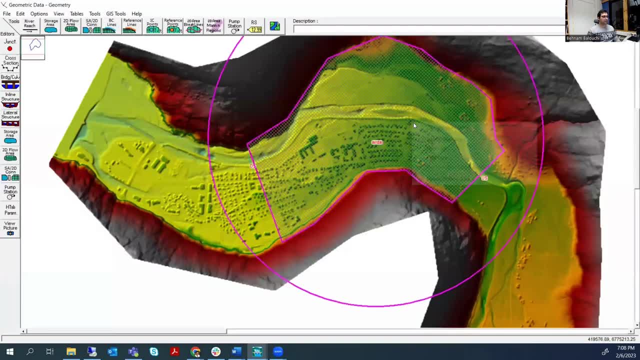 created successfully. it's a normal error. created successfully. it's a normal error if you close it and then go to the. if you close it and then go to the. if you close it and then go to the geometric data and then geometric data and then geometric data and then right click on the edit flow area. 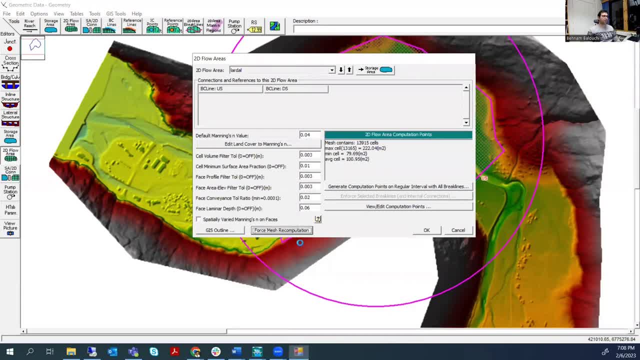 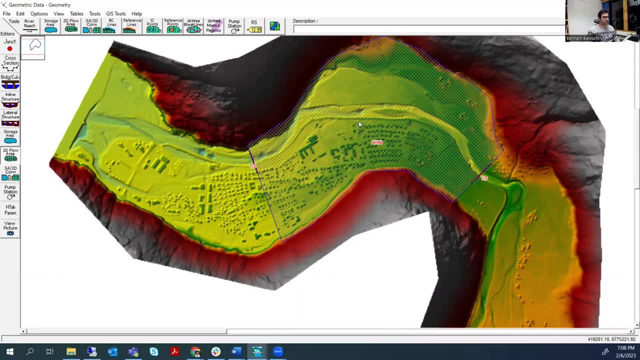 right click on the edit flow area. right click on the edit flow area and then force mesh recompression and then force mesh recompression, and then force mesh recompression. recomputation again, recomputation again, recomputation again. this is happens sometimes, sometimes, sometimes, and you have to recompute the mesh for 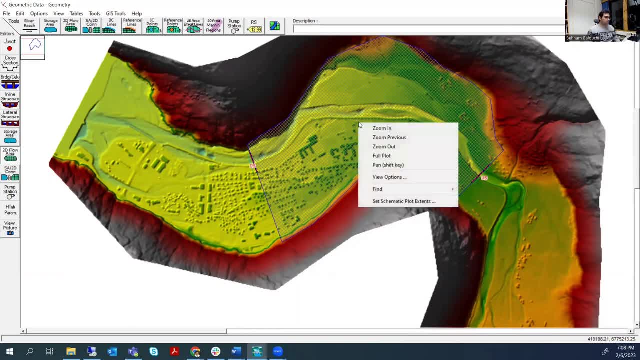 and you have to recompute the mesh for, and you have to recompute the mesh for running the across, running the across, running the across. you, if you right click on your mesh, you, you, if you right click on your mesh, you, you, if you right click on your mesh, you can go to the view. 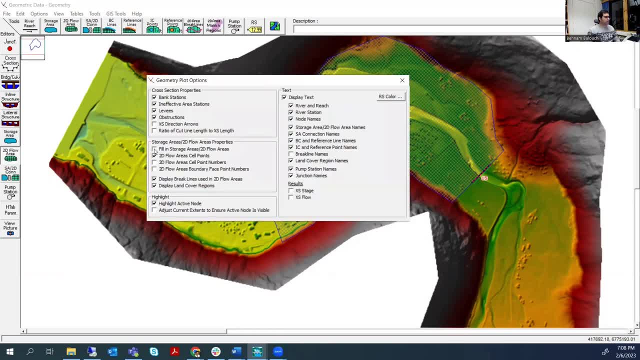 can go to the view can go to the view options. here you can see various options options. here you can see various options options. here you can see various options, for example, if you want to fill it, for example, if you want to fill it. for example, if you want to fill it, you can fill it. or other options that you 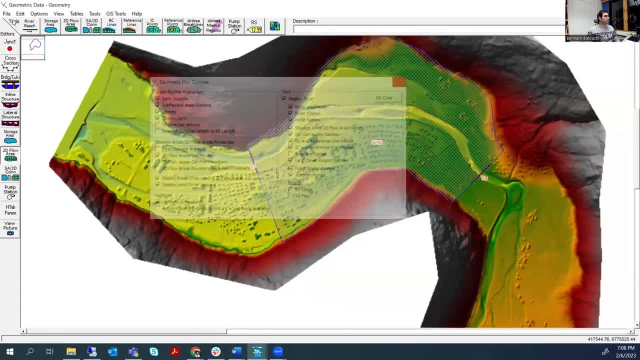 you can fill it, or other options that you you can fill it, or other options that you have to have to have to change the view of the geometric data, change the view of the geometric data, change the view of the geometric data, then i like to save it. 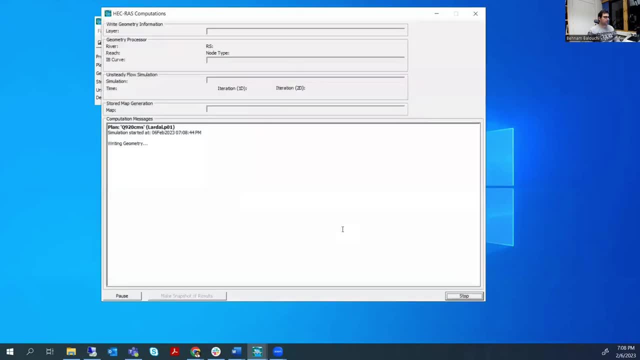 then i like to save it, then i like to save it, exit and here run and compute it, exit and here run and compute it, exit and here run and compute it. now i explain you what is the now. i explain you what is the now. i explain you what is the hydraulic warm-up, which is very, very. 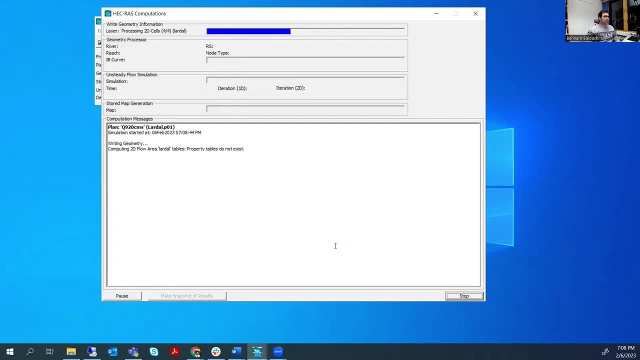 hydraulic warm-up, which is very, very hydraulic warm-up, which is very, very important in sediment modeling and also important in sediment modeling, and also important in sediment modeling, and also here, here, here, and i show you by, and i show you by a graph, and i show you by a graph. 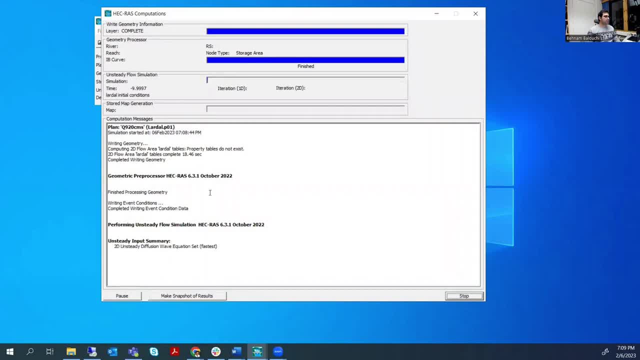 and i show you by a graph. here you can see the models information. here you can see the models information. here you can see the models information and the runs and the runs and the runs and the warm-up that we had and the warm-up that we had. 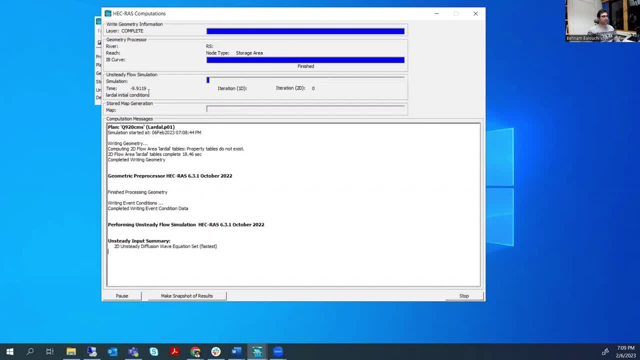 and the warm-up that we had. here it's i, if you remember. i add 10. here it's i, if you remember. i add 10. here it's i, if you remember. i add 10. now, from now, from now, from minus 10 to 0, we have a hydraulic. 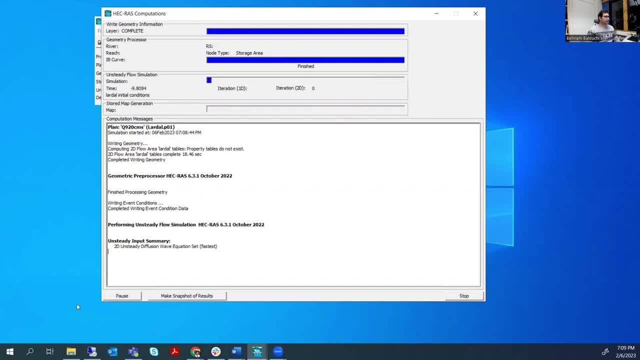 minus 10 to 0. we have a hydraulic minus 10 to 0. we have a hydraulic warm-up that you can see here. so let's go to the data we have. so let's go to the data we have. so let's go to the data we have. unsteady fellow data. 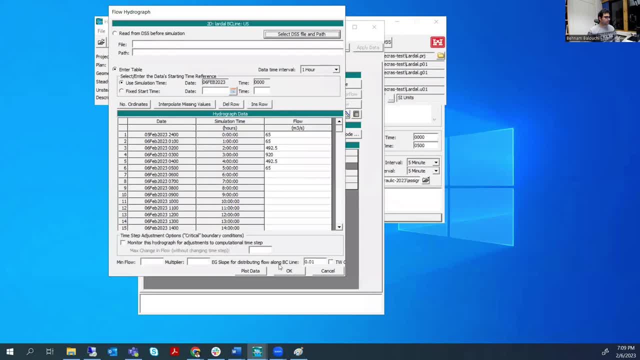 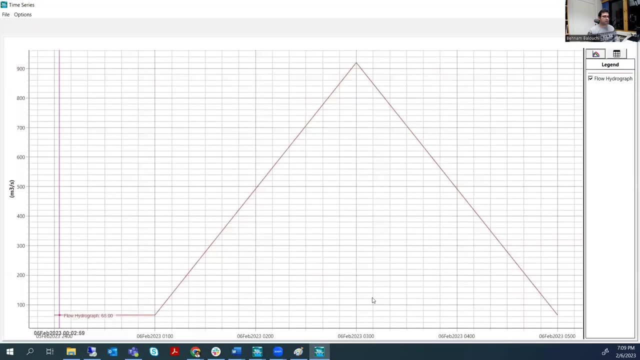 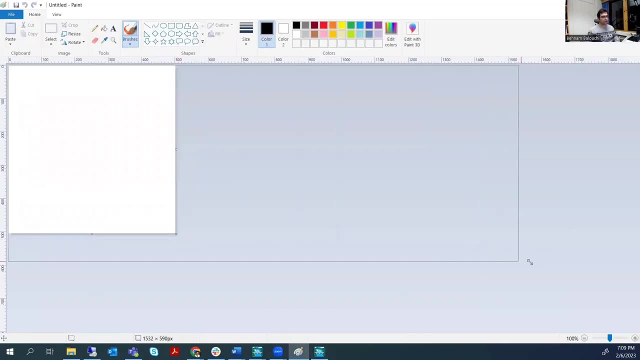 unsteady fellow data. unsteady fellow data. and below hydrograph and below hydrograph and below hydrograph. you can plot the data and here you can see, and here you can see, and here you can see the and here you can see the data. i like to draw this, so we just use a. 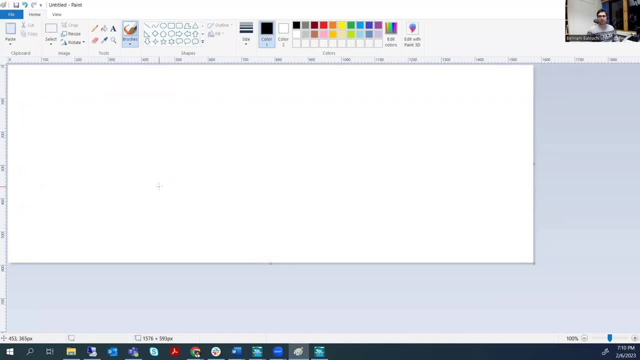 assumption for the unsteady hydrograph. assumption for the unsteady hydrograph, assumption for the unsteady hydrograph that we have so in the real scenario, you that we have so in the real scenario, you that we have so in the real scenario, you use a real hydrograph. 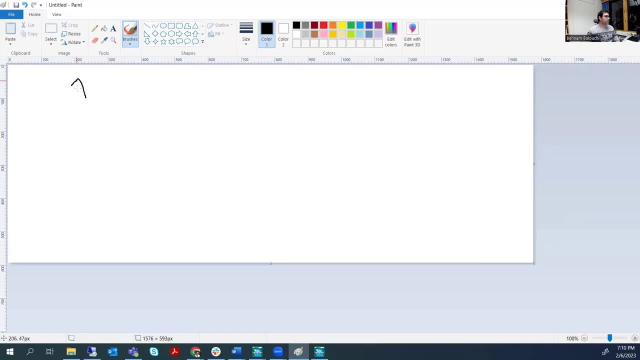 use a real hydrograph, use a real hydrograph, but again in the hydrograph, for example, but again in the hydrograph, for example, but again in the hydrograph, for example. i just try to, i just try to, i just try to show you the hydrograph that we have. 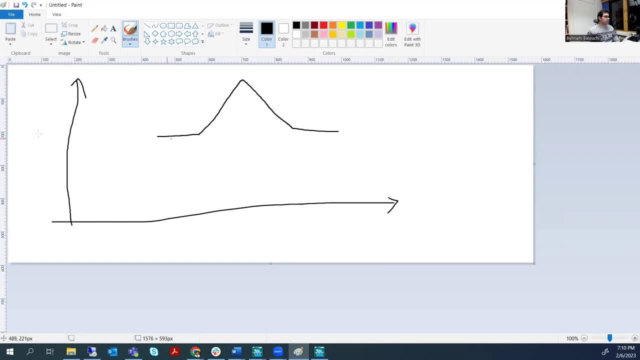 show you the hydrograph that we have. show you the hydrograph that we have, the hydrograph that we use. it's like this: the hydrograph that we use. it's like this: the hydrograph that we use. it's like this: here it's 65 and here it's. 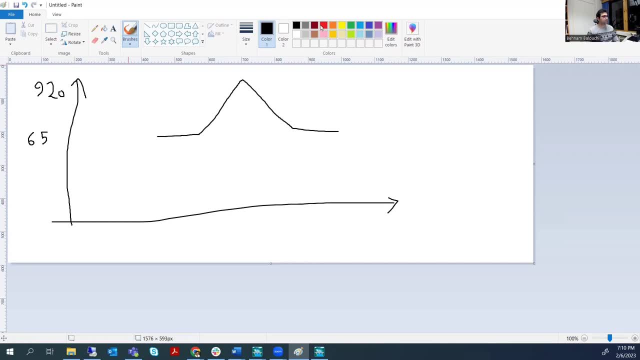 65, and here it's 65 and here it's 920.. so the 10 values that we use, so the 10 values that we use, so the 10 values that we use- is a hydraulic warm-up and it's is a hydraulic warm-up and it's. 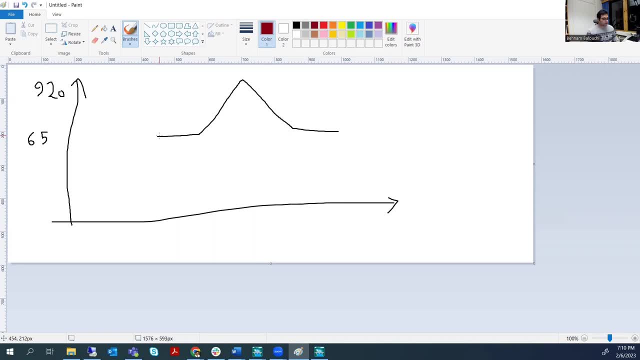 is a hydraulic warm-up and it's so usually from if we want to avoid so, usually from if we want to avoid so, usually from if we want to avoid the shock to the shock, to the shock to our model, our model, our model, so we, it is better not to start modeling. 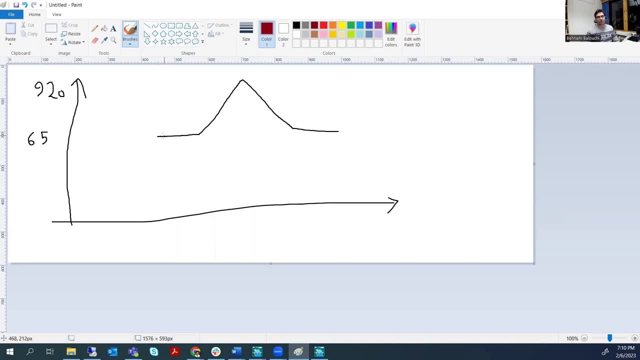 so we, it is better not to start modeling. so we, it is better not to start modeling from, from from this high value of discharge, so it is better, this high value of discharge, so it is better. this high value of discharge, so it is better to start from, like discharge of zero. 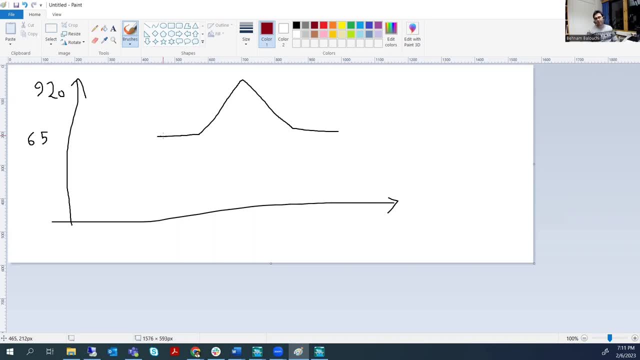 to start from like discharge of zero. to start from like discharge of zero and gradually we increase it till, and gradually we increase it till, and gradually we increase it till: 6, 6, 6, 65 discharge, 65 discharge, 65 discharge, so, so, so some researchers or some modelers use a 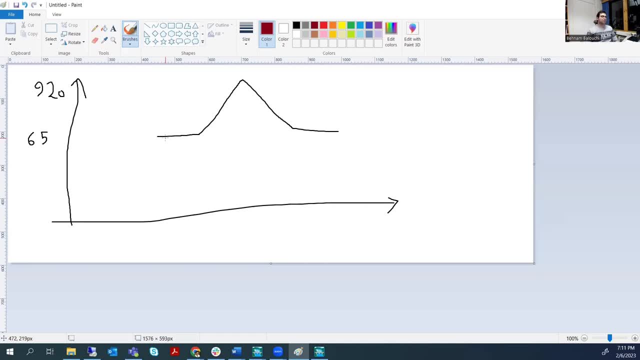 some researchers or some modelers use a. some researchers or some modelers use a synthetic, synthetic, synthetic hydraulic discharge at some values before hydraulic discharge, at some values before hydraulic discharge, at some values before that, that that. but i really recommend to use this, but i really recommend to use this. 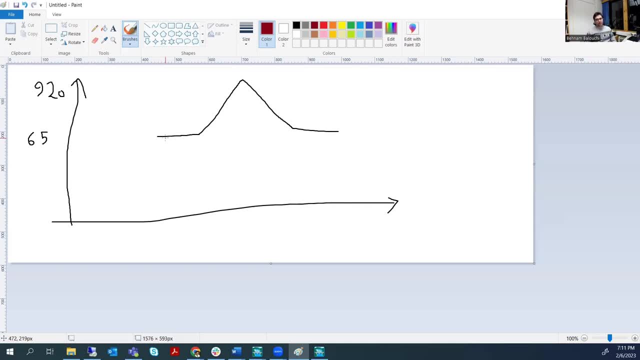 but i really recommend to use this interesting option of hecress, especially interesting option of hecress, especially interesting option of hecress, especially for the sediment modeling. it's really for the sediment modeling. it's really for the sediment modeling. it's really important to use it. so the first value: 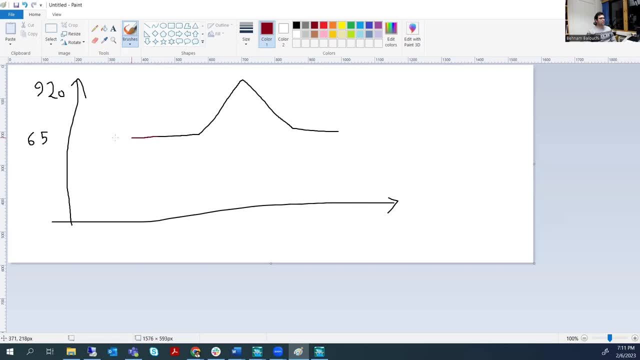 important to use it. so the first value: important to use it. so the first value: that we use 10, it's just to increase, that we use 10, it's just to increase. that we use 10, it's just to increase 10, 10 hours of. 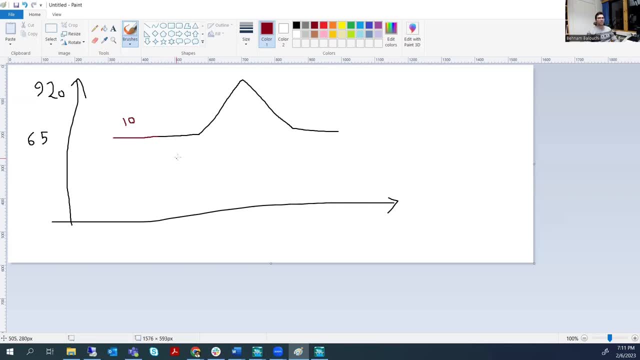 10 hours of 10 hours of modeling, which i modeling, which i modeling, which i add a lot, because our modeling is just add a lot, because our modeling is just add a lot, because our modeling is just five hours, and i add five hours and i add. 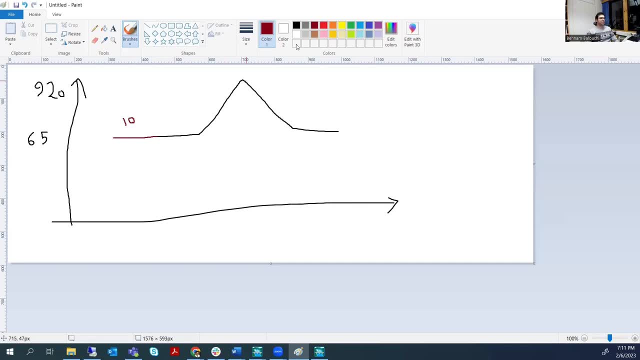 five hours and i add a lot, a lot, a lot. and what is the ramp? the ramp is the and what is the ramp? the ramp is the and what is the ramp? the ramp is the one point, one point, one point, uh, uh, uh. point one is the. 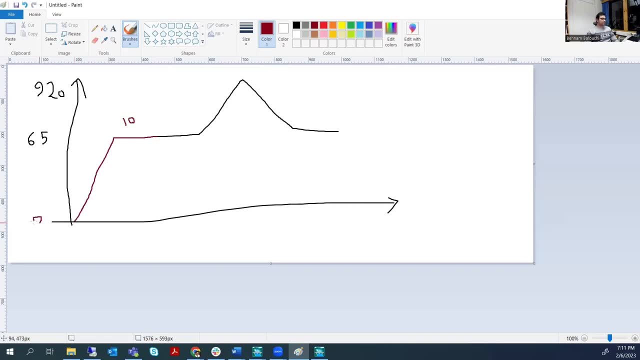 point one is. the point one is the slope of these till slope of these till slope of these till discharge of zero, discharge of zero, discharge of zero. the maximum of the maximum, of the maximum of ramp value is the ramp value is the ramp value is the 0.5. 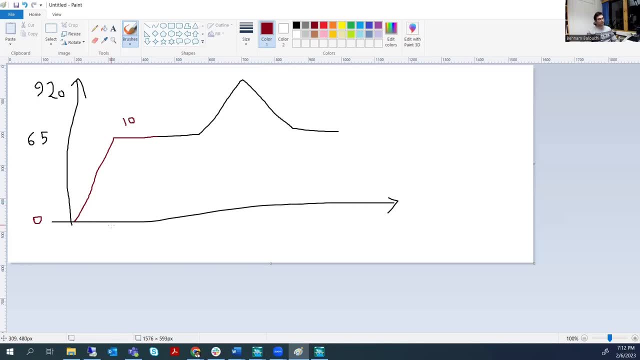 0.5, 0.5, which is like a 45, which is like a 45, which is like a 45: uh degree, uh degree, uh degree. the angle of this, i think it's it will be. the angle of this, i think it's it will be. 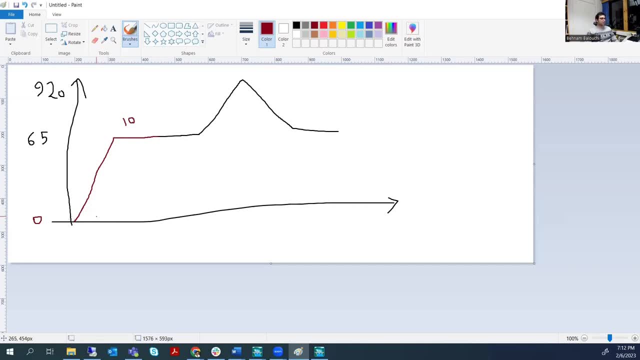 the angle of this, i think it's. it will be 45 and it's the maximum 45 and it's the maximum 45 and it's the maximum one if you want to have a one, if you want to have a one, if you want to have a like. 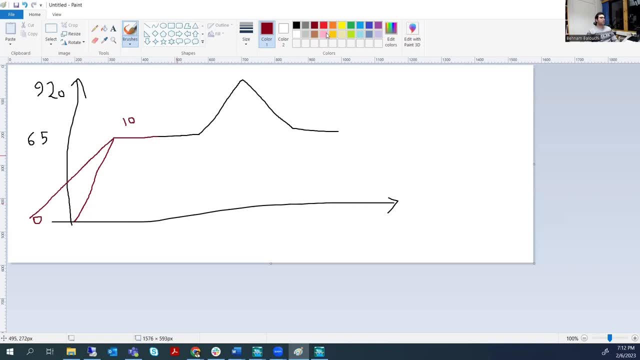 like like mild slope or high slope- mild slope or high slope, mild slope or high slope- so i really recommend to use this. so i really recommend to use this. so i really recommend to use this. so this is discharge, so this is discharge, so this is discharge and this is time. 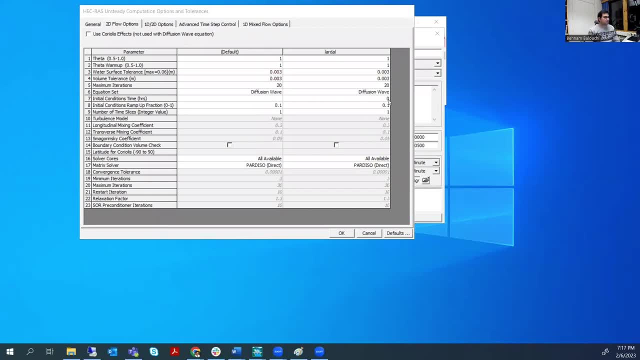 so this is the value that i told you. i. so this is the value that i told you, i. so this is the value that i told you. i change it to zero. because change it to zero, because change it to zero, because i want to be so fast. 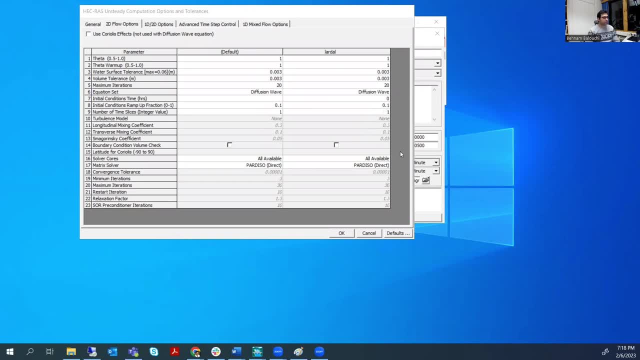 i want to be so fast, i want to be so fast, and we keep it this one as, and we keep it this one as, and we keep it this one as a point one, a point one, a point one. and if you have so many uh, and if you have so many uh, 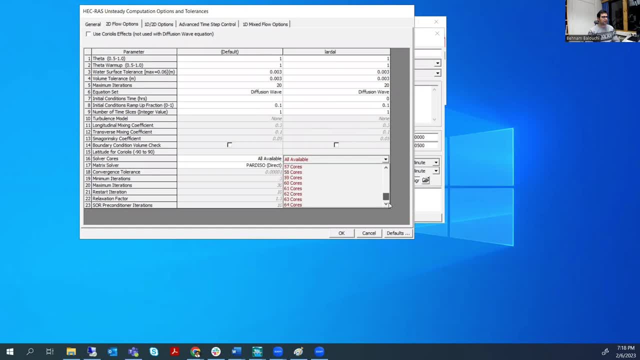 and if you have so many uh runs with so many cores, you can also runs with so many cores. you can also runs with so many cores. you can also decrease, decrease, decrease these cores, these cores, these cores, because, for, because, for, because, for a crash, it is a crash, it is. 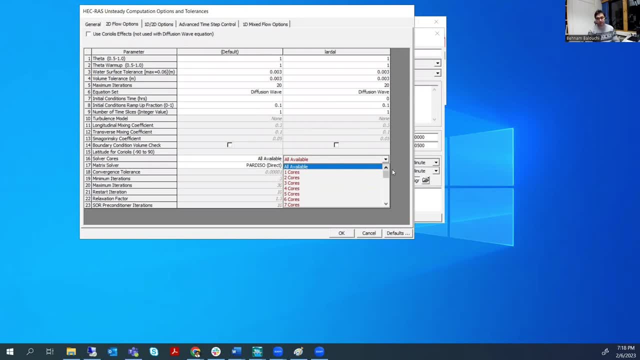 a crash. it is really important to have a course with really important to have a course with really important to have a course with high speed, high speed, high speed instead of- instead of- instead of having so many cores like having so many cores, like having so many cores like 60 cores with low speed. 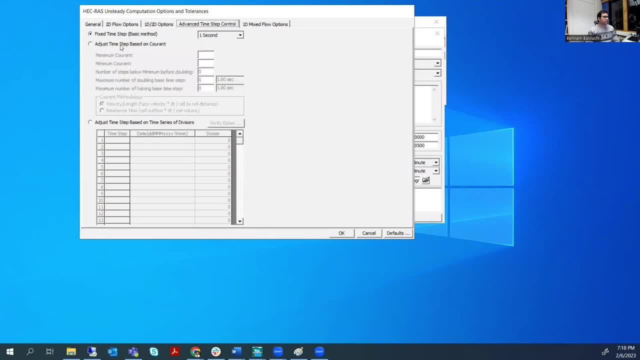 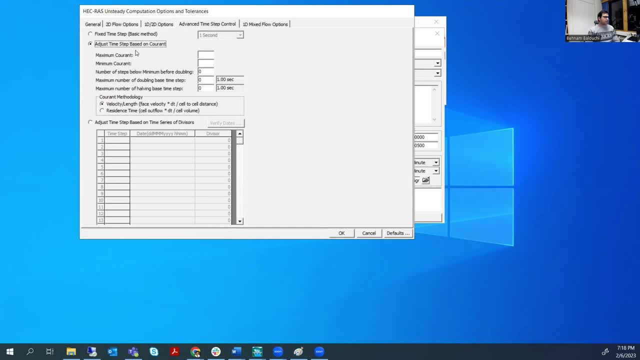 instead of fixed time step, you can change it to the adjust time step. change it to the adjust time step. change it to the adjust time step. delta t, delta t. delta t in the heckress is a. in the heckress is a. in the heckress is a model parameters, so you can change it. 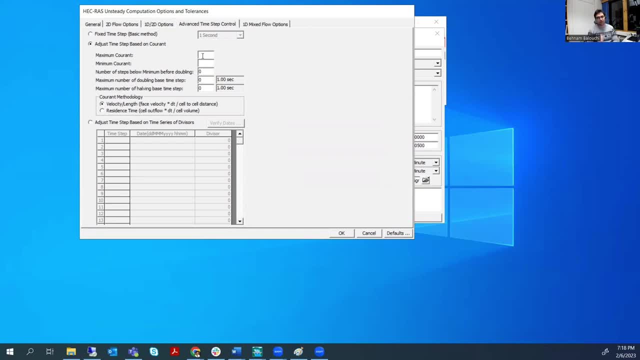 model parameters, so you can change it. model parameters, so you can change it, but it's not necessary to have it like, but it's not necessary to have it like, but it's not necessary to have it like one or to have it like 1.2. 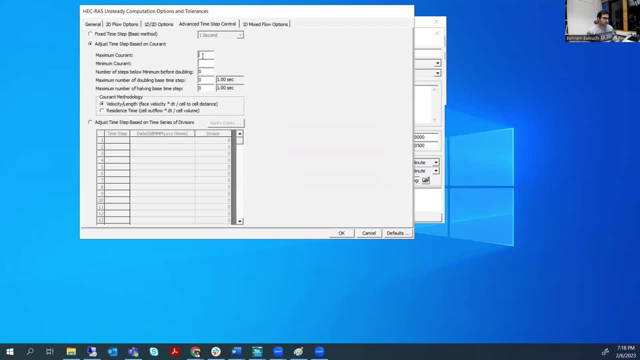 one, or to have it like 1.2 one, or to have it like 1.2 it's converged: the results to a it's converged. the results to a it's converged the results to a stable stable. stable. stable results. stable results, stable results. so you can. 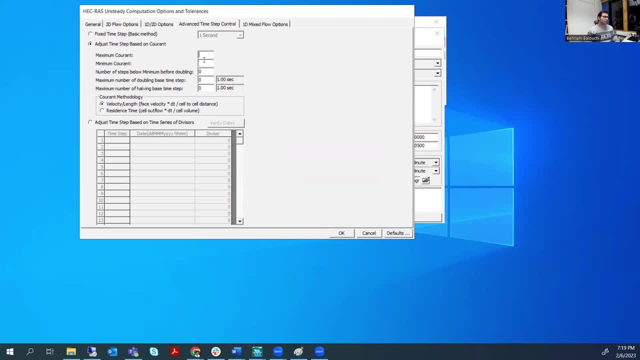 so you can. so you can use like one here, use like one here, use like one here, but you can also use two. but you can also use two, but you can also use two, and then the minimum, and then the minimum, and then the minimum current should be more than. 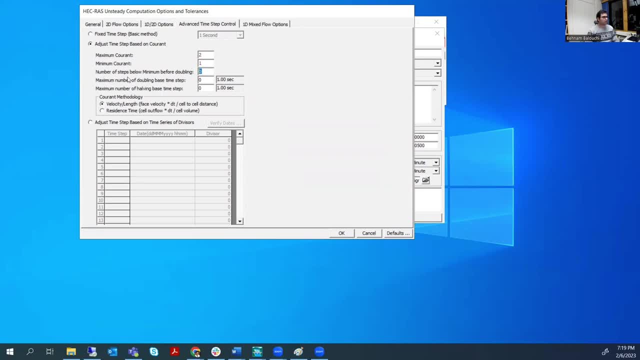 current should be more than current, should be more than half of the two, half of the two, half of the two, and then you have a number of steps below, and then you have a number of steps below, and then you have a number of steps below minimum, for example. you can change it. 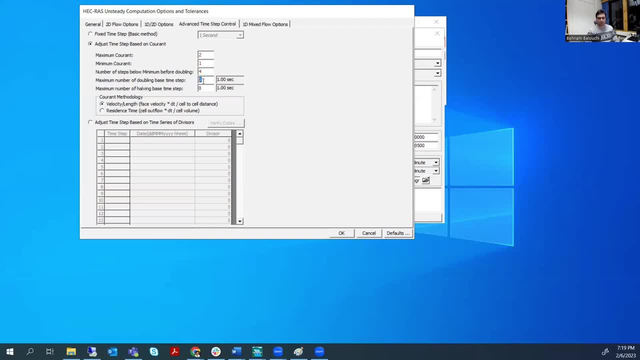 minimum, for example, you can change it. minimum, for example, you can change it to four to four to four, and maximum number of doubling you can and maximum number of doubling you can and maximum number of doubling you can change it, change it, change it to four. i also use this one to four here. 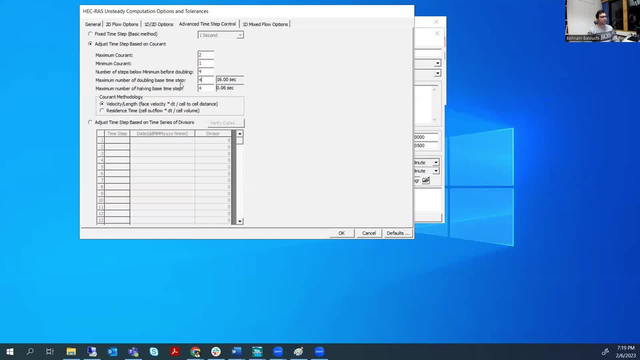 to four. i also use this one to four here to four. i also use this one to four here you can see the maximum number of. you can see the maximum number of. you can see the maximum number of time step that time. step that time, step that hecras or your model will use is 16. 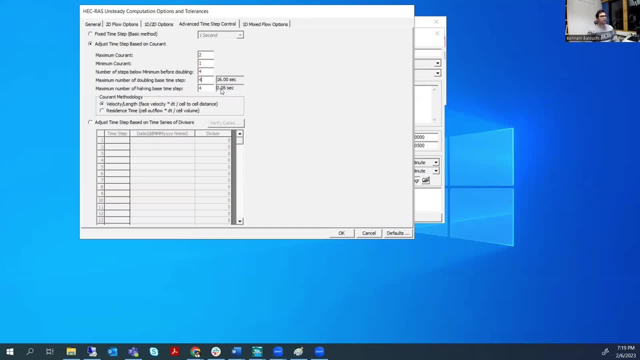 hecras, or your model will use is 16 hecras, or your model will use is 16 seconds, seconds, seconds, and then the minimum is, and then the minimum is, and then the minimum is 0.06. so if your results are not stable, 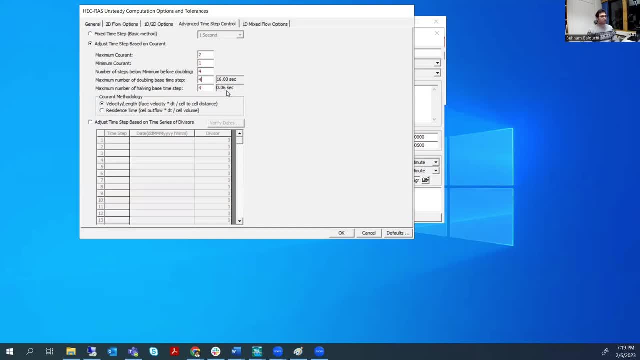 0.06. so if your results are not stable, 0.06. so if your results are not stable, then then then the model decrease the delta t to this, the model decrease the delta t to this, the model decrease the delta t to this value, and if it is stable, so for: 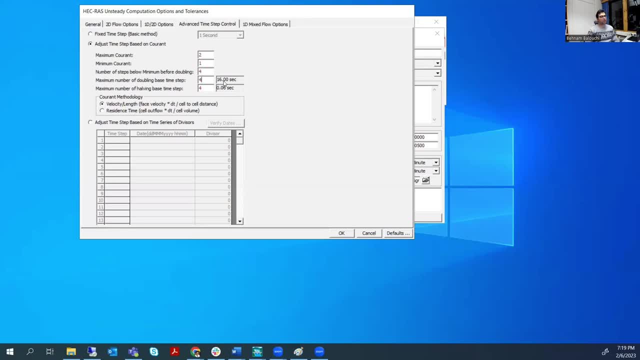 value. and if it is stable, so for value, and if it is stable, so for having a faster result. it may choose the having a faster result, it may choose the having a faster result. it may choose the bigger one, the bigger one, the bigger one, the 16, or between these values. 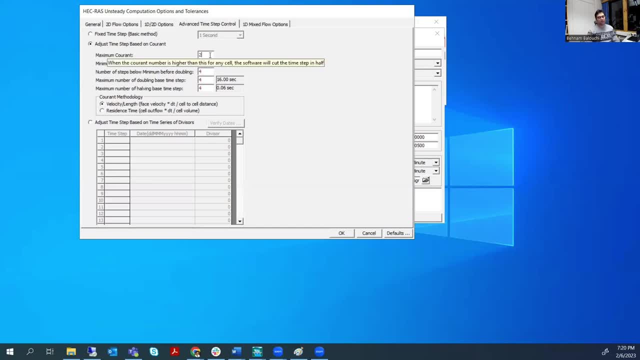 16 or between these values. 16 or between these values. i think two is, i think two is. i think two is a good value. a good value. a good value, but you can also use one. it depends on. but you can also use one. it depends on. 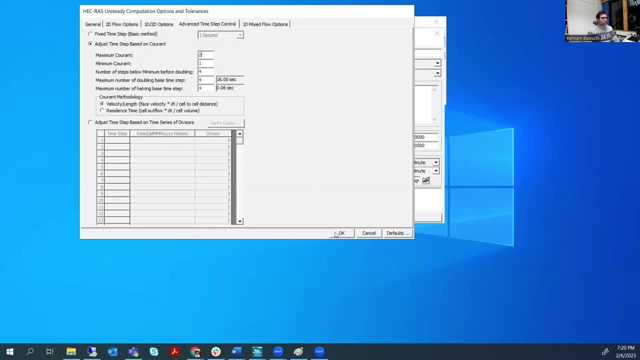 but you can also use one. it depends on your, your, your modeling or result, but both of them modeling or result. but both of them modeling or result. but both of them should be good according to my, should be good according to my, should be good according to my experience. 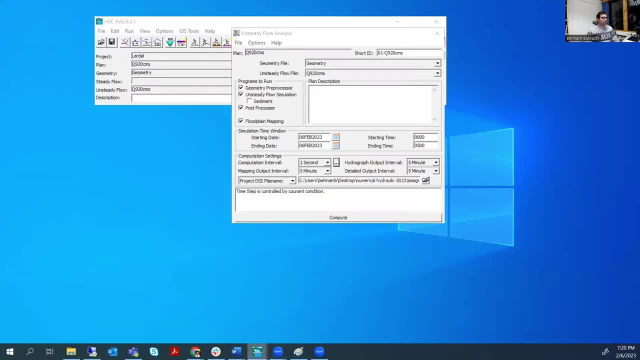 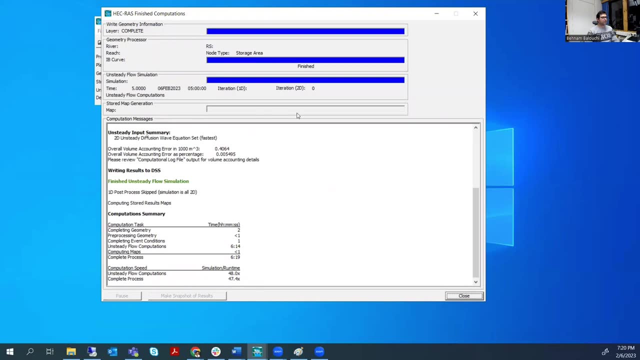 experience. then you can have a result here. you can see the results that you have here. you see the results that you have here. you see the results that you have here. you see the number of your plan and some the number of your plan and some the number of your plan and some information here. 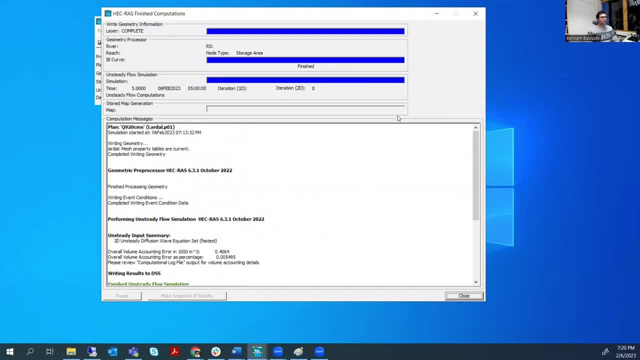 information here. information here, so we don't have any error here. but if so, we don't have any error here. but if so, we don't have any error here. but if you run it, you can see the number of. you run it, you can see the number of. 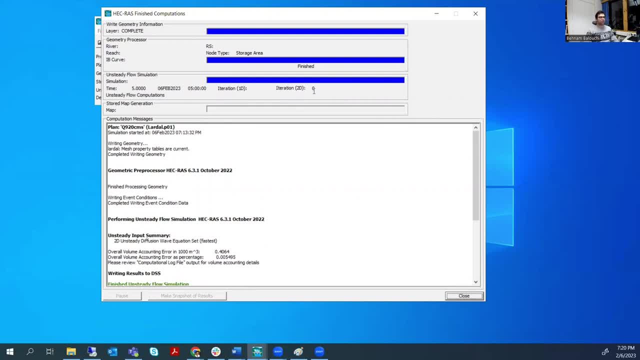 you run it, you can see the number of iteration. here it's 2, 3 or it's reach 20. iteration: here it's 2, 3 or it's reach 20. iteration: here it's 2, 3 or it's reach 20. and if 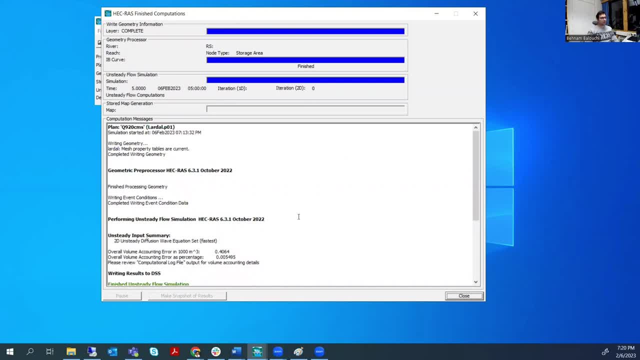 and if and if it, and if it reach 20, then you have the sales number reach 20, then you have the sales number reach 20, then you have the sales number of the errors that you have here and you of the errors that you have here and you. 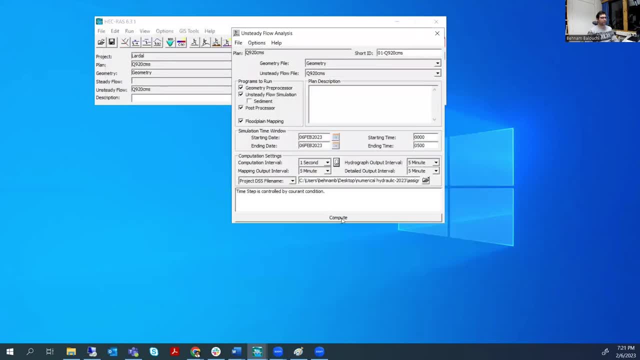 of the errors that you have here and you can find the sales number. can find the sales number, can find the sales number. so as i change the delta t here, i just run it to show you delta t here. i just run it to show you delta t here. i just run it to show you it is. 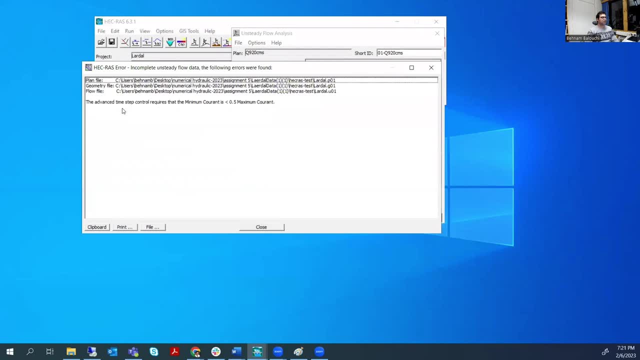 it is, it is correct. you can see here, you will receive correct. you can see here, you will receive correct. you can see here, you will receive the error: the advanced time step. the error, the advanced time step, the error, the advanced time step. control requires that the minimum 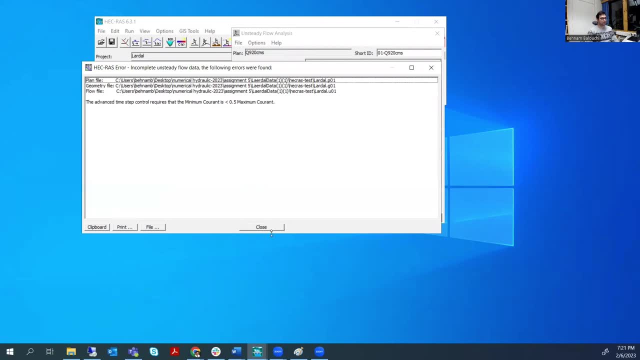 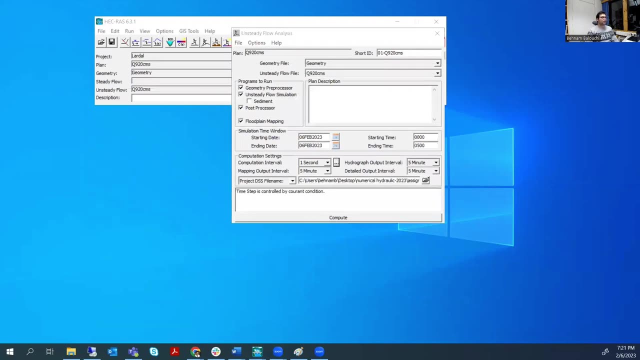 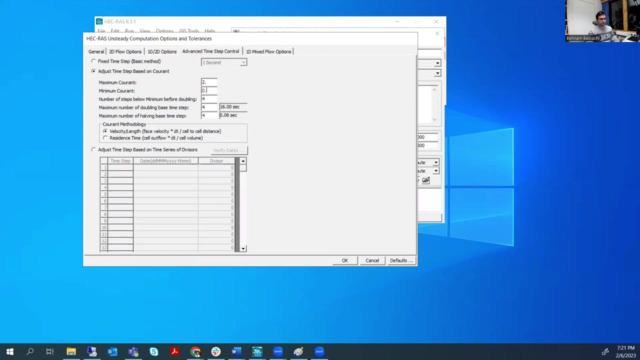 control requires that the minimum control requires that the minimum current is less than half of the current is less than half of the current is less than half of the maximum. so i, i, i, i change it to this value, and then i change it to this value, and then 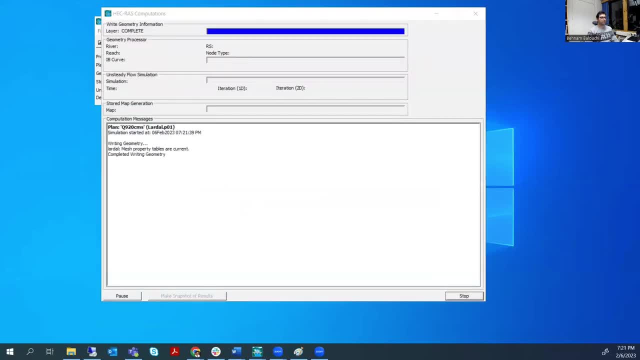 i change it to this value and then you can see it's, you can see it's, you can see it's wrong, wrong, wrong. but i stop it because, but i stop it because, but i stop it because with the previous one it's. with the previous one it's. 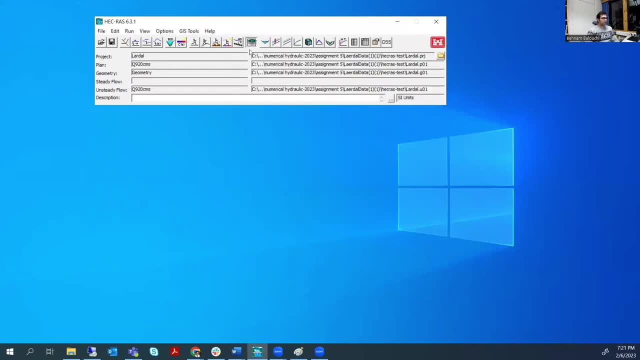 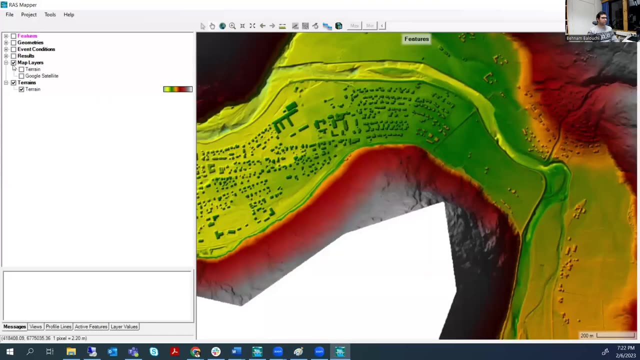 with the previous one. it's done, done, done. okay, now we are going to the last mapper. okay, now we are going to the last mapper. okay, now we are going to the last mapper to see the results. you can go to the results and for. you can go to the results and for. 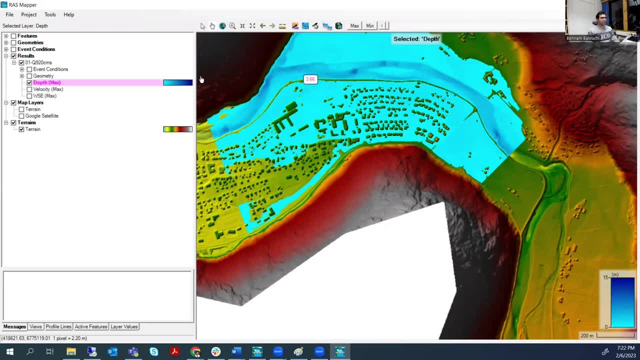 you can go to the results and, for example, show the example. show the example. show the depth. if you play the depth, you can see. if you play the depth, you can see. if you play the depth, you can see it's changed, it's changed, it's changed. so if you want to change it, for example, 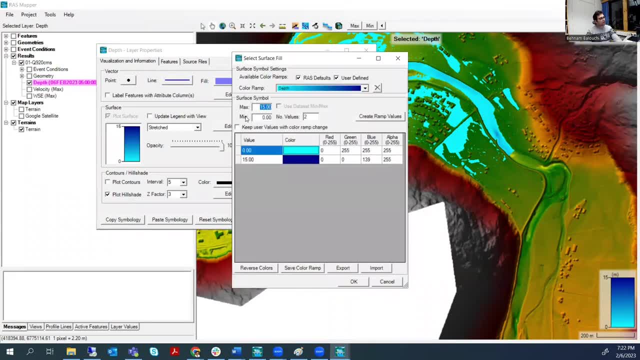 so if you want to change it for example, so if you want to change it for example, go to go to go to double click on the color pattern, then double click on the color pattern, then double click on the color pattern, then here change it to two. you can here have a. 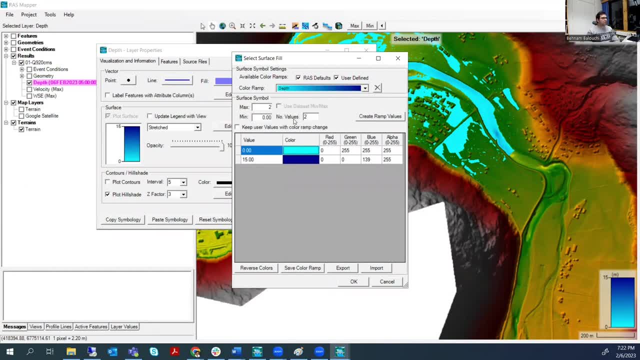 here, change it to two. you can here have a. here, change it to two. you can here have a different color, but the depth is this, or different color, but the depth is this, or different color, but the depth is this. or you can also increase the. you can also increase the. 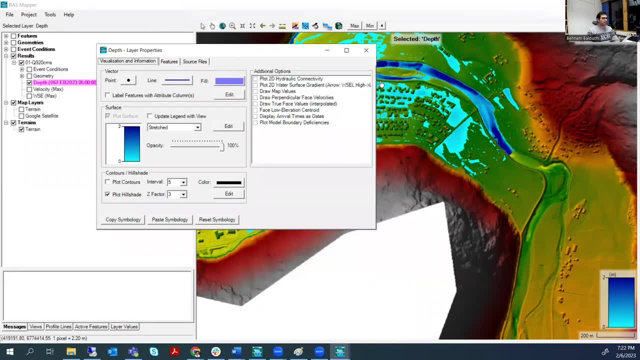 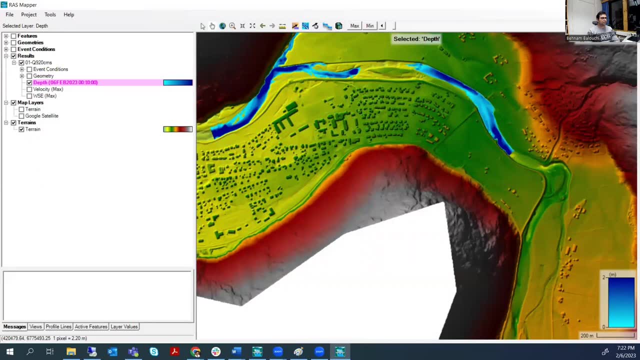 you can also increase the glasses, then create ramp value, and then glasses, then create ramp value, and then glasses, then create ramp value, and then, okay, now you can see the results again. okay, or, if you want to see the vectors, you. or if you want to see the vectors you. 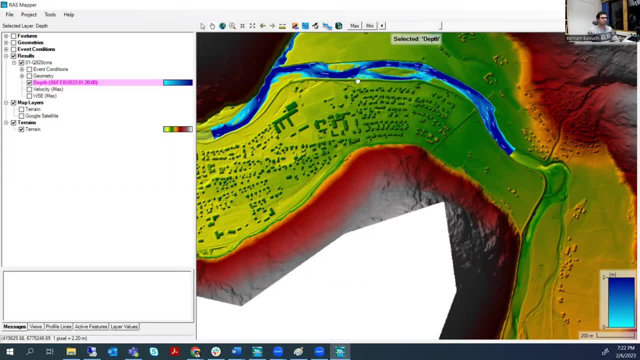 or if you want to see the vectors, you can use this one can use this one, can use this one. or if you want to see the, or if you want to see the, or if you want to see the animated vectors, you can add this one. animated vectors, you can add this one. 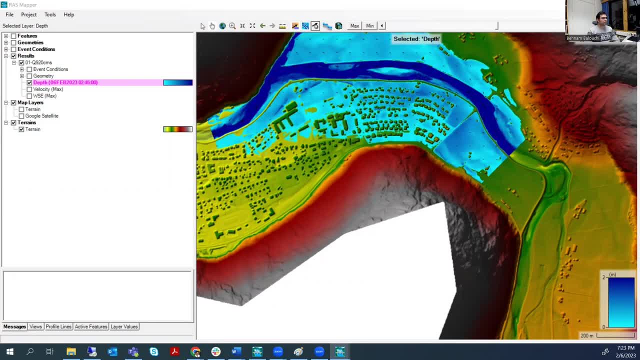 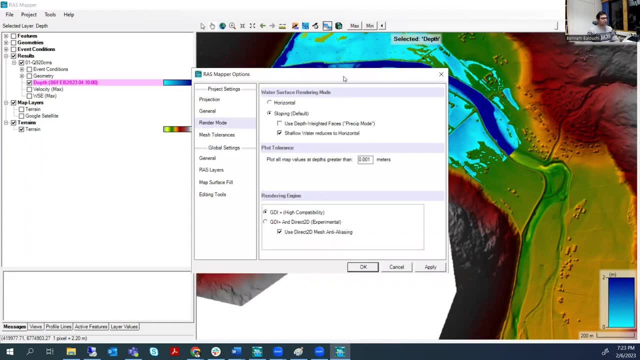 animated vectors. you can add this one. this is also some options that you have. this is also some options that you have. this is also some options that you have for the vectors, for the vectors, for the vectors, or here you have some other parameters. this one is: you have some other parameters? this one is: 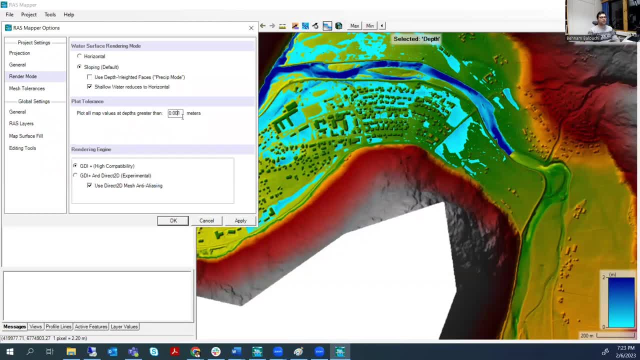 you have some other parameters. this one is useful, for example: useful, for example. useful, for example, use, useful, for example, use set. okay, our accuracy is not like one set. okay, our accuracy is not like one set. okay, our accuracy is not like one millimeters. i want to increase it to one. 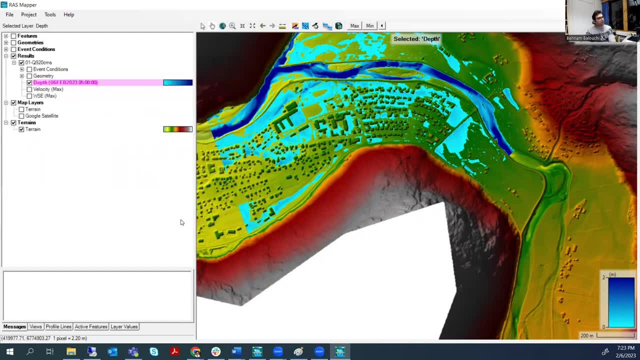 millimeters. i want to increase it to one millimeters. i want to increase it to one centimeter, then you centimeter, then you centimeter, then you delete this one, and okay, and you delete this one, and okay, and you delete this one, and okay, and you delete the water depth below. 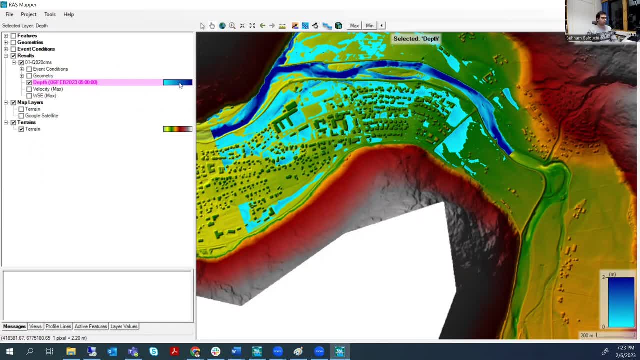 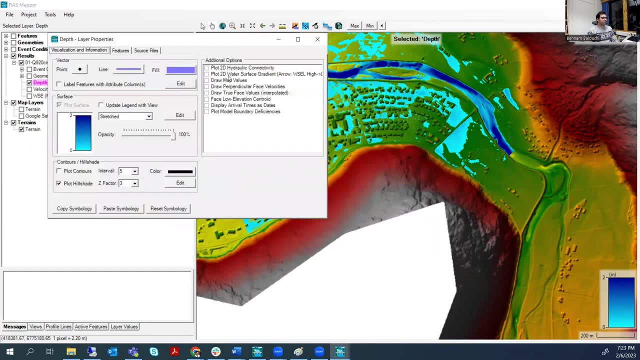 delete the water depth below, delete the water depth below that. that value like that, that value like that, that value like one centimeters, one centimeters, one centimeters. another important thing that you should, another important thing that you should, another important thing that you should learn how to work with this. what is? 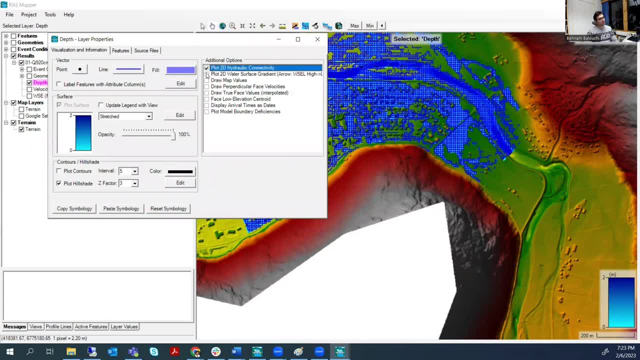 learn how to work with this? what is learn how to work with this? what is these, these, these options, for example plot, if you options for example plot, if you options for example plot, if you take this one, take this one, take this one, you can see the, you can see the. 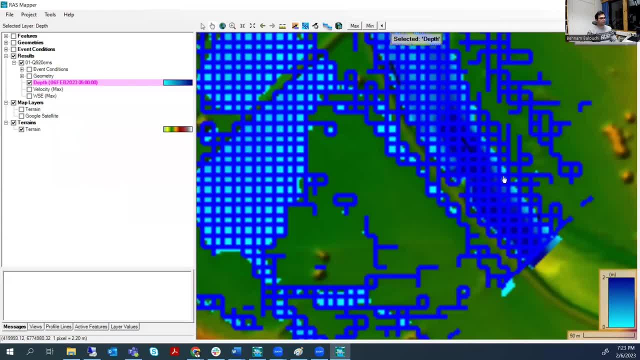 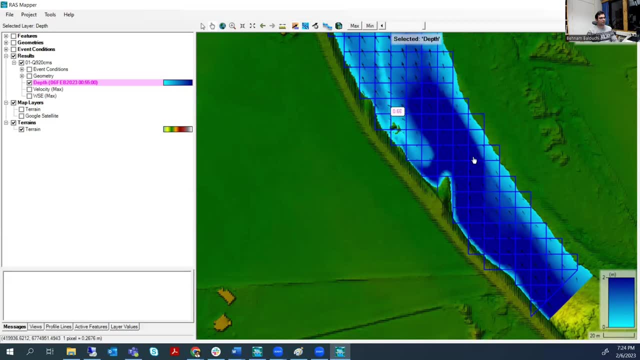 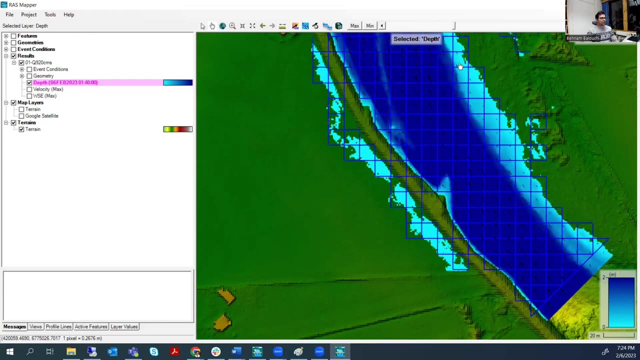 you can see the flow connectivity of them. so we want to evaluate this, the fellow. so we want to evaluate this, the fellow. so we want to evaluate this, the fellow and the vectors. you can see them. everything is, everything is everything is seems correct till here. seems correct till here. 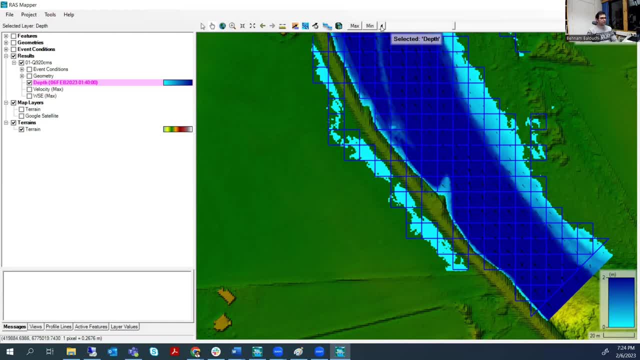 seems correct till here. so we have a wall here, so we have a wall here, so we have a wall here, but the water goes to the other sides, but the water goes to the other sides, but the water goes to the other sides, exactly at, exactly at, exactly at this. 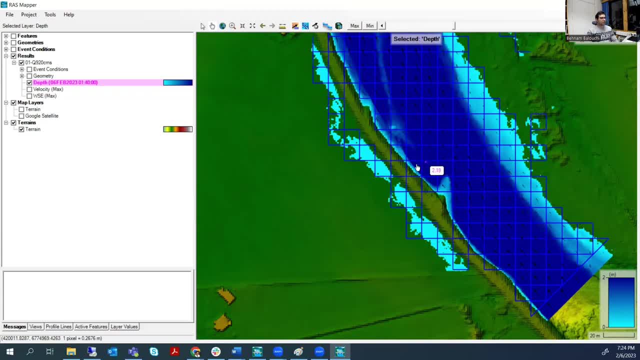 exactly at this time, this time, this time. so what's happened as the? so what's happened as the? so what's happened as the our mesh is large, then we have some. our mesh is large, then we have some our mesh is large, then we have some cells like this one: 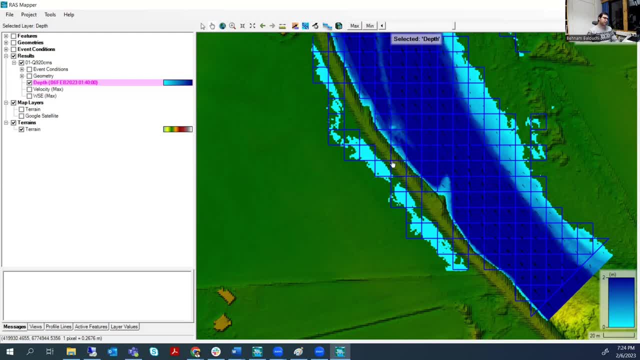 cells like this one, cells like this one: half of them is in the water and half of half of them is in the water. and half of half of them is in the water and half of them is in the on the wall. them is in the on the wall. 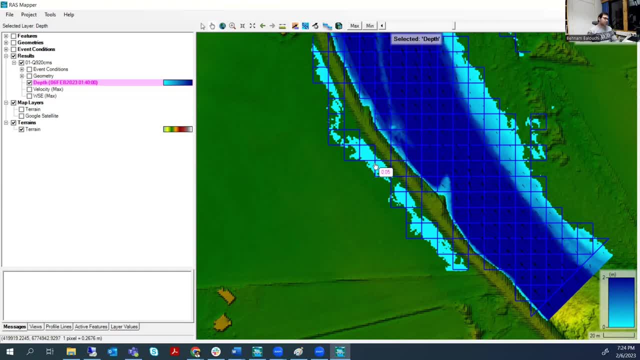 them is in the on the wall, then the water from these cells coming, then the water from these cells coming, then the water from these cells coming here, here, here, and what's happened to the connectivist and what's happened to the connectivist and what's happened to the connectivist cells that i show you. it shows the. 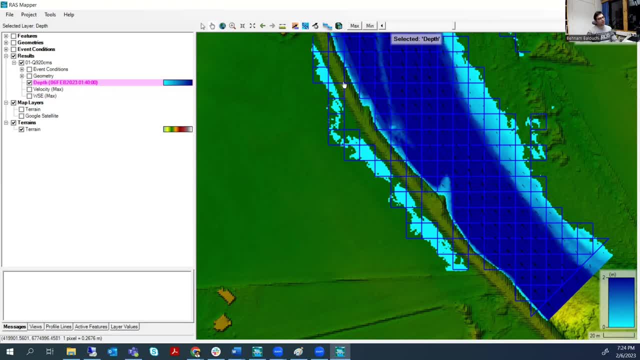 cells that i show you. it shows the cells that i show you. it shows the connection of the cells, connection of the cells, connection of the cells. you can see the water. one comes here, the. you can see the water. one comes here, the. you can see the water. one comes here, the water comes from here, these cells. 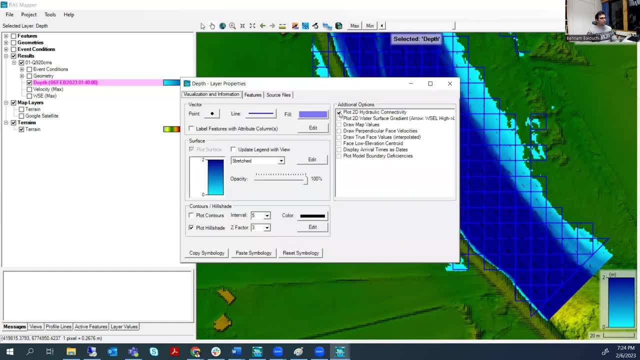 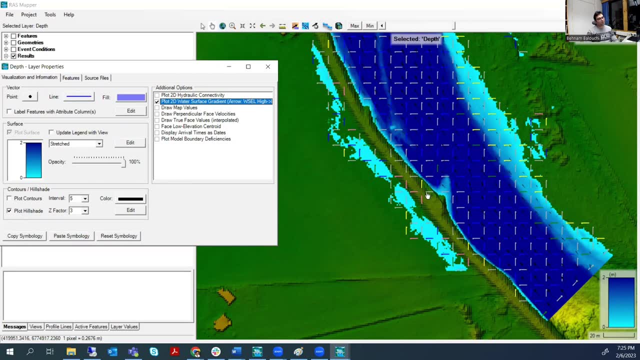 water comes from here, these cells. water comes from here, these cells, and here and here and here. you have also other, you have also other, you have also other parameters, parameters, parameters. 2d gravitation- it's, we have various. 2d gravitation- it's, we have various. 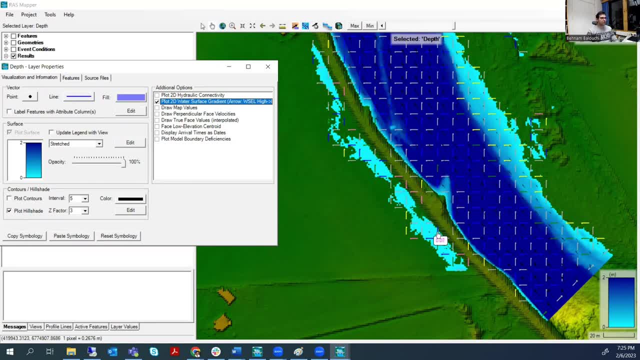 2d gravitation it's. we have various vectors here, vectors here, vectors here. each vectors show different. each vectors show different. each vectors show different options. options: the blue vector is a normal fellow. the blue vector is a normal fellow. the blue vector is a normal fellow. the green one here is a intermediate. 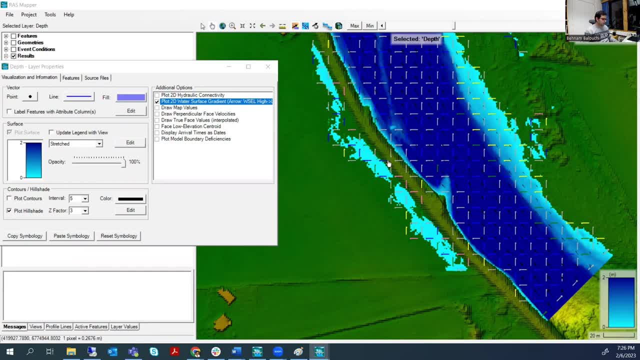 the green one here is a intermediate. the green one here is a intermediate fellow depth, fellow depth, fellow depth. the yellow one is the shallow fellow. the yellow one is the shallow fellow. the yellow one is the shallow fellow depth- here for example depth, here for example depth. here for example, the peak. the pink one: 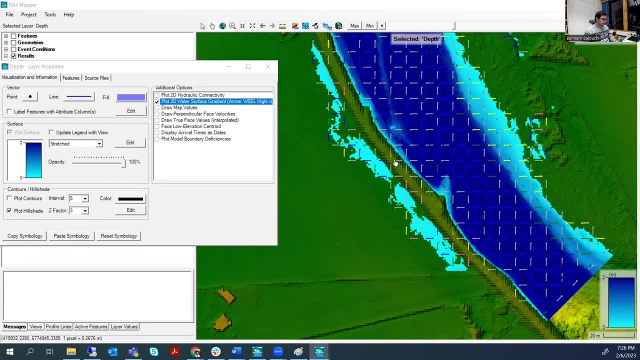 the peak, the pink one. the peak, the pink one is the critical depth and the gray one is the critical depth. and the gray one is the critical depth and the gray one is a back water is a back water, is a back water. it's like the hydraulic connectivity. 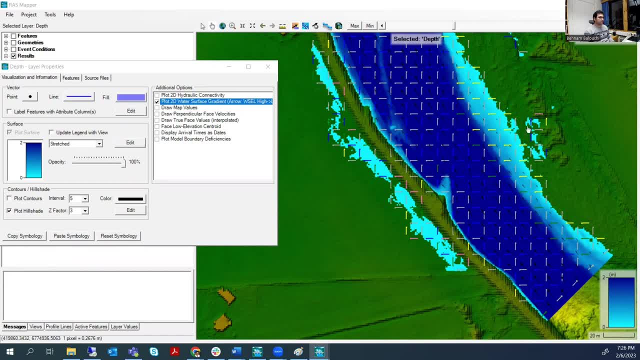 it's like the hydraulic connectivity. it's like the hydraulic connectivity. shows you the errors which says the. shows you the errors which says the. shows you the errors which says the water goes from. water goes from. water goes from which cells and coming from which cells? which cells and coming from which cells. 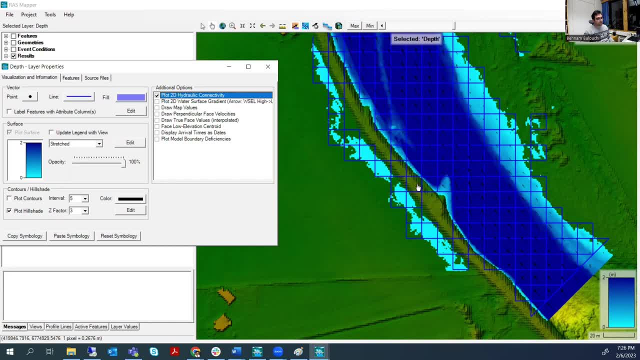 which cells and coming from which cells. but i, but i, but i really um like this one, especially for really um like this one, especially for really um like this one, especially for the not so professional, the not so professional, the not so professional modeling, and also you have others for. 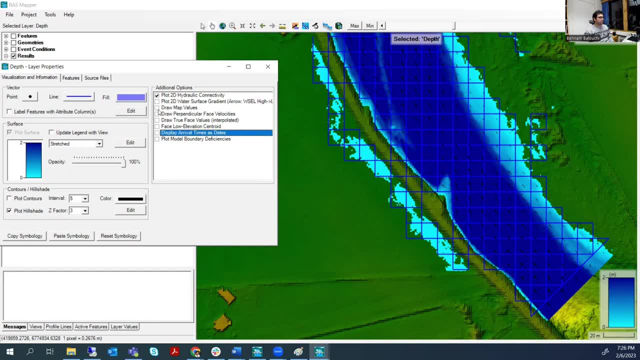 modeling and also you have others for modeling and also you have others, for example, display arrival time, or example display arrival time or example display arrival time, or other parameters that you can use here, other parameters that you can use here, other parameters that you can use here, and they are useful. 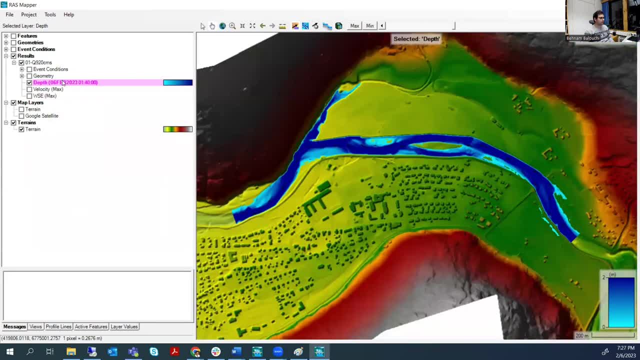 and they are useful. and they are useful. then you have zoom to layer, you can. then you have zoom to layer, you can. then you have zoom to layer. you can zoom to layer like this and zoom to layer like this, and zoom to layer like this and also see the results. 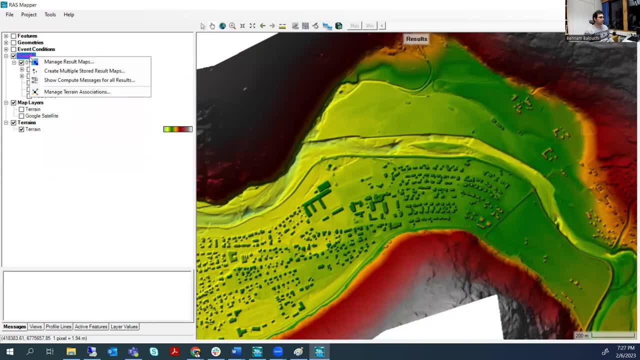 also see the results. also see the results if you click on right click on this. if you click on right click on this, if you click on right click on this: manage the results. manage the results. manage the results. here you can add each results that you. here you can add each results that you. 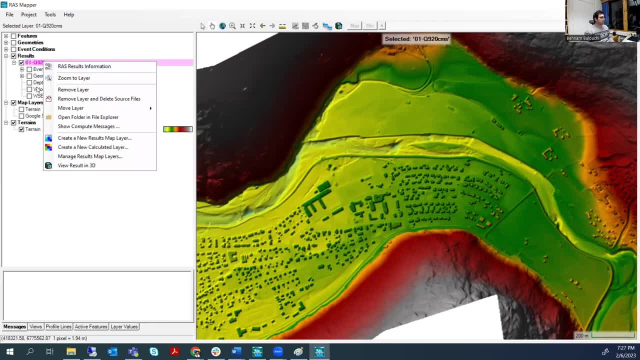 here you can add each results that you want for different, want for different, want for different geometry. or here create new results: geometry. or here create new results: geometry. or here create new results. so you have hydraulics or 2d hydraulics. so you have hydraulics or 2d hydraulics. 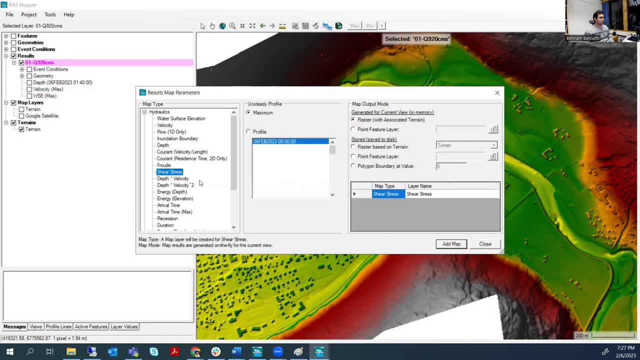 so you have hydraulics or 2d hydraulics in hydraulics, for example. you can use in hydraulics, for example, you can use in hydraulics, for example, you can use the: the, the shear stress, shear stress, shear stress. you should wait till this finish or other. 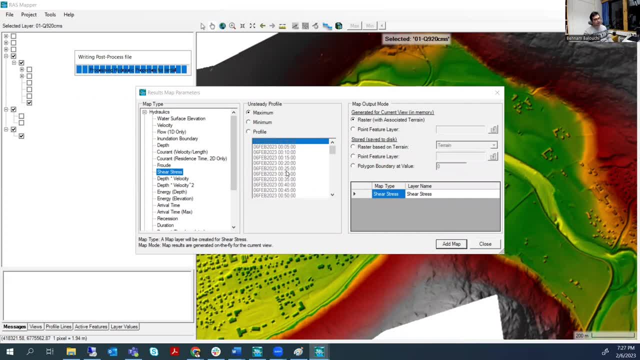 you should wait till this finish or other. you should wait till this finish or other parameters that you have and you can parameters that you have and you can parameters that you have and you can also choose a specific time for you. if also choose a specific time for you, if. 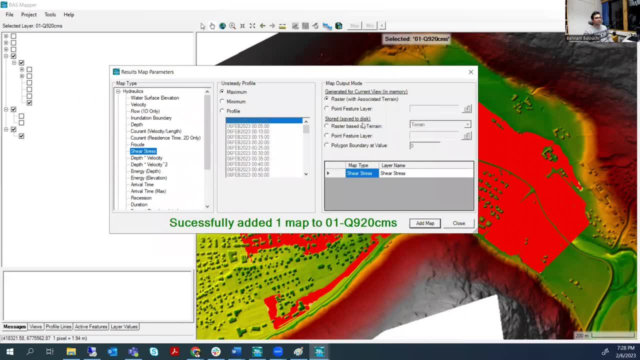 also choose a specific time for you. if you want to save it, you want to save it. you want to save it as a train file and as a train file and as a train file and open it in the open it in the open it in the arc gis. i recommend to use this. 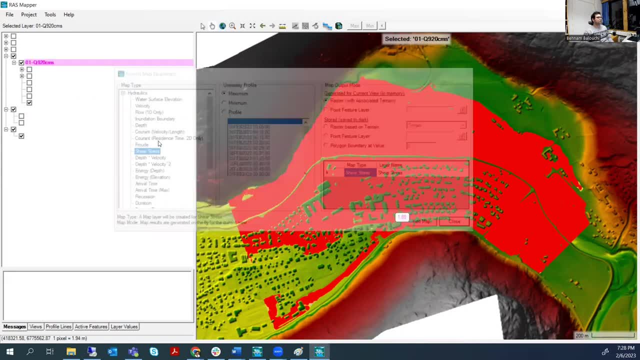 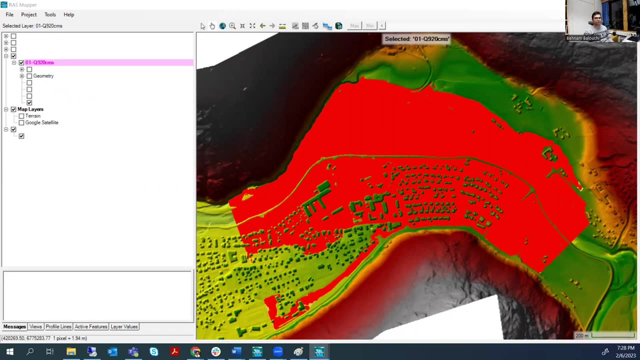 arc gis. i recommend to use this arc gis. i recommend to use this option, option, option here, this one. so here, for example, we can see the. so here, for example, we can see the. so here, for example, we can see the results. so here it's a shear stress for. 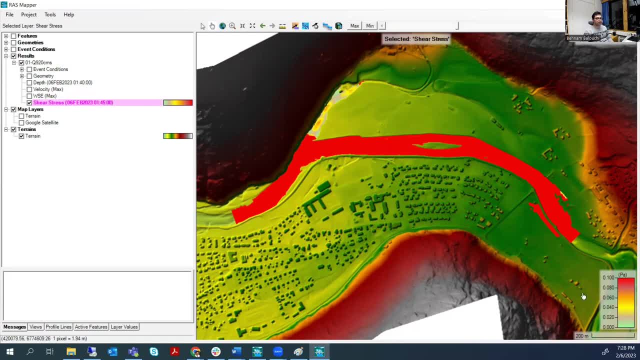 so here it's a shear stress for. so here it's a shear stress for a specific time. you can see it's 50 a specific time. you can see it's 50 a specific time. you can see it's 50 around 50.. so if we want to change this, 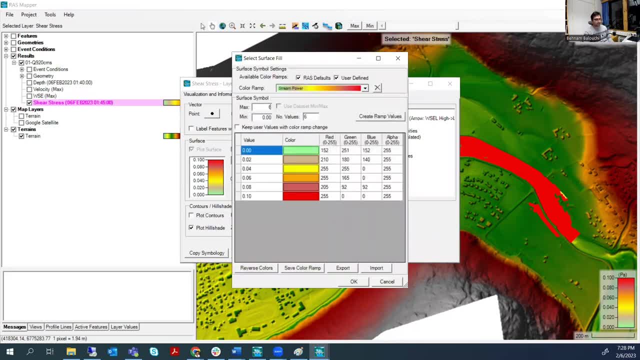 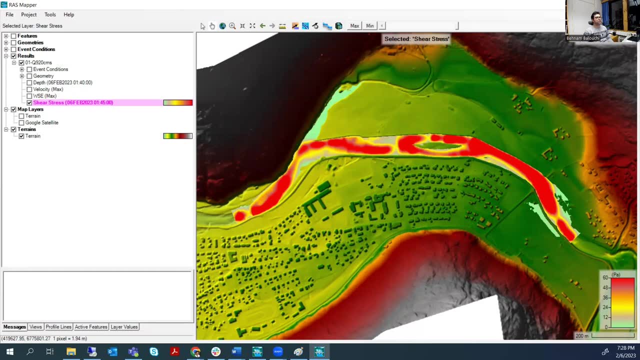 around 50. so if we want to change this around 50, so if we want to change this, so like from 0 to so like from 0 to so like from 0 to till 60, you can see the results of shear stress. you can see the results of shear stress. 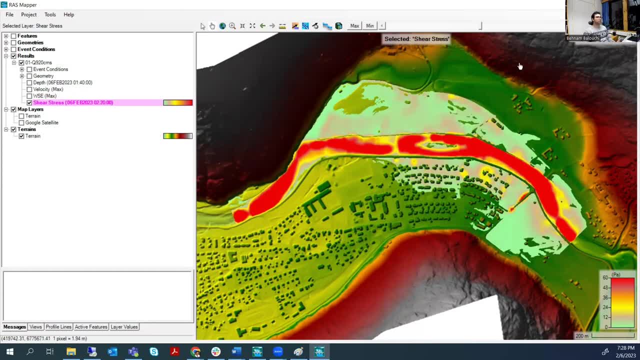 you can see the results of shear stress, and, and, and. if you play it, it's increased, or you, if you play it, it's increased, or you, if you play it, it's increased, or you. you can see the results of. you can see the results of. you can see the results of fruit, or, if i right click on it. 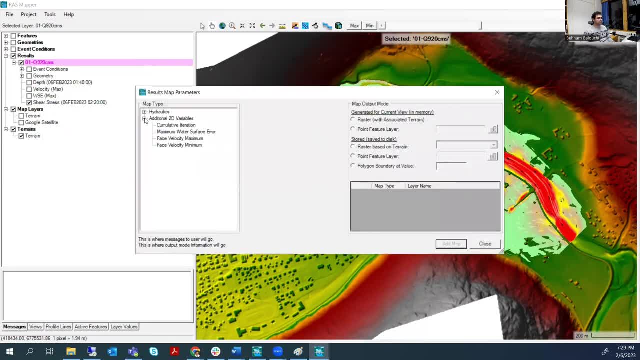 then go to the create new results, then go to the create new results, then go to the create new results and to the additional 2d variable if. and to the additional 2d variable if. and to the additional 2d variable if you want to check your results. 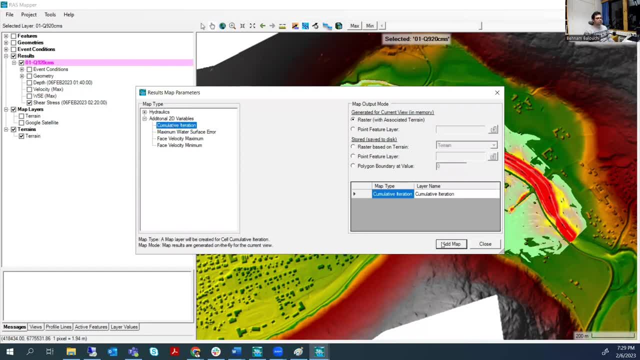 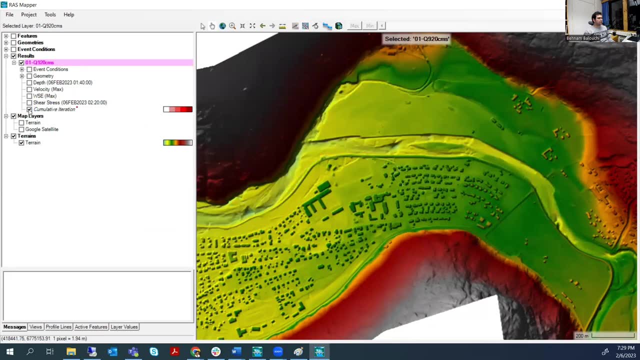 you want to check your results. you want to check your results. here you have a cumulative iteration. here you have a cumulative iteration. here you have a cumulative iteration, if you click on this, especially for the- when you have a, especially for the when you have a, especially for the when you have a sediment. 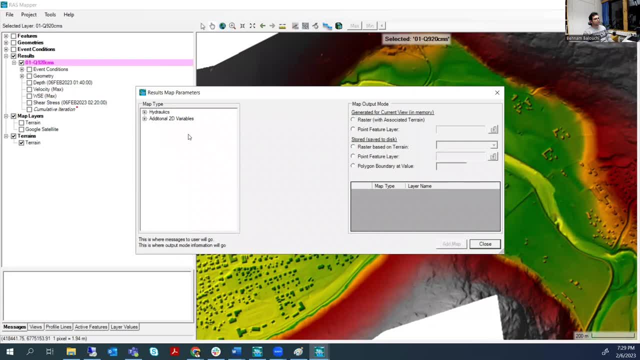 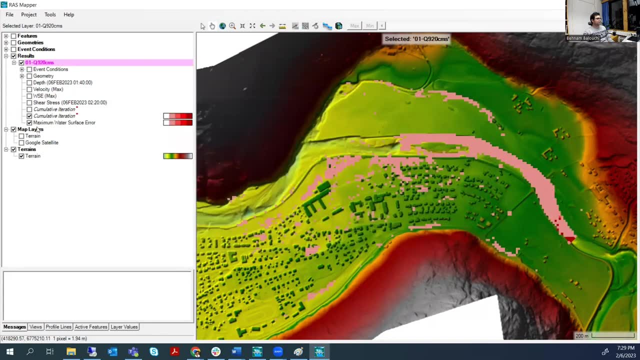 sediment, sediment. this option, it's useful. cumulative iteration or maximum water. cumulative iteration or maximum water. cumulative iteration or maximum water surface error. so here, so here, so here, we don't have any, we don't have any, we don't have any, uh uh. cumulative, special cumulative iteration. 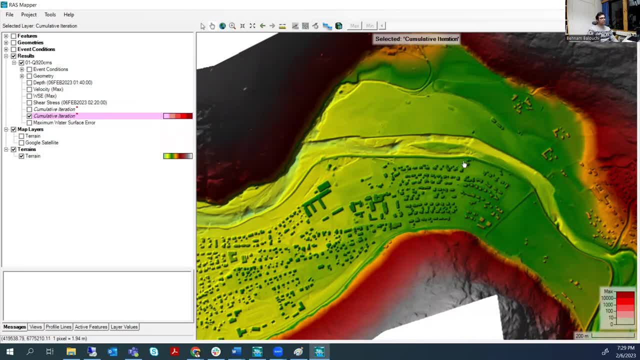 cumulative, special cumulative iteration, cumulative, special cumulative iteration, and actually it's not and actually it's not and actually it's not reading, but then on the cells you can see reading. but then on the cells you can see reading. but then on the cells you can see, for example, maybe here we have some. 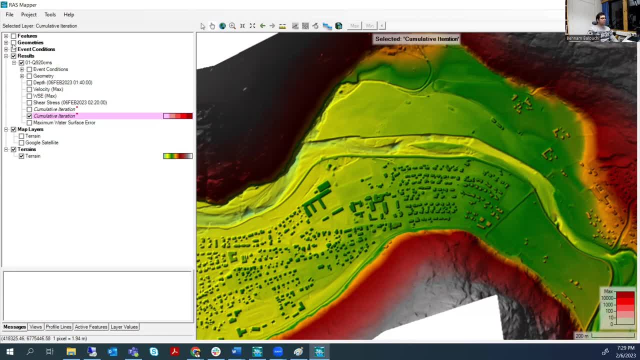 for example, maybe here we have some. for example, maybe here we have some values. or you know where is the problem values, or you know where is the problem values. or you know where is the problem with the mesh and in the geometric you, with the mesh and in the geometric you. 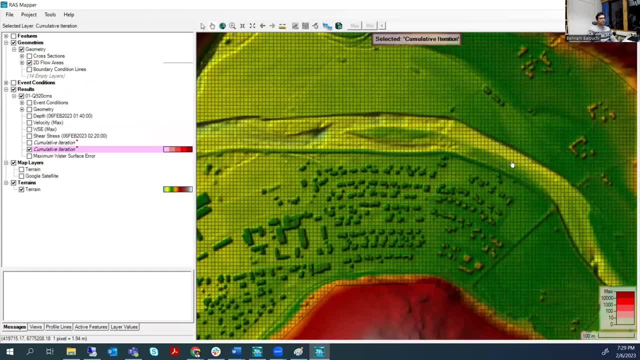 with the mesh and in the geometric you can, can, can show your mesh, show your mesh, show your mesh. here you can see the mesh, here you can see the mesh. here you can see the mesh. and if you have like a cumulative, and if you have like a cumulative, 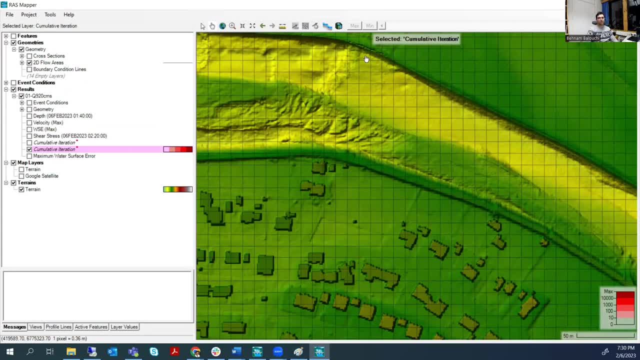 and if you have like a cumulative errors, cumulative iteration, here you errors, cumulative iteration, here you errors. cumulative iteration, here you. so there is a problem most probably with. so there is a problem most probably with. so there is a problem most probably with the mesh or with the slope that you have. 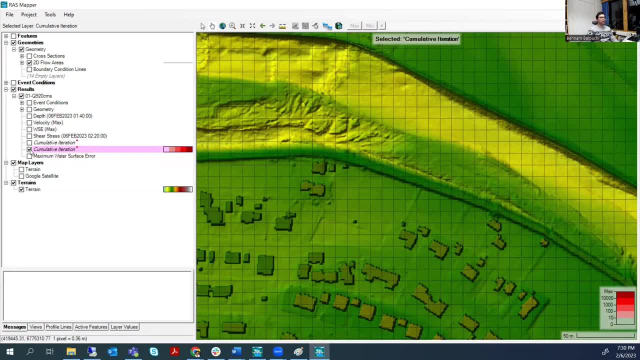 the mesh or with the slope that you have the mesh or with the slope that you have here, and you should fix the problem here and you should fix the problem here and you should fix the problem. i explain a little about how to fix the. i explain a little about how to fix the. 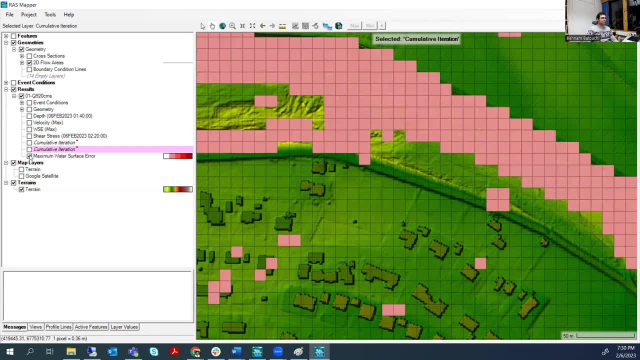 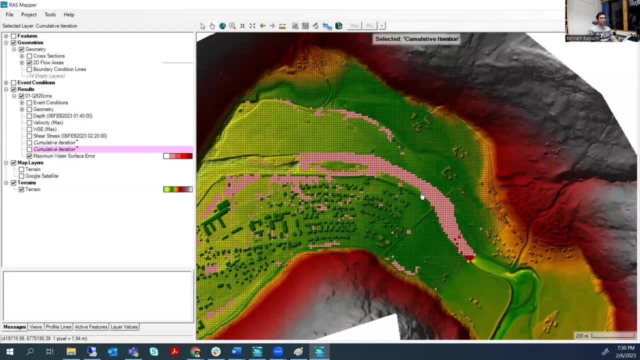 i explain a little about how to fix the problem for the problem, for the problem for the mesh, and then maximum water surface mesh, and then maximum water surface mesh and then maximum water surface error. you can see the points that we have for. you can see the points that we have for. 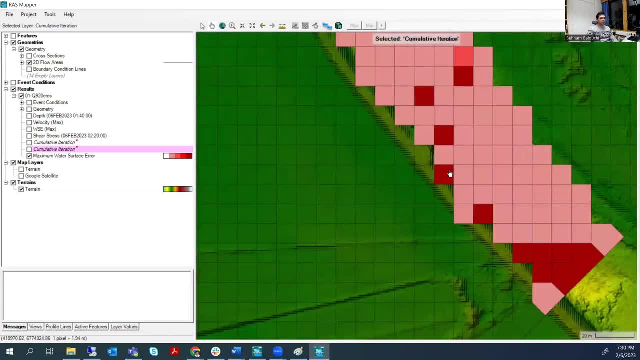 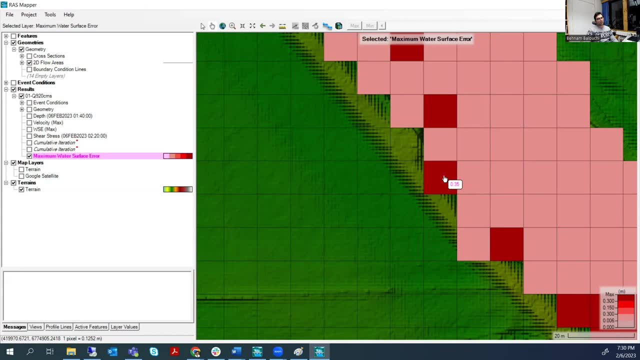 you can see the points that we have, for example, example, example. here we have a huge maximum iteration, it's, we have a huge maximum iteration, it's, it's a maximum point, it's a maximum point. it's a maximum point so we can go and fix it. so one reason is: 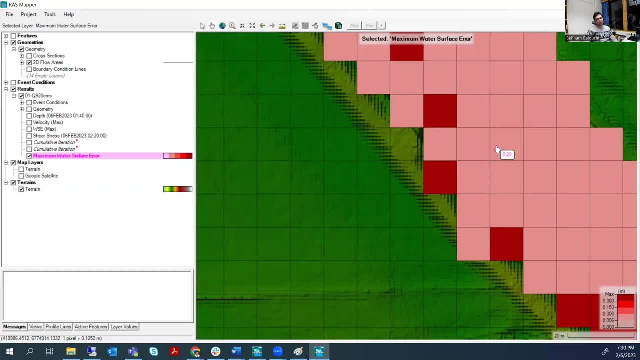 so we can go and fix it. so one reason is: so we can go and fix it. so one reason is that this cell, that this cell, that this cell is half of on the river ridge and half of is half of on the river ridge and half of. 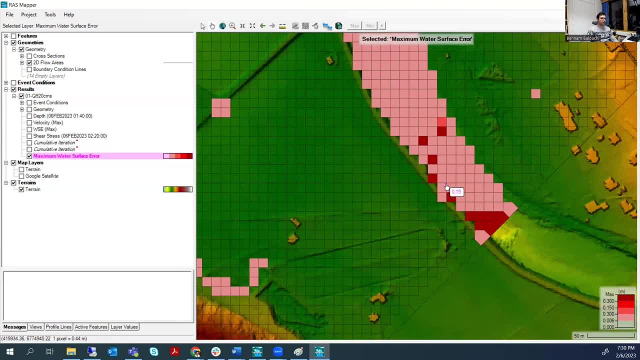 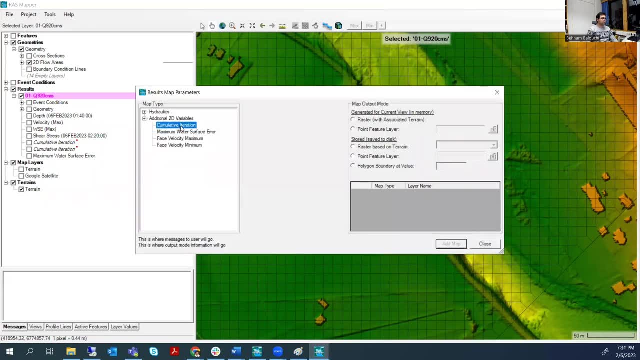 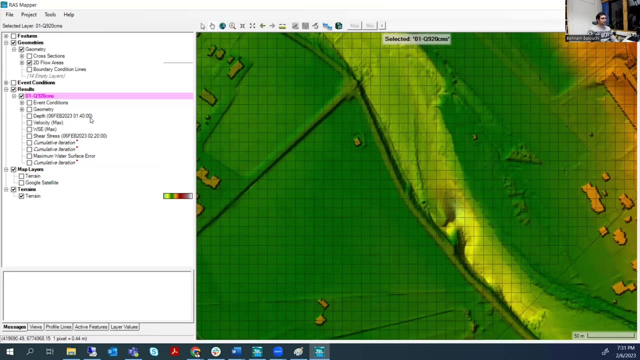 is half of on the river ridge and half of of them on the of them, on the of them on the wall. let me, if i can, so we don't have this result now. so we don't have this result now. so we don't have this result now. okay then, i think. 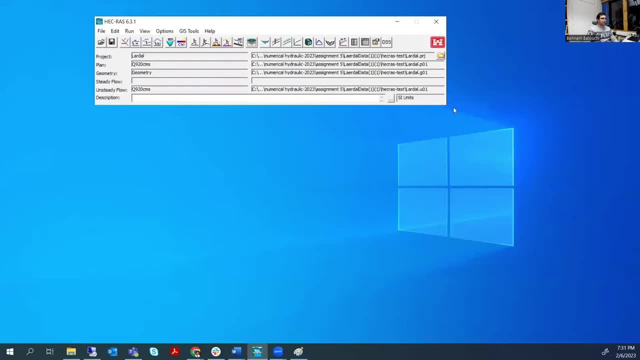 okay, then, i think okay, then i think we, we, we are finished here, so i close it. we are finished here, so i close it, we are finished here, so i close it. so then, if you need to so, then if you need to, so, then if you need to have another run for another discharge. 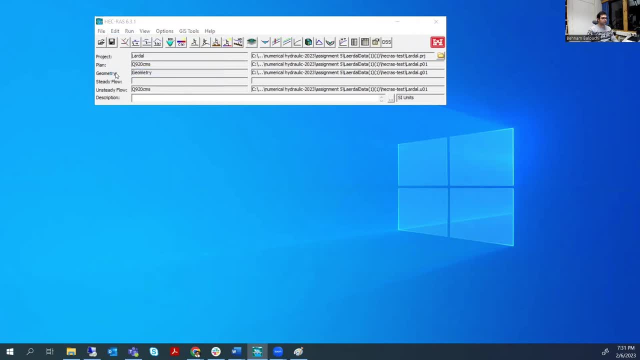 have another run for another discharge. have another run for another discharge again. go to the again. go to the again. go to the unsteady fellow data and change the unsteady fellow data and change the unsteady fellow data and change the parameters here and then save as as. 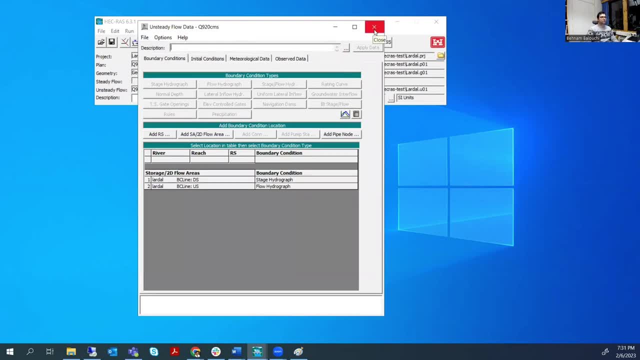 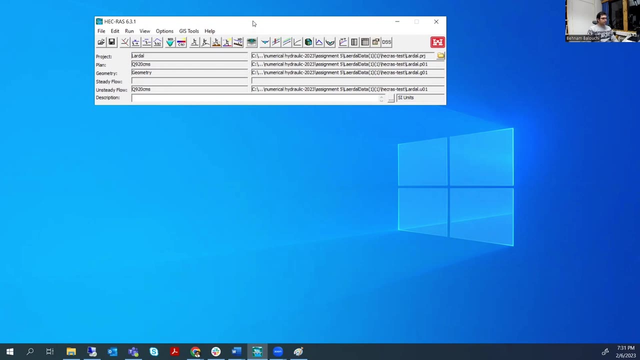 parameters here and then save as as parameters here and then save as as as another flow data like q620 cms flow data like q620 cms flow data like q620 cms or cubic meter or cubic meter or cubic meter per per per second. so now, so now. 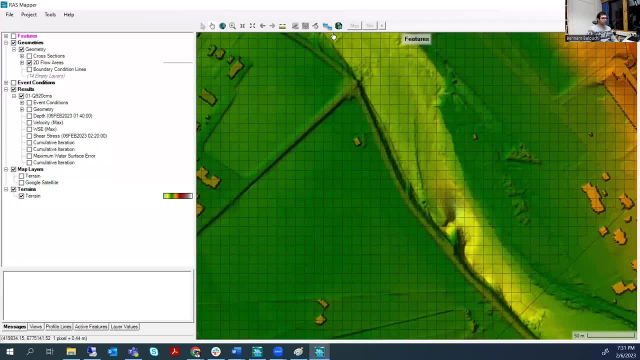 so now, i would like to show you the 3d results. i would like to show you the 3d results. i would like to show you the 3d results. so let's see, so, let's see, so let's see the depth, the depth. 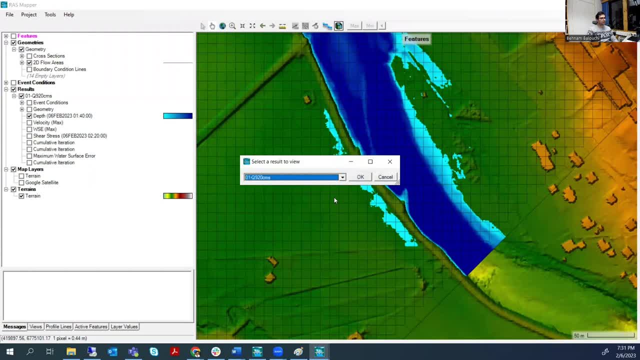 the depth. here it's great, here it's great, here it's great. then go to the, then go to the, then go to the 3d results and okay, yes, so here in the, so here in the, so here in the 3d, 3d. 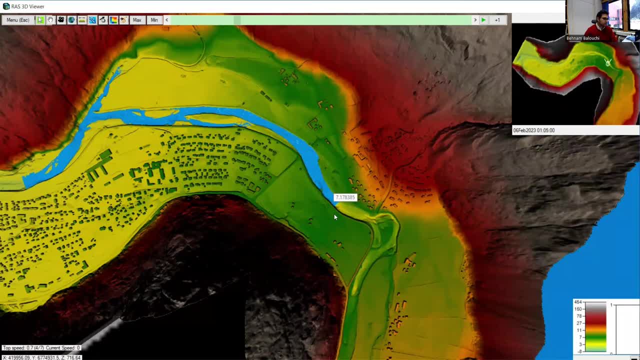 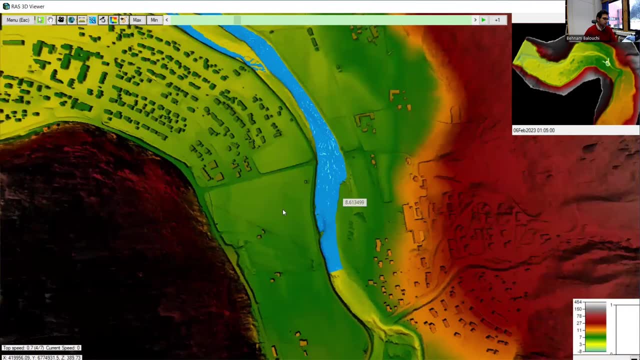 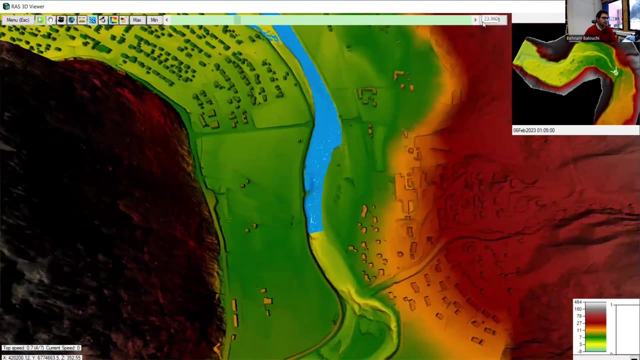 3d view. we should 3d view. we should 3d view. we should zoom a little, zoom a little, zoom a little and then by and then by, and then by right click you can turn it. and i played. you can see the here here. 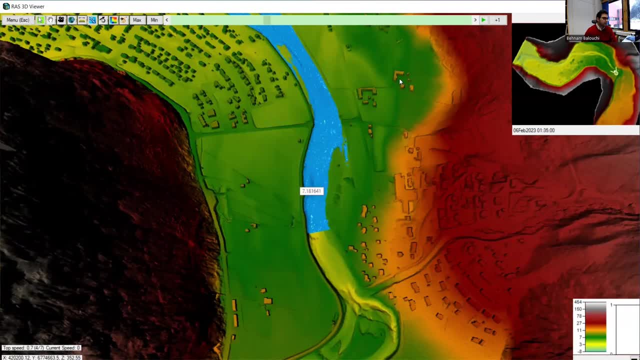 here. you see that we have a. you see that we have a. you see that we have a: watercomings, watercomings, watercomings- from these cells, but we have a from these cells, but we have a from these cells, but we have a wall. so data wall is more than the. 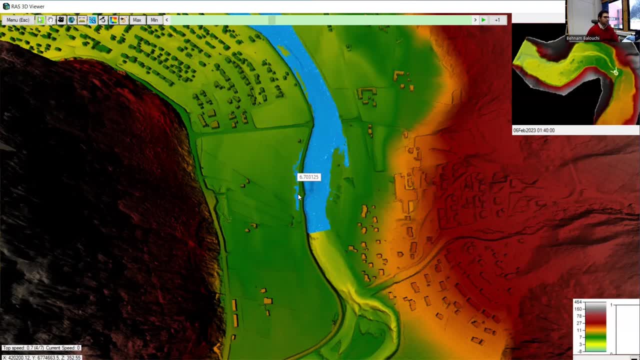 wall. so data wall is more than the wall. so data wall is more than the water elevation. so water elevation, so water elevation. so we shouldn't have any water here. so we shouldn't have any water here. so we shouldn't have any water here. so what should we do? 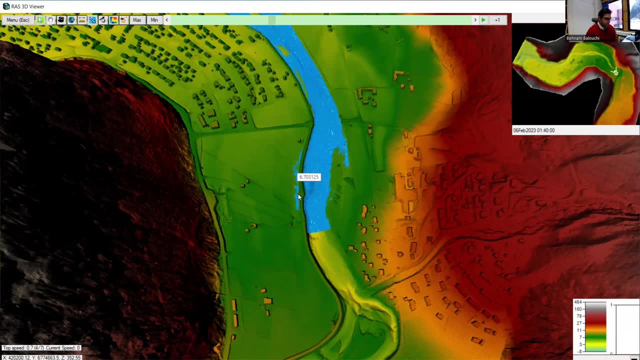 what should we do? what should we do? we should go to the geometry, we should go to the geometry, we should go to the geometry data, and then we have two options: first data, and then we have two options: first data, and then we have two options: first to use break lines to 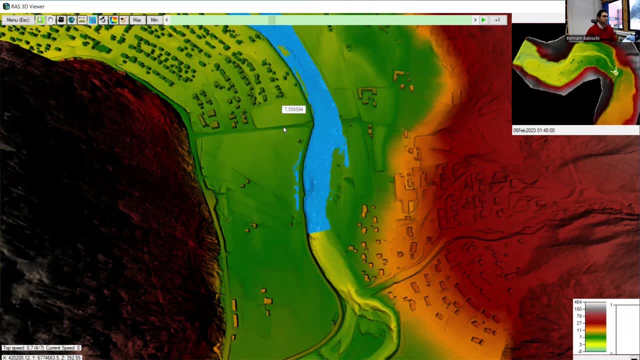 to use break lines to to use break lines to modify the mesh and then modify the mesh, and then modify the mesh. and then we should, we can use the refine, we should, we can use the refine, we should, we can use the refine, a mesh. so i am going to that and show. 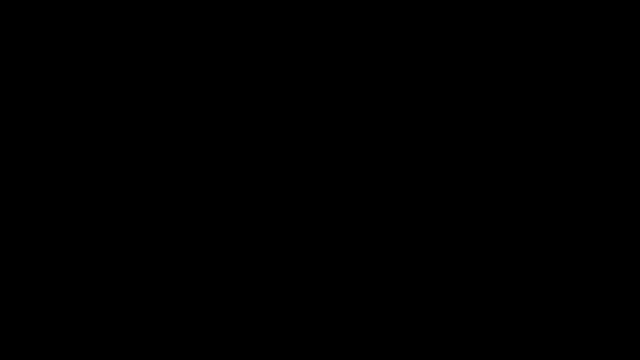 a mesh. so i am going to that and show a mesh. so i am going to that and show you, you, you, how to work first with break lines. so what should we do for fixing this? so what should we do for fixing this? so what should we do for fixing this problem? we should have a break lines and 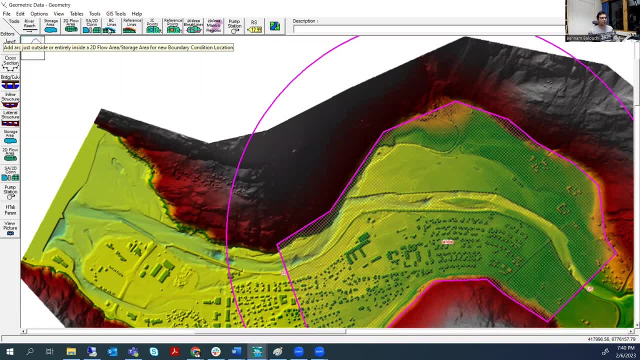 problem: we should have a break lines and problem: we should have a break lines. and i recommend, i recommend, i recommend to make this, to make this, to make this at the starting point of your defining the mesh. i just do it now. defining the mesh. i just do it now. 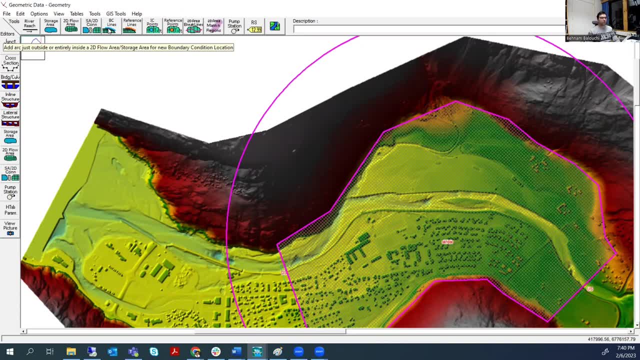 defining the mesh. i just do it now because i want first you learn what is because i want first you learn what is because i want. first you learn what is the difference and what is your options- the difference and what is your options- the difference and what is your options. so 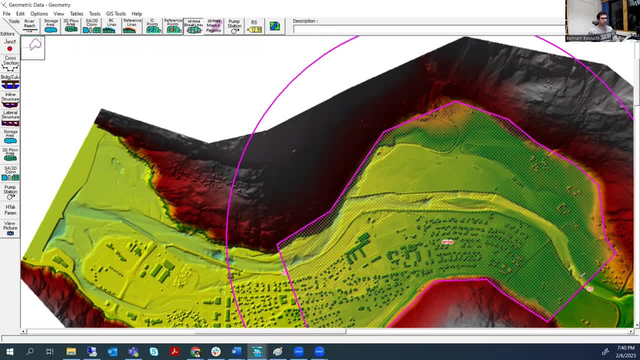 so. so we are going to the, we are going to the, we are going to the 2d break lines and then 2d break lines, and then 2d break lines, and then- i just make it so fast here, but you, i just make it so fast here, but you. 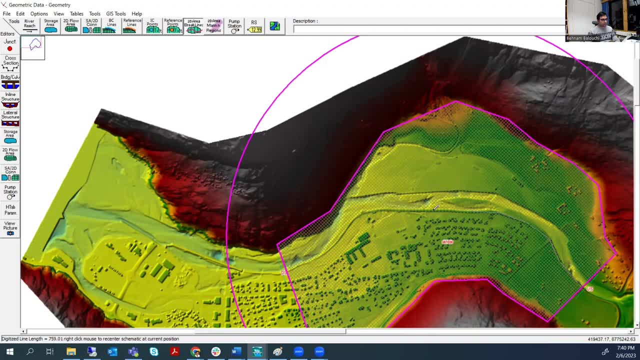 i just make it so fast here, but you should have a details on that and put time to have a details on that and put time to have a details on that and put time to have a good, good, good, defining, defining, defining. so i make it as a 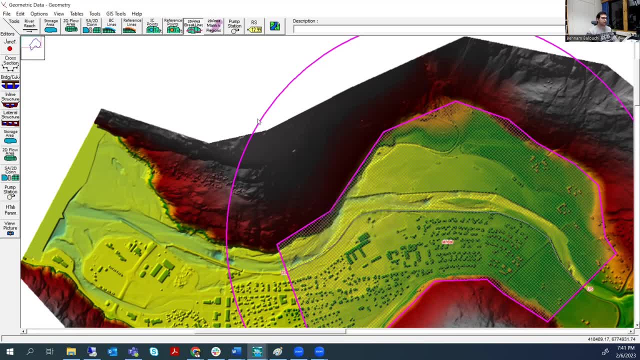 left, left, left break line, break line, break line, and then okay then, and then okay then, and then okay, then i should, i should, and then okay, then i should also introduce another one as a right. so right correct line. it is very, very important especially. it is very, very important especially. 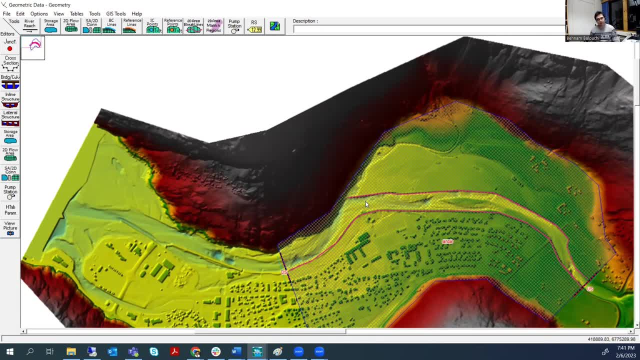 it is very, very important, especially when you have a, when you have a, when you have a, it depends when you have another format, it depends when you have another format, it depends when you have another format of the river. you should of the river. you should of the river. you should define break line as a bottom of the 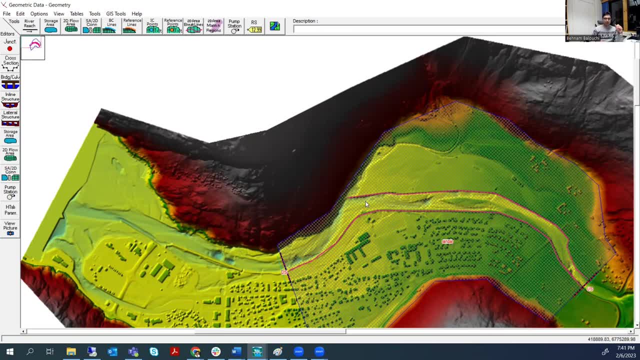 define break line as a bottom of the. define break line as a bottom of the your bank and at the top of your bank or your bank and at the top of your bank or your bank and at the top of your bank or flat plane, and one at the middle of the. 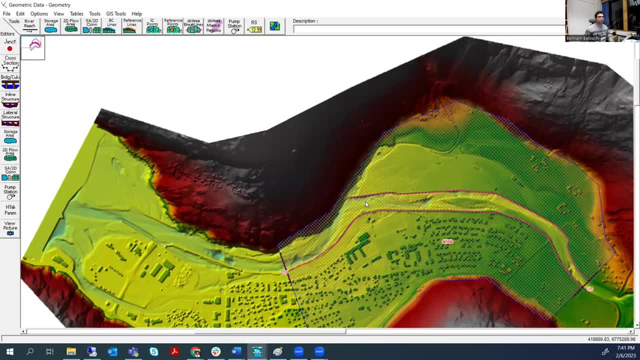 flat plane and one at the middle of the flat plane and one at the middle of the river or the center line of the river river or the center line of the river river or the center line of the river. and how to and how to and how to choose the center line. i explain it in. 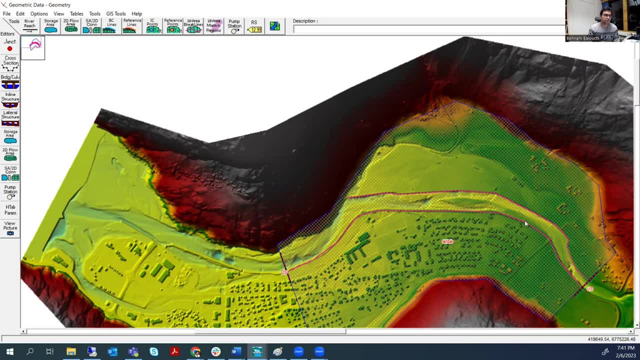 choose the center line. i explain it in: choose the center line. i explain it in: uh previous video for the 1d modeling. uh previous video for the 1d modeling. uh previous video for the 1d modeling. you should, you, should, you should choose the. you should go to the. 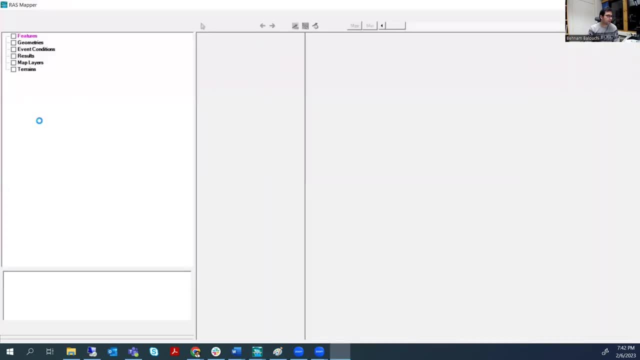 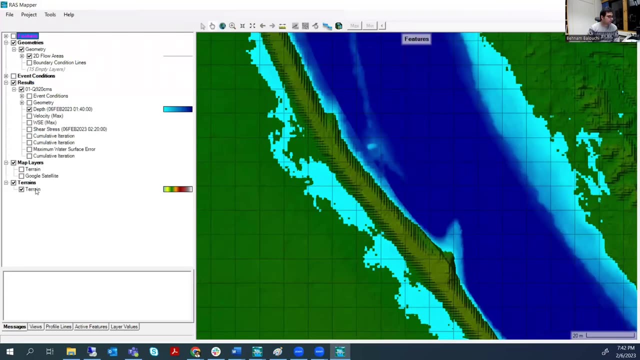 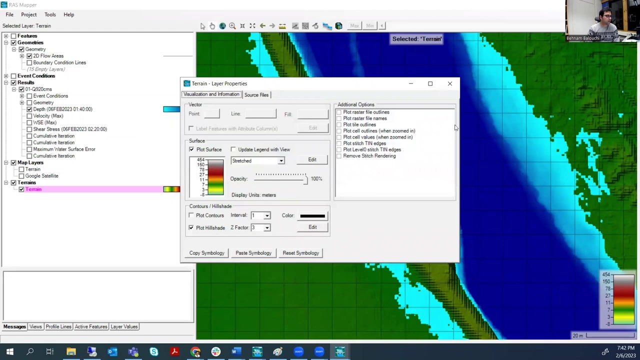 grass mapper and then choose the contour lines. for example, here you contour lines. for example, here you contour lines. for example, here you should go to the double click and you can use the contour line, and, and you can use the contour line, and and you can use the contour line, and then you can see. 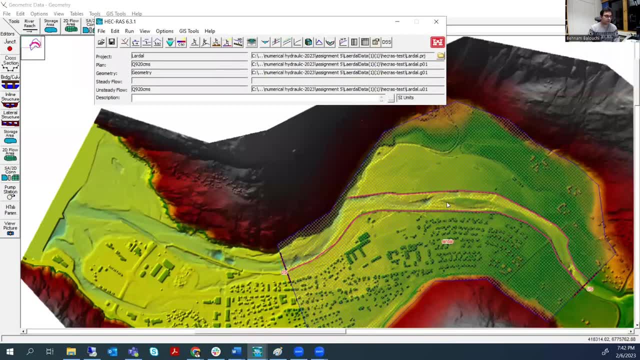 then you can see, then you can see the con various contours and you can the con various contours and you can the con various contours, and you can easily find the bottom of the river, easily find the bottom of the river, easily find the bottom of the river. but now we just use these two. 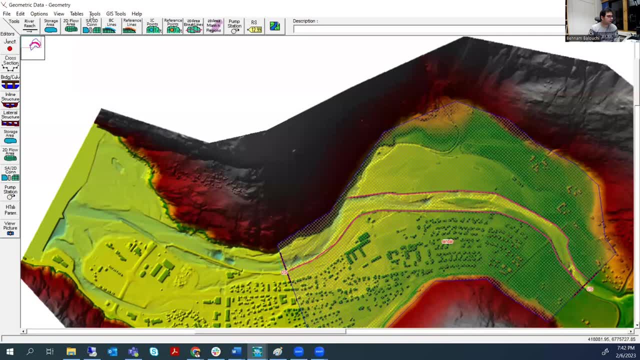 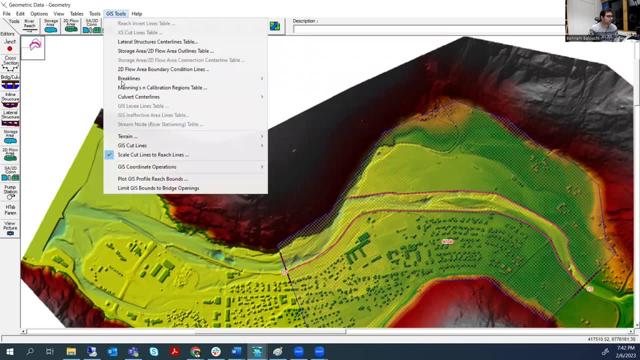 but now we just use these two, but now we just use these two and then, after drawing the two, break, and then after drawing the two, break, and then, after drawing the two break, lines, lines, lines. we are coming here to the, we are coming here to the, we are coming here to the gis tools and then break lines, cell. 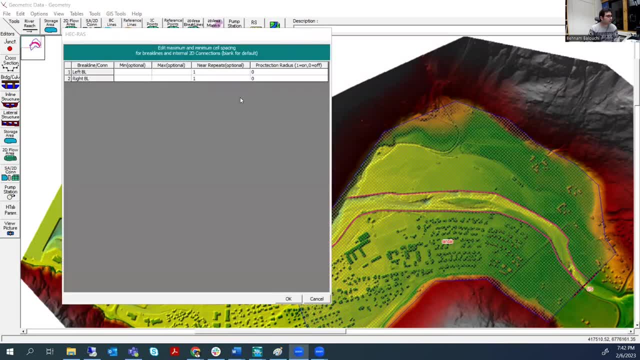 gis tools and then break lines, cell gis tools and then break lines, cell spacing. you can see the various break spacing. you can see the various break spacing. you can see the various break lines that we have here, lines that we have here, lines that we have here: minimum value of the distance from the. 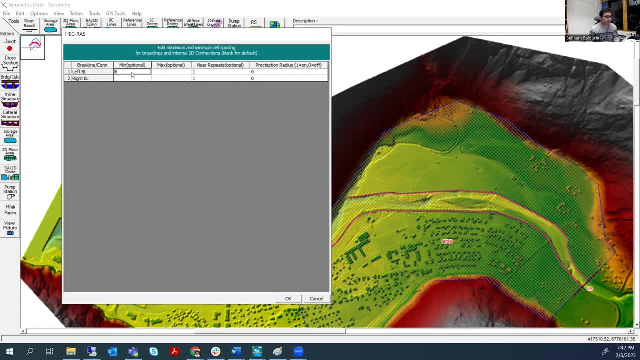 minimum value of the distance from the minimum value of the distance from the break line or the maximum, for example, we break line, or the maximum, for example, we break line, or the maximum, for example. we can make it here as a, can make it here as a, can make it here as a five and here as a five for both. 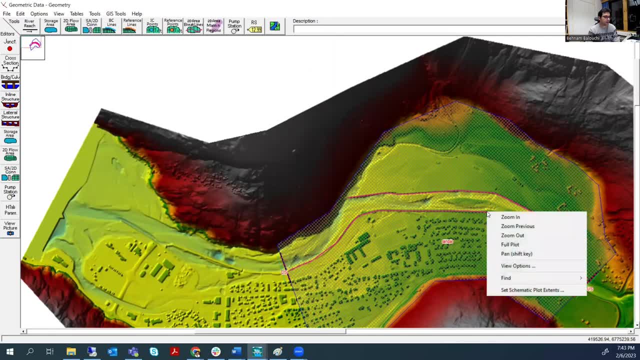 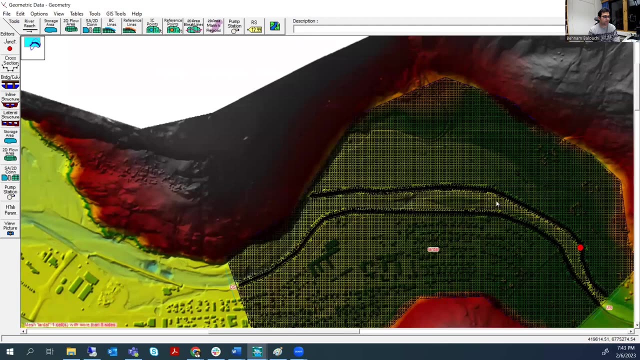 five, and here as a five for both, five and here as a five for both, and then okay, and then okay, and then okay, and then i just write, and then i just write, and then i just write. click on that and enforce break line. here also enforce break line. you can see. 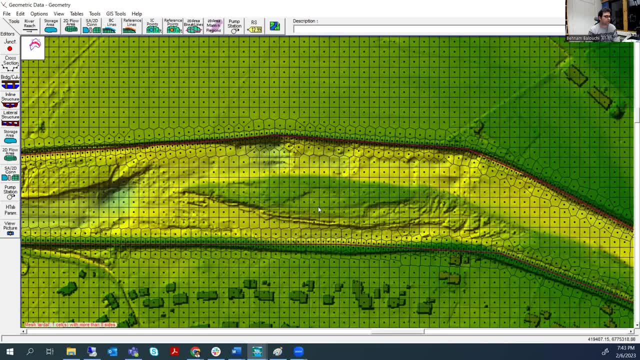 the meshes start from these lines and the meshes start from these lines and the meshes start from these lines, and you can also increase the these values. you can also increase the these values. you can also increase the these values or decrease these values in the that, or decrease these values in the that. 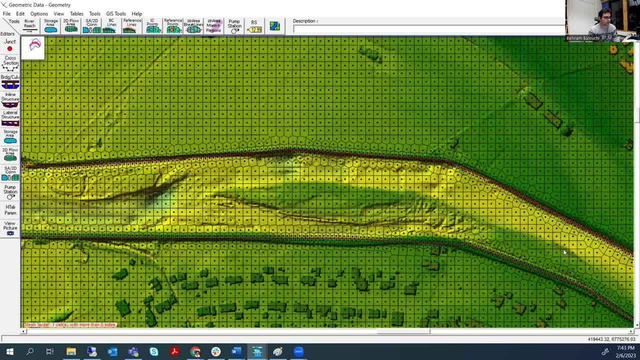 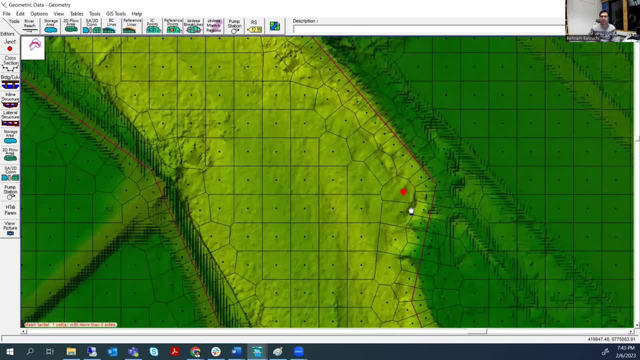 or decrease these values in the that option that you have, but we have a option that you have, but we have a option that you have, but we have a problem here. it defines, it defines one important things for the heckress mesh, it is really important that you don't have a very 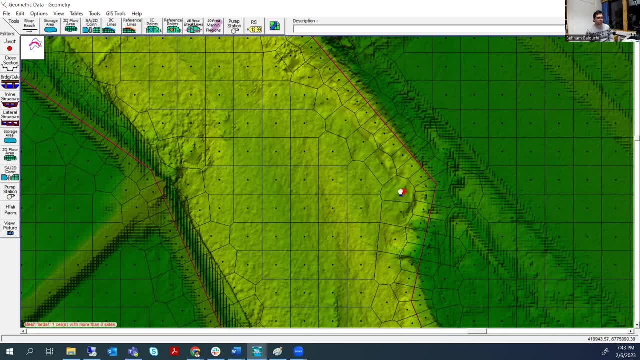 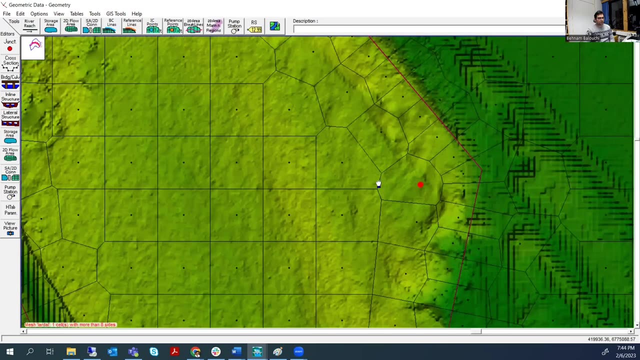 small edges like this one it is better. your mesh is between like four and six like rectangular, but you know these small edges. it's not good for heckress and you have error for that. but if you want to add or remove any points, you can go to the edit: add points or. 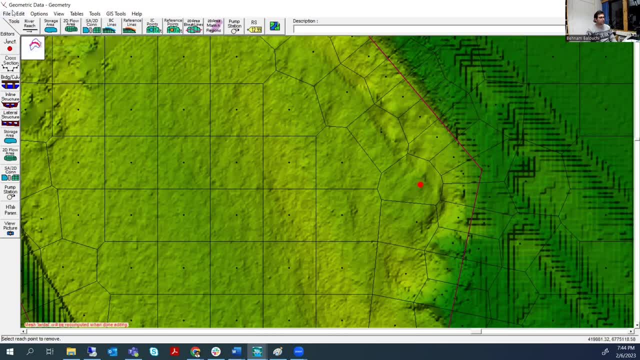 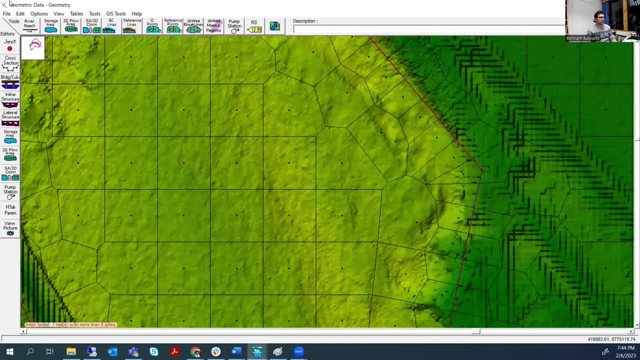 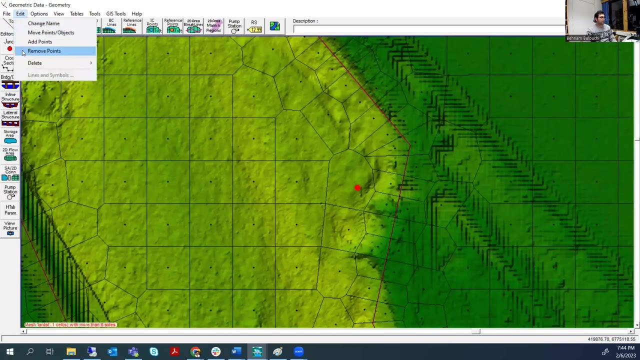 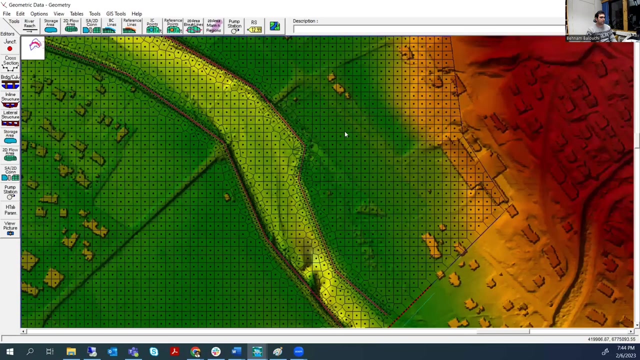 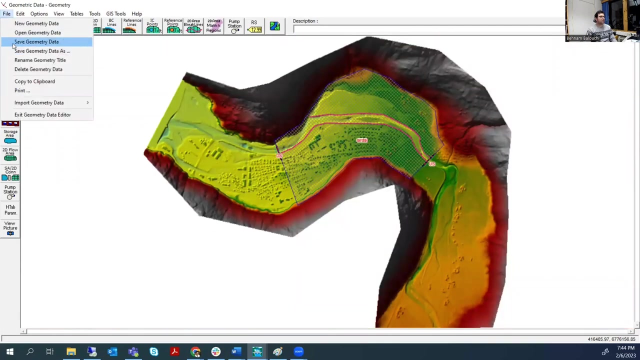 remove points, for example this one, i just remove it. then you can see. you, we have a new mesh, so i just check if we have any other error. so we have another error here so we can remove it, or we can add another point, or right click full plot. so, as you see, it seems the mesh is good without error, so we save it. 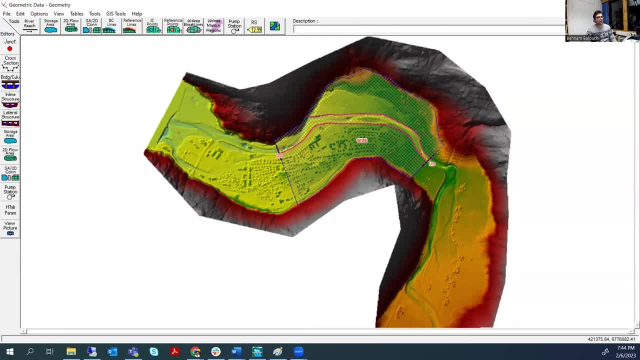 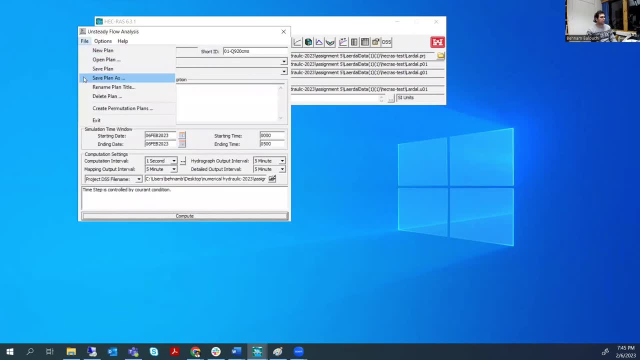 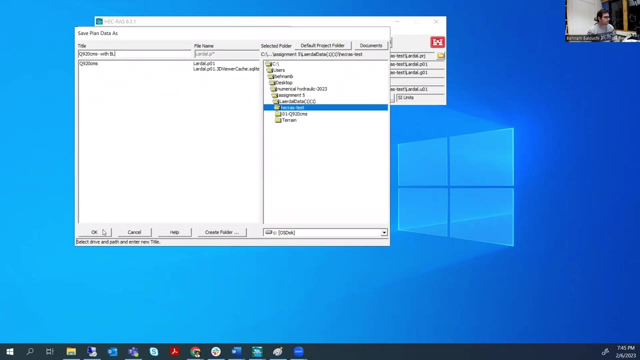 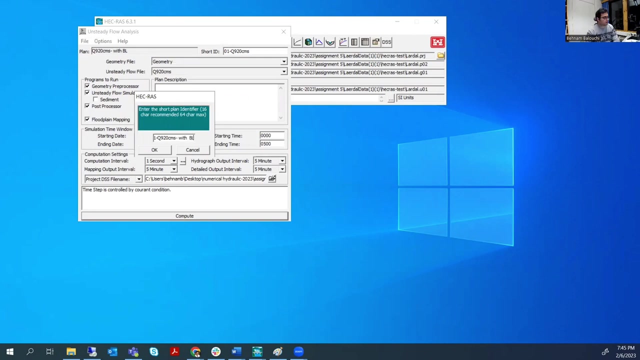 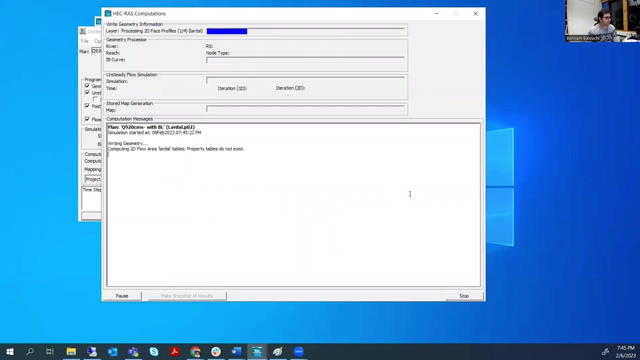 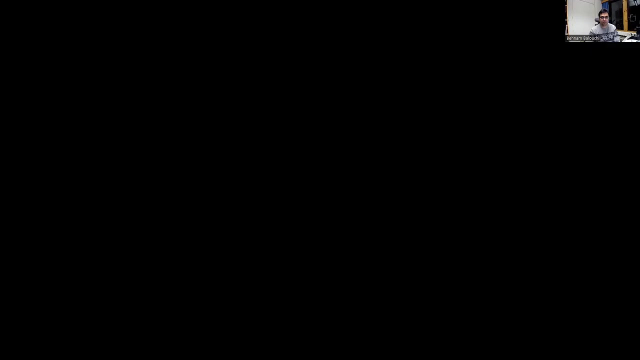 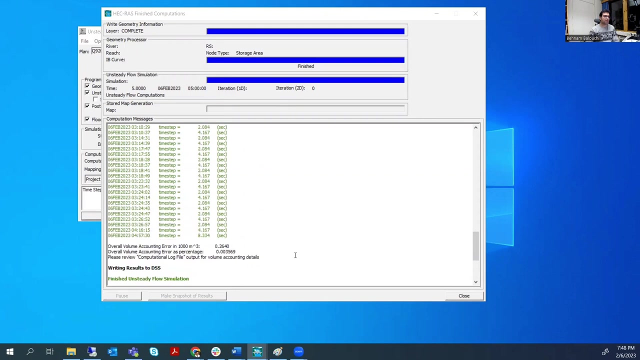 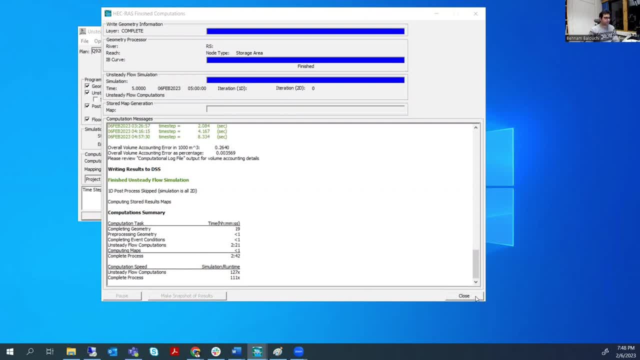 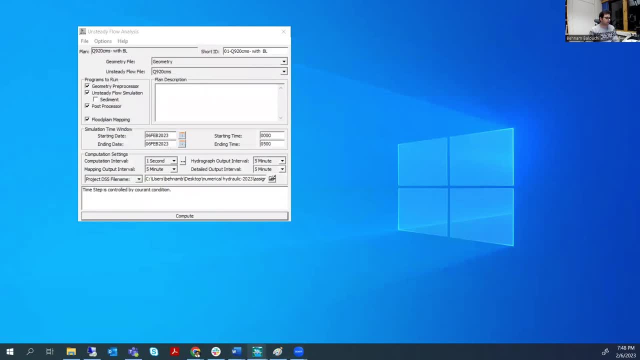 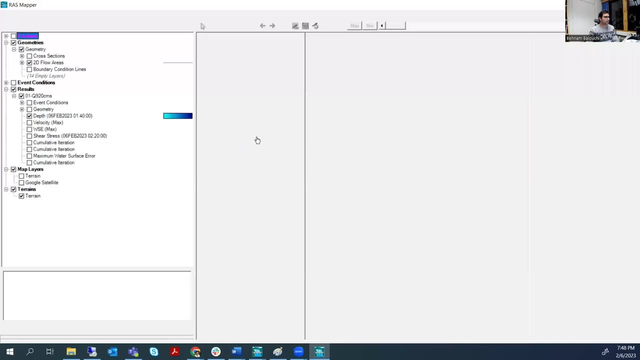 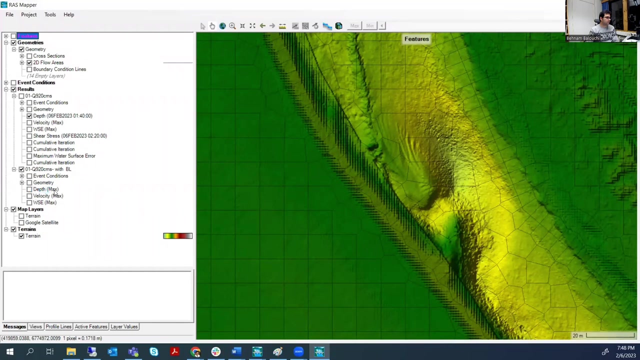 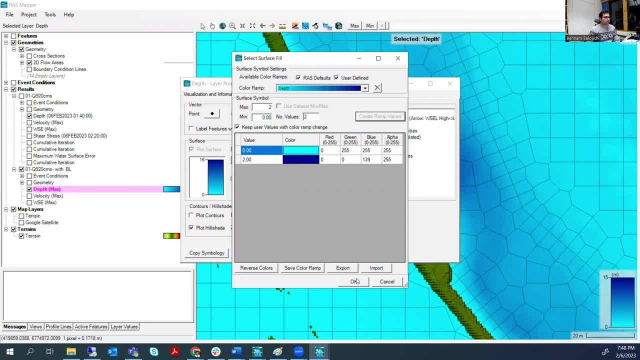 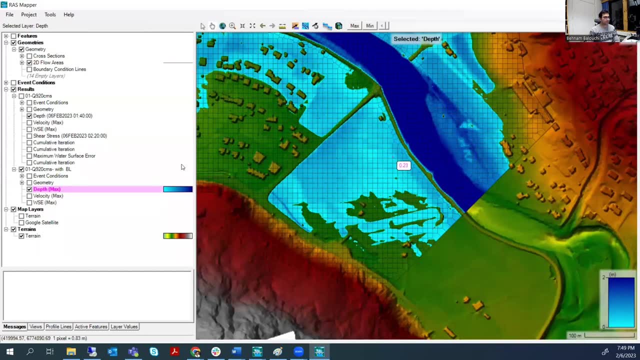 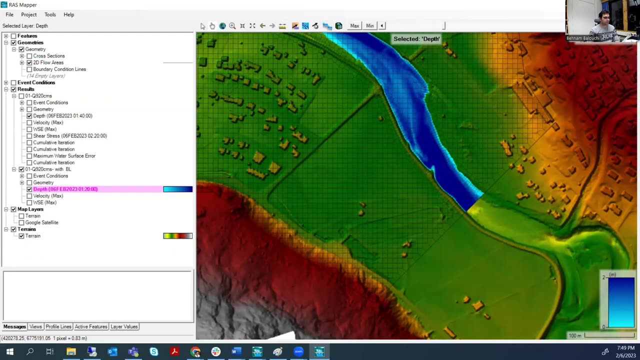 the contour, the maximum of two, then create and okay and then close it. i hope we can fix it. so, as you see it is really, let's see if it is improved. so we have it on 2 and 15, the previous one here. we have it at almost 1 hour and 30 minutes, 35 minutes. but as we improve the results, we 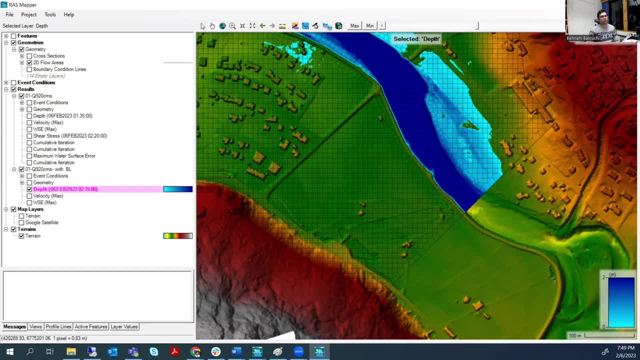 improve the mesh. now we have it on almost 2 hour and 20 minutes, so we have it on 2 and 15, the previous one minutes. so if you do it in a really accurate way, just zoom it and make the break lines very well and use the break lines at the middle of the river, at the bottom of the bank and the top of the bank. 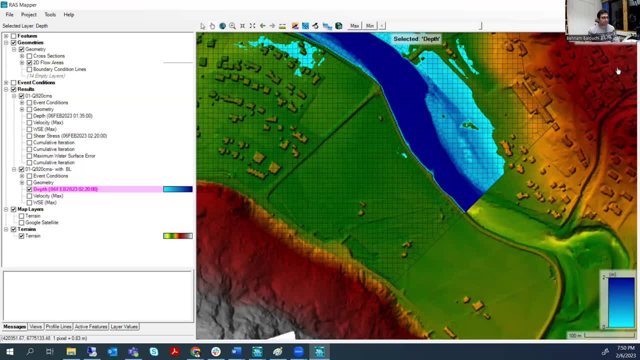 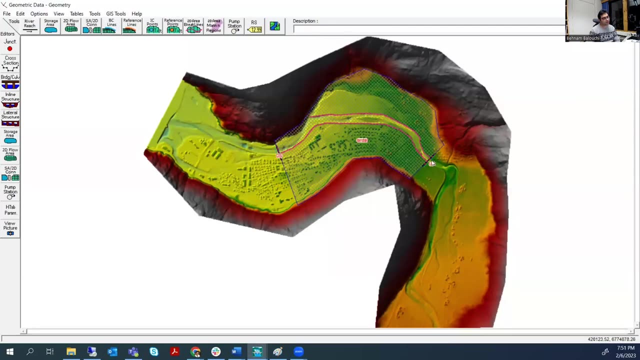 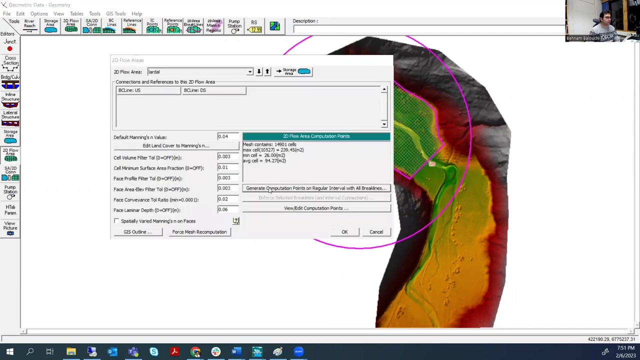 you can have a really good results. very well. the next options for define the mesh: it's, instead of using break line, it's using the refine region. i just go to these break lines and delete the break lines here. delete the break lines and then go to the edit flow and just 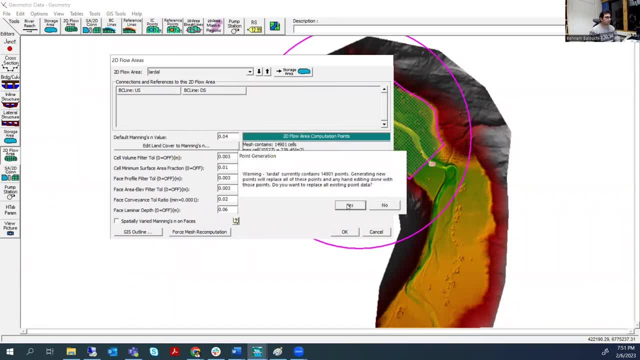 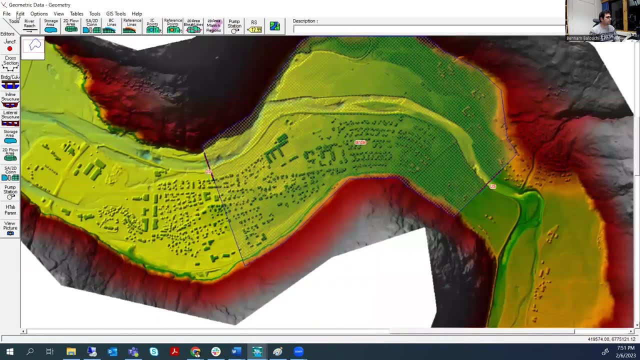 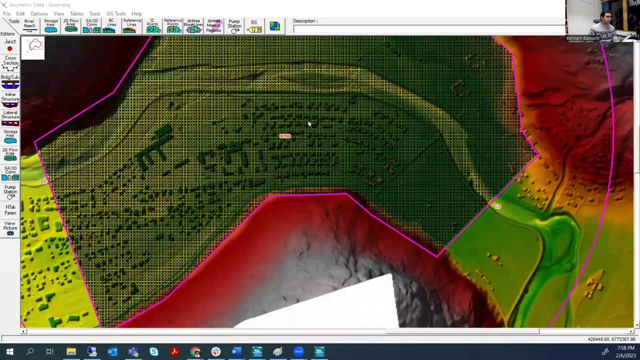 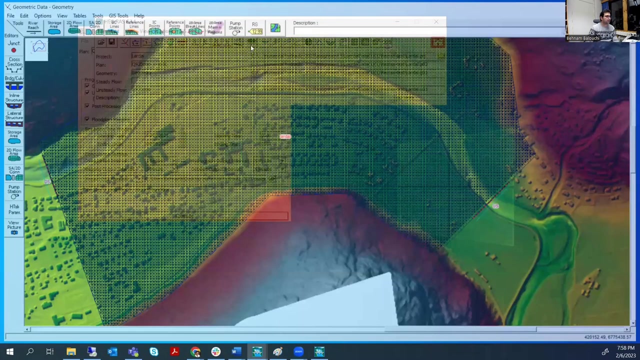 make it as before, then okay, then force to compute, then you can see we have a previous mesh and then save it. so then, after we delete the break lines, now we have a refine, we have a normal mesh, so i save it and then exit. so for the defining the refine. 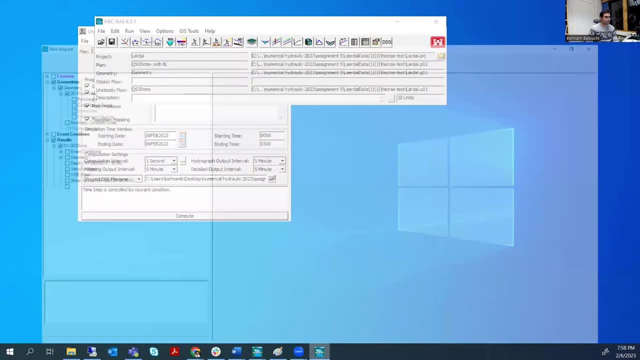 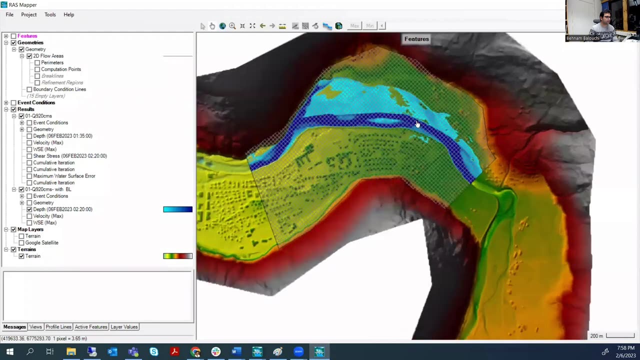 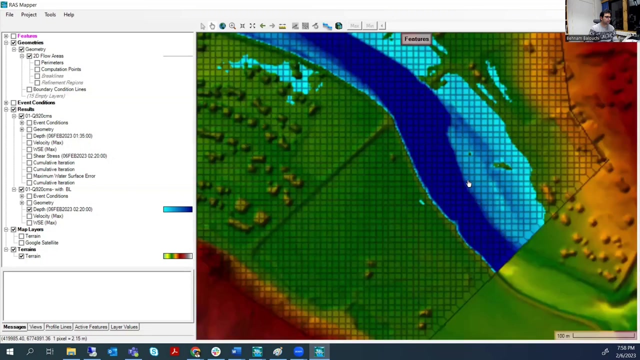 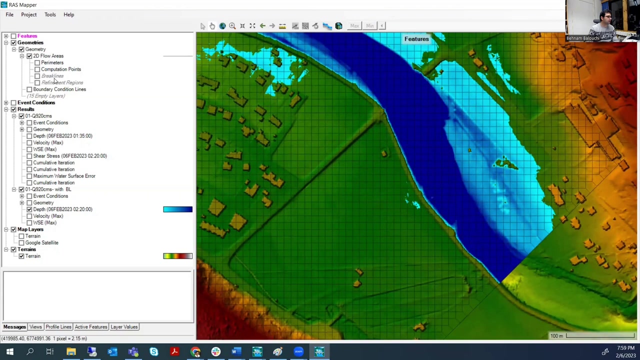 zone or define mesh and then exit. so for the defining the refine zone or define mesh, we should go to the RAS mapper and then geometry to the fellow area and then you can see break lines or refine mesh. I click here and right click edit geometry, or you have it here. 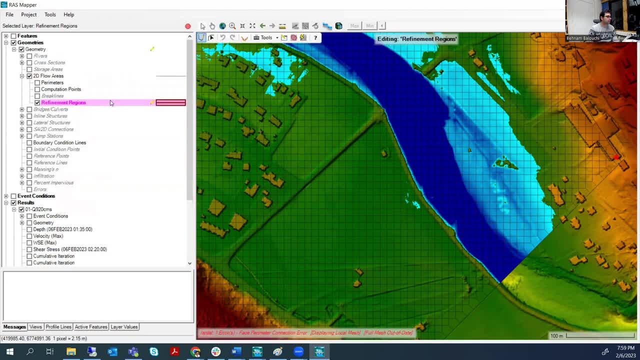 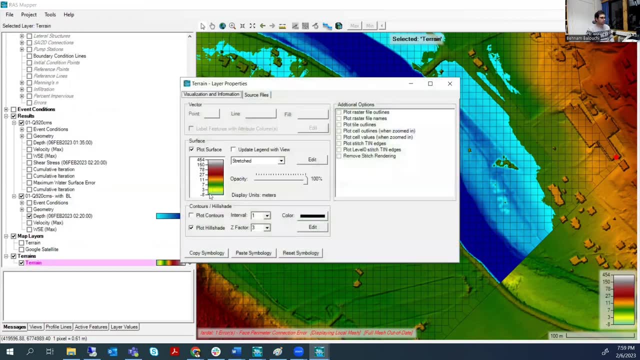 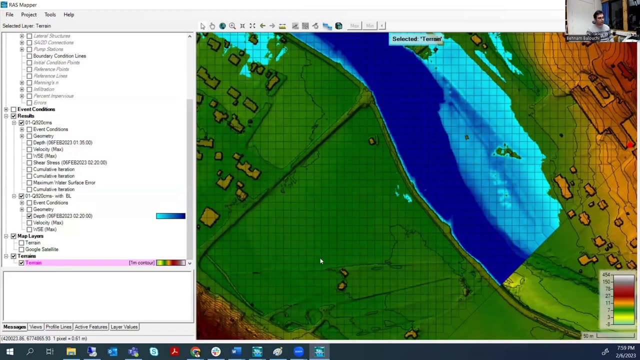 So we are going to the edit geometry. now we can draw a refine mesh. So for this purpose I told you that it is good to have a contour line. then I click OK. Now you can see we have a contour line. 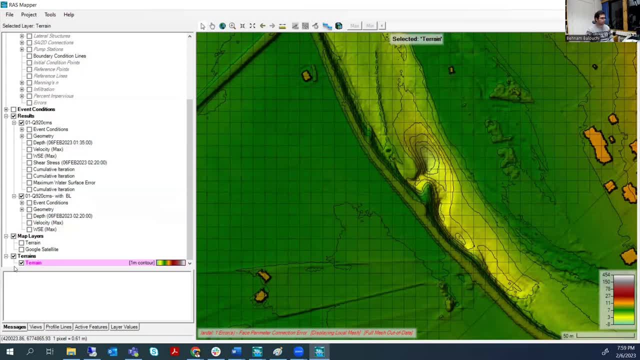 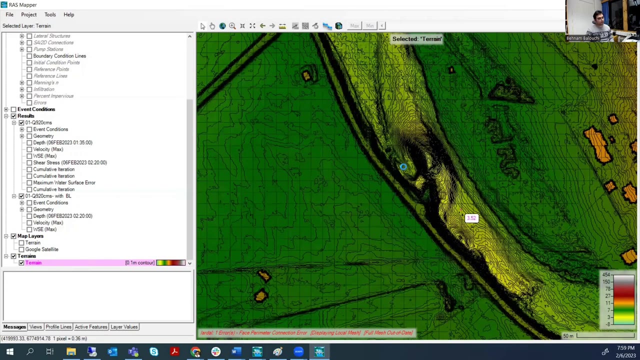 I can also turn off this. so it is better to have a like, of course, not to have borders, but those borders needs to be are separated out. So now you can see the refine mesh and also in the geometry. 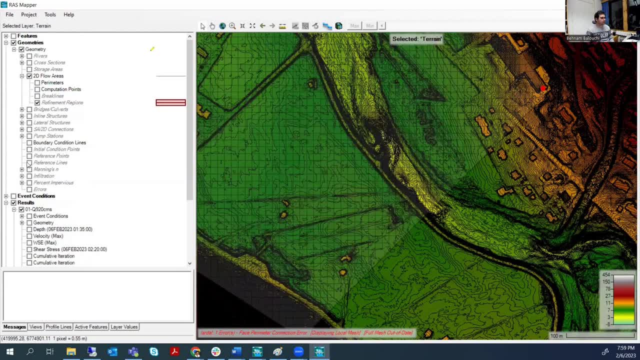 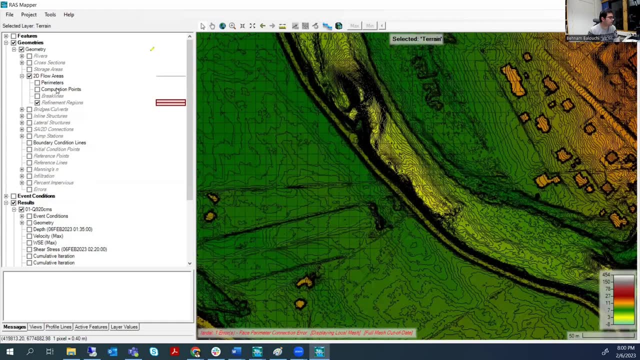 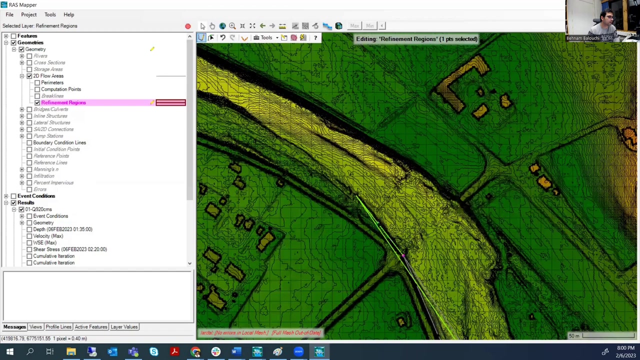 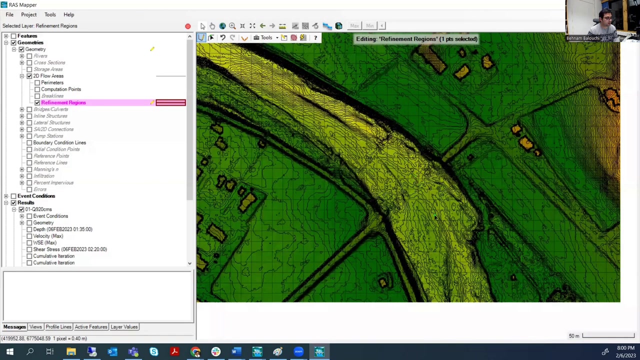 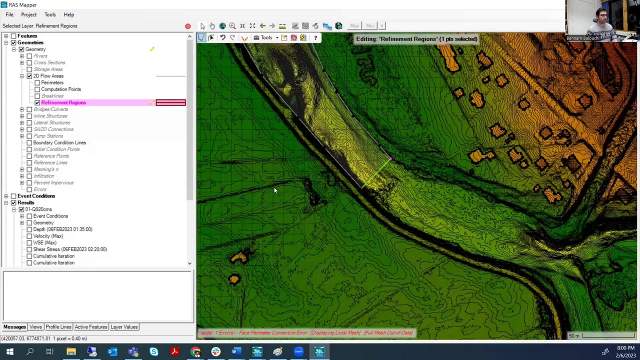 You can see the points or the area that we have. So for the defining the refine region can go like this: and we define area with water. I just defined this area to make everything faster and then double click, then you have a. this so region. I just call it as. 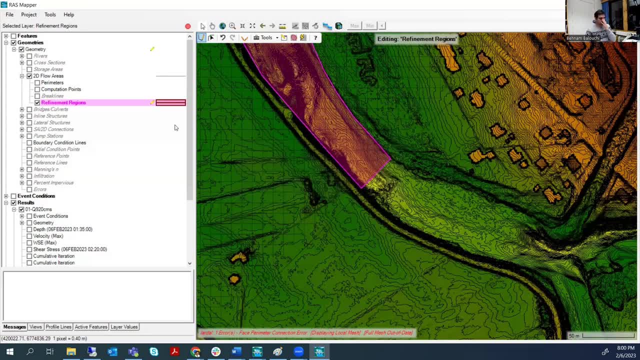 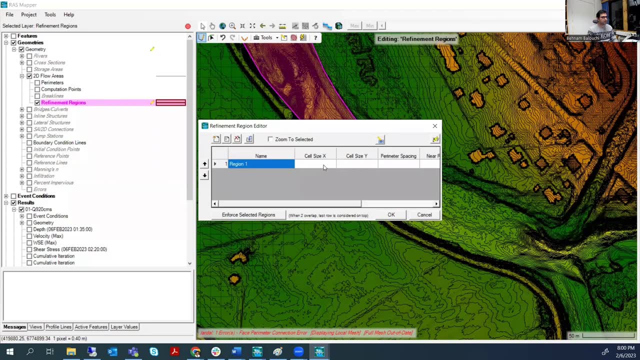 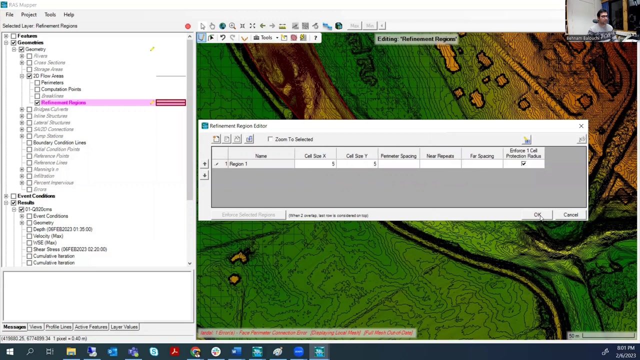 region 1 and then. okay. so now you have. you can go to the edit. you find regime properties, you can see the cell size. we can add it like five in X and five in Y. you can have a forest pacing near spacing. I think we can have it as 10 as 10 to be fast, and then you can go to. 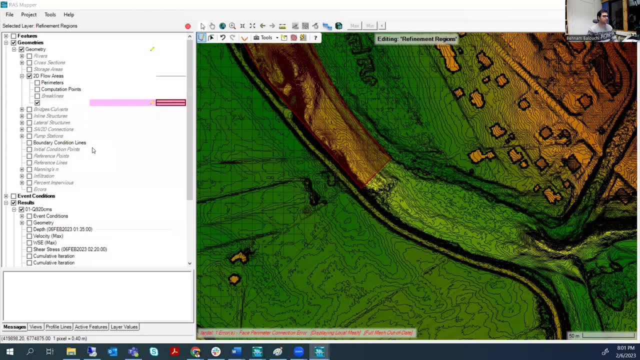 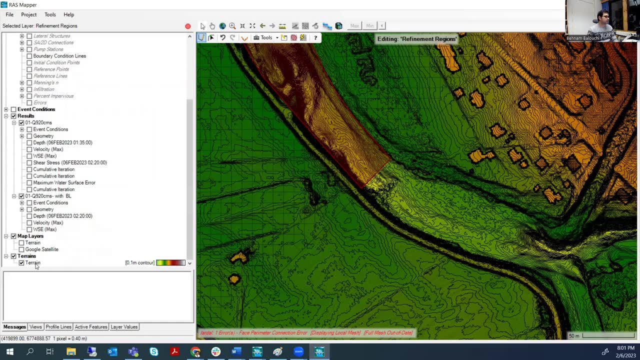 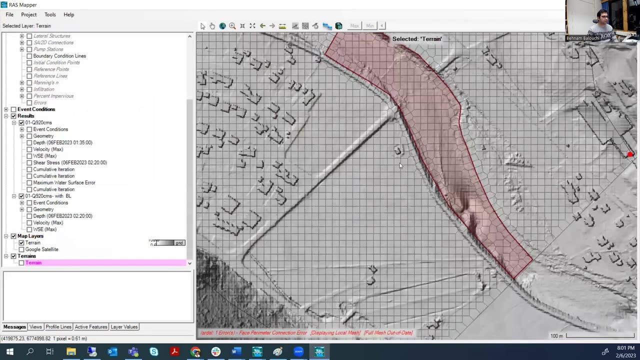 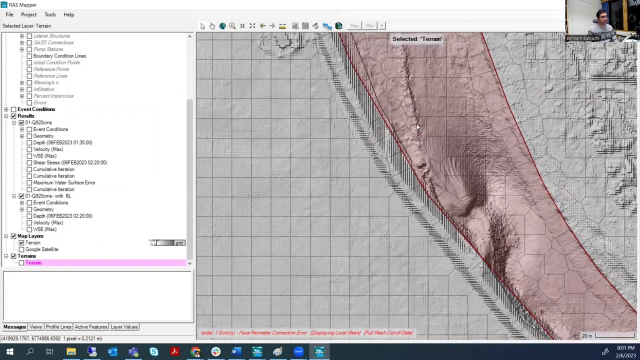 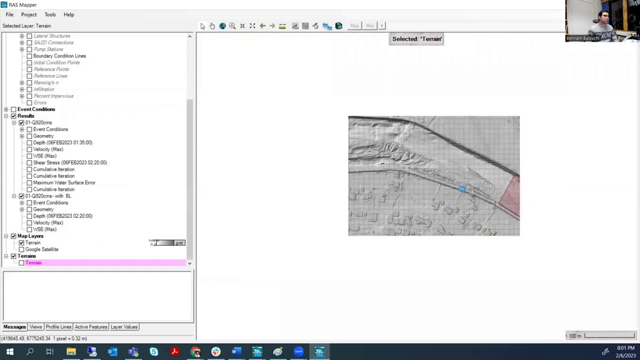 the enforce all regions and then have a this area. let me just turn off the layer, so we have this layer, so you can see the mesh start from this area and then it's again the same. so it is it is. I really recommend to continue it, because then you don't have problem. you to continue it, it's, it's sometimes. 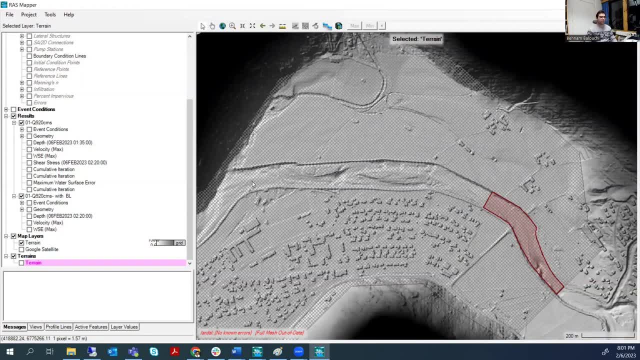 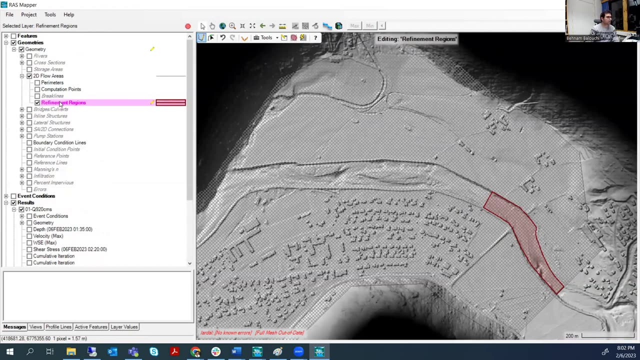 good for like a berated river. if you have that, you have values berated with low, with the course mesh or fine mesh. so I think I just want to show you how to work. so we just keep it simple as this, but you please remind that it is really recommend to continue it till here. and if I want to model, 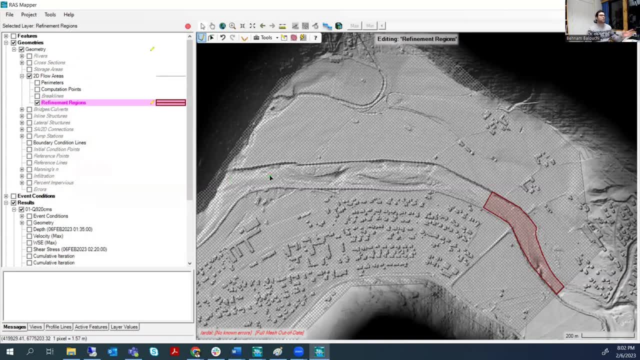 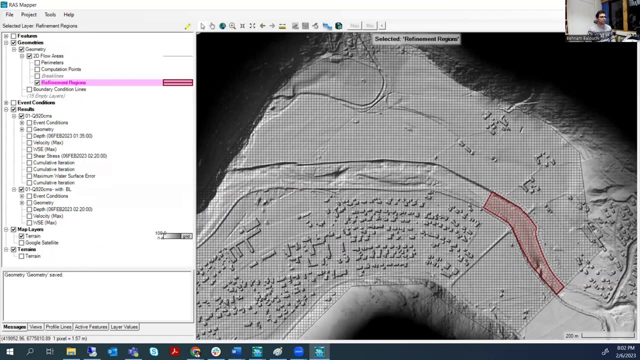 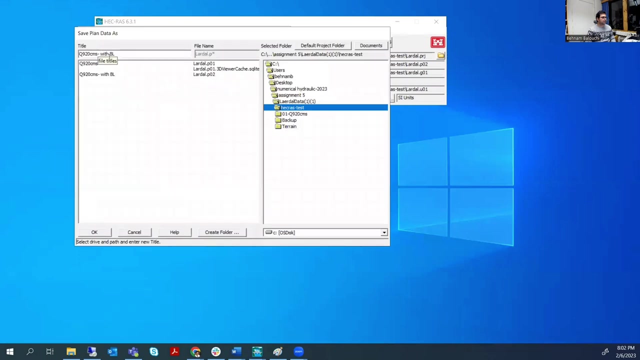 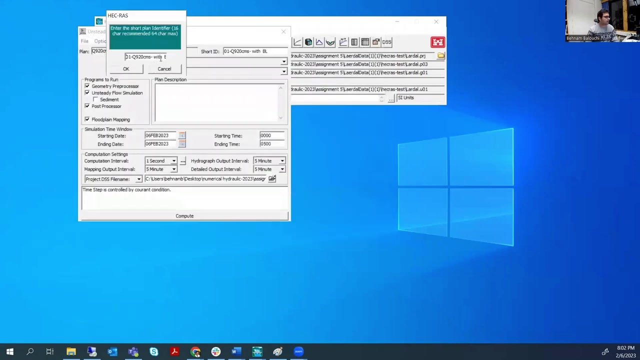 this with the refinement region. I will continue it to the end of the reach. so then stop, yes, save it, and then you can see it's saved, and then save the total and then exit. now here we can make a save plan as so with refined region, I just name it as RR- and here with 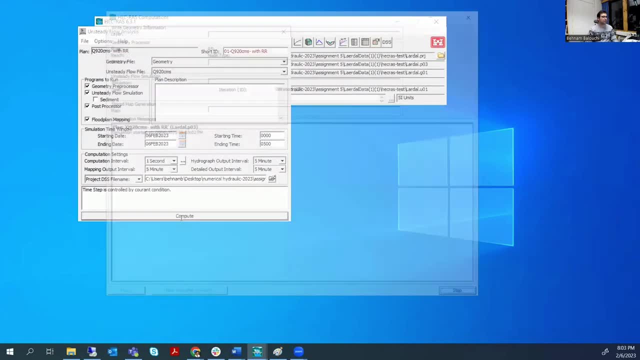 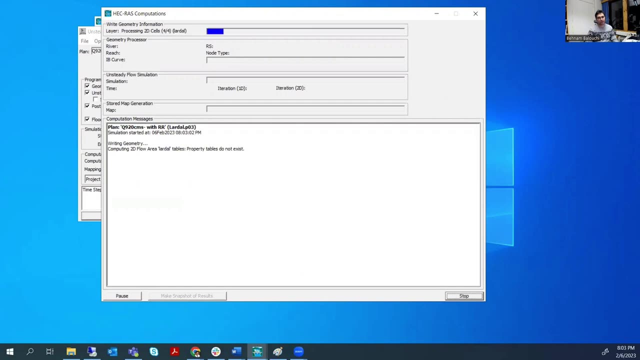 refined region, then okay and compute it. we can now see the effect of the refined region, if we have any errors or problem or if we can fix the that area that we had problem because of the cell size, mean there's sort of a current error or model. and then go to Pi and if I were to create some 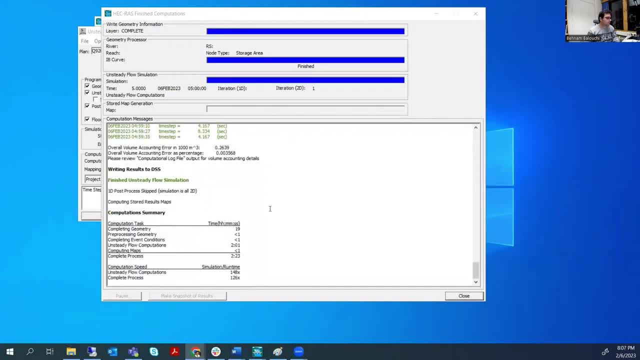 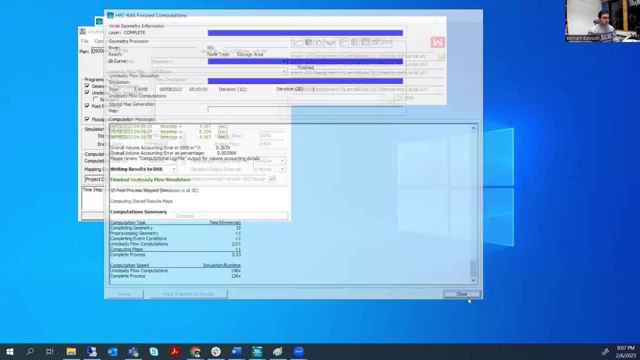 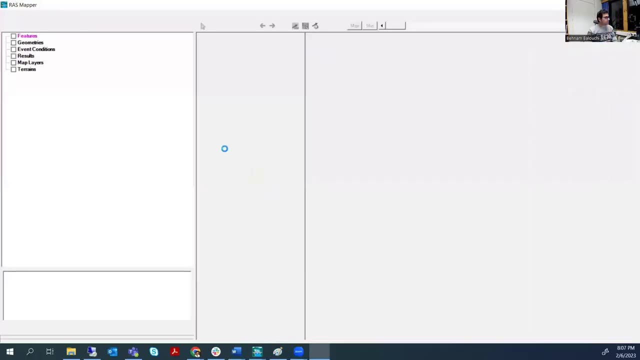 other something as an IP server. we need to make the tego Modal crises retee. then it's done. okay, now the run is finished. you can see the time I step and if you have attitude, so here. but if you model the sediments and you of erased and you have more challenges, then go to the rest mapper to see the results. very well, so here, so I try to. 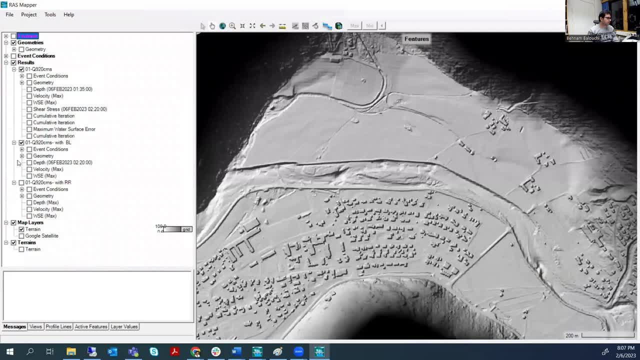 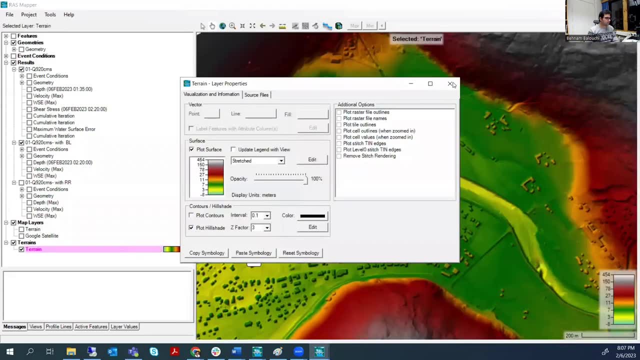 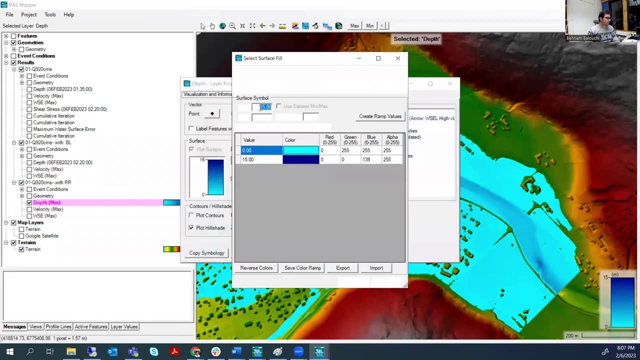 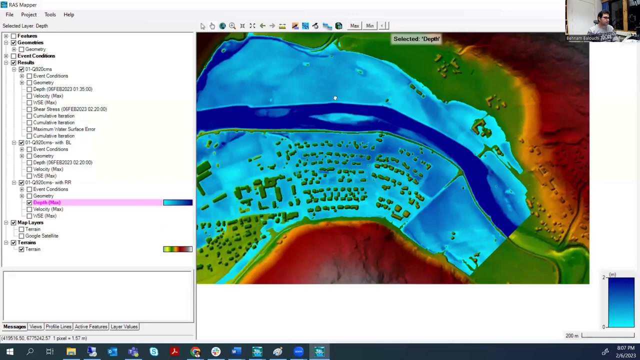 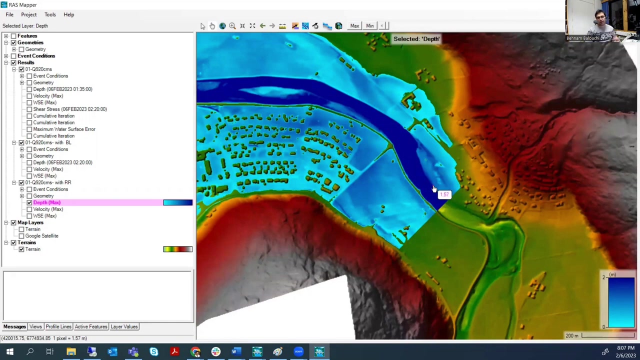 So I try to turn off the geometry, turn off this layer and then go to overtrain. So it is better to turn off the contours, And now it's with refine regime. Then we have depth And then make it as two create ramp. So let's see if again we have this problem or not. But anyway, if we have it or if we don't have it, it's a way of calibration. 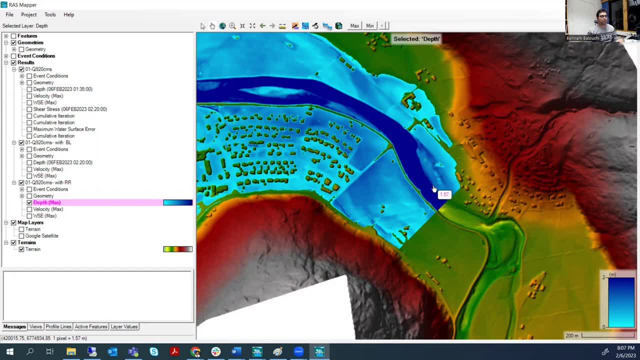 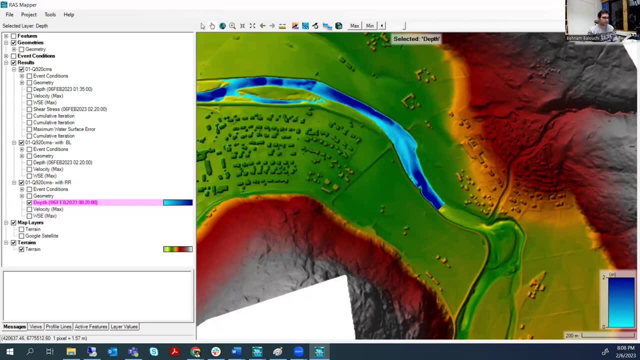 And the first step is you have to make a really good mesh according to your geometry and your train. So let's start. Okay, now we have again this problem, But, as you can see, it's again occurred in the previous time, But here we have it at two hours and 20.. So you can see the differences of these methods. 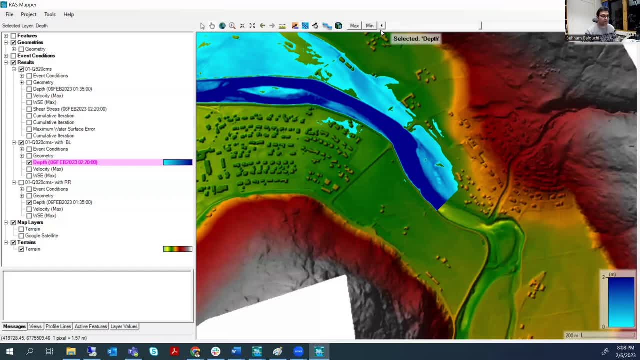 And the accuracy of them. So first, according to your river reach, I recommend to see what is the length of your river reach. For example, you can use the ruler and come here and see: Okay, what is it? You can see the length is 50 meters, almost 50 meters. 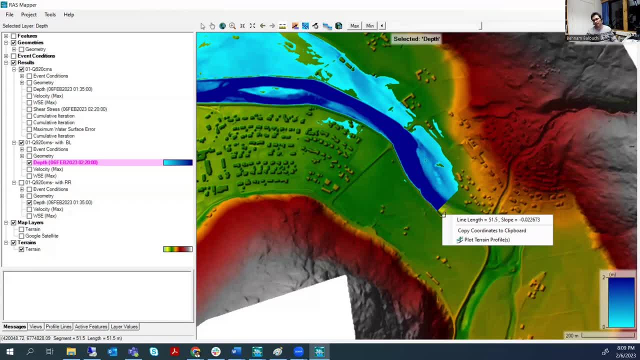 So a mesh like five meters or even 10 meters, maybe it's a good as a course- Mesh, of course- and then try to refine the center line of your river than the bottom of the banks and then the top of the banks. 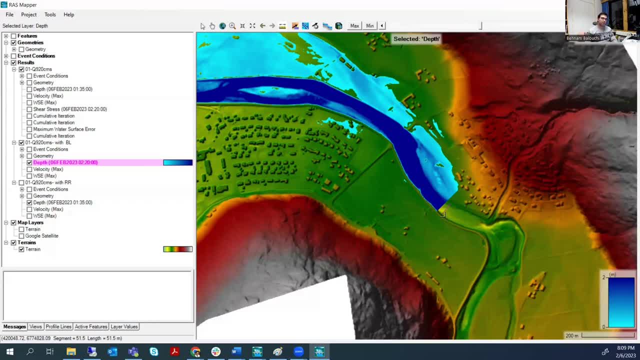 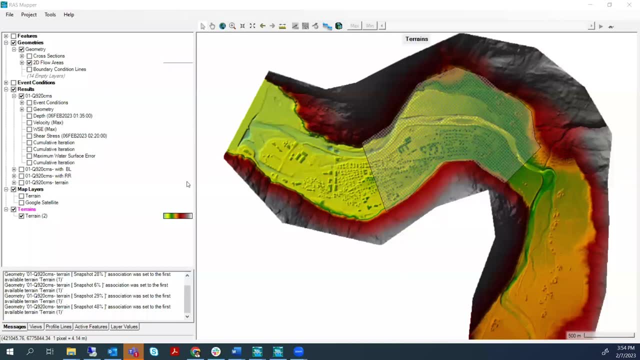 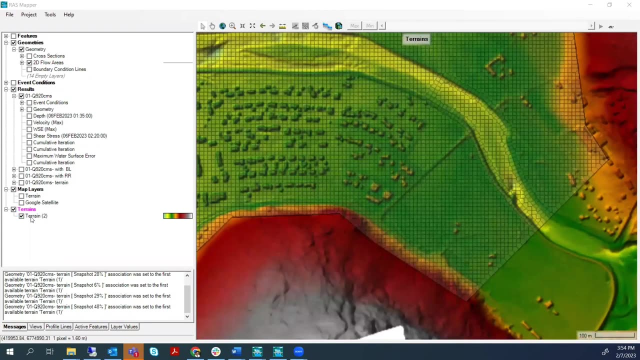 And then introduce the accurate flow data and run your model and enjoy your Modeling. So now I would like to show you how can we Modify the train So You can Right click on the trend and Use the cologne trend. 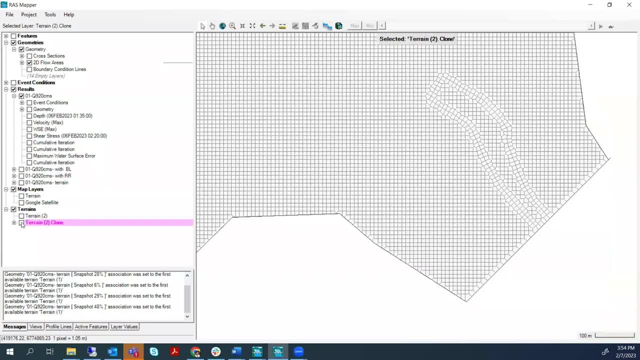 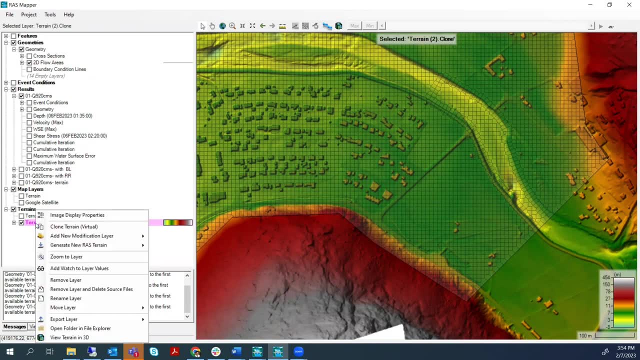 It's like a virtual copy of your train and you can change and modify it without Make any change on your real train. So if you right click on this and go to the add new modification layers, you have various shapes, lines, polylines to modify your train. 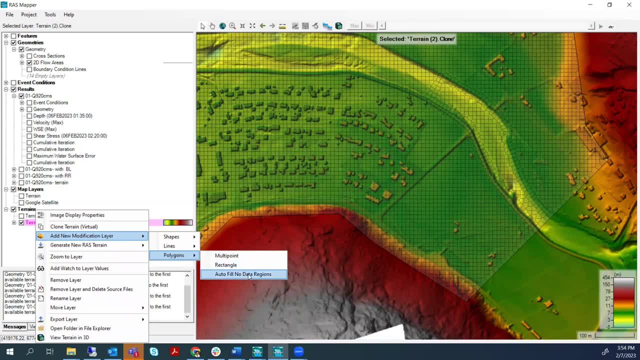 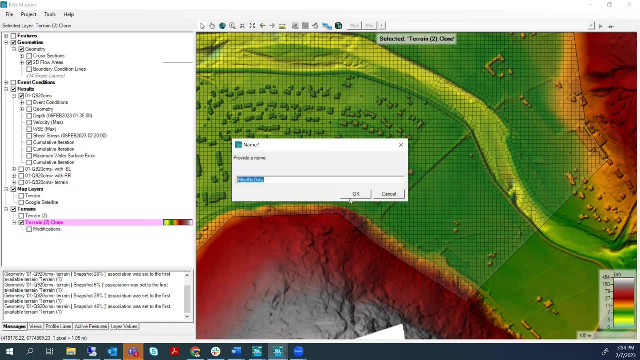 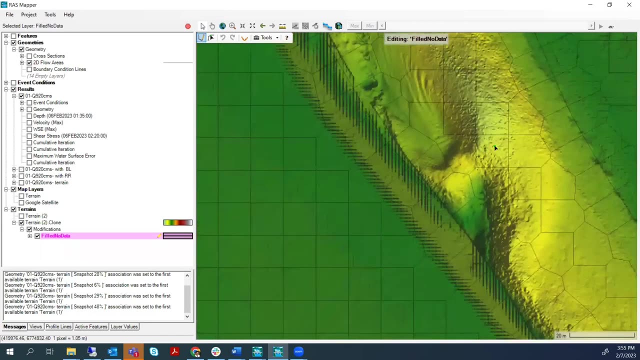 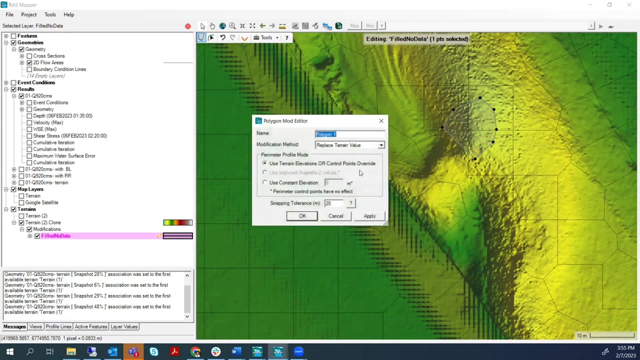 For example, if you have a All or a problem in your on your train, then you can use how to fill no data regions. then you click on it. OK, So we don't have any problem on this train. but I would like to show you, for example: imagine that you don't have a data here and you just make a. 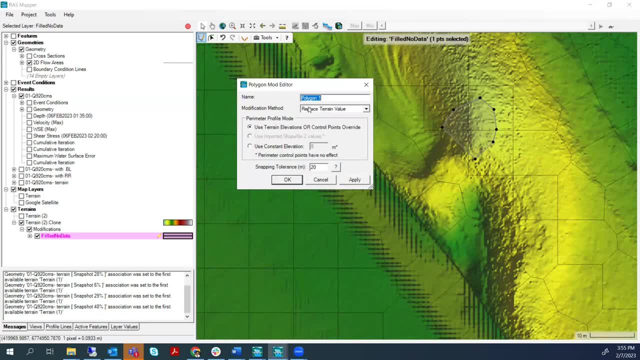 Modification and it used the elevation of the neighbors and interpolate the train. so you can choose a name And you can also choose the modification method. use the replace train values, higher values at constant values, Or here you can use the concept value, but these just keep the. 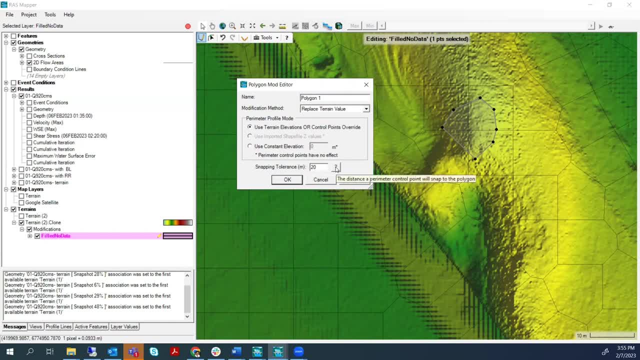 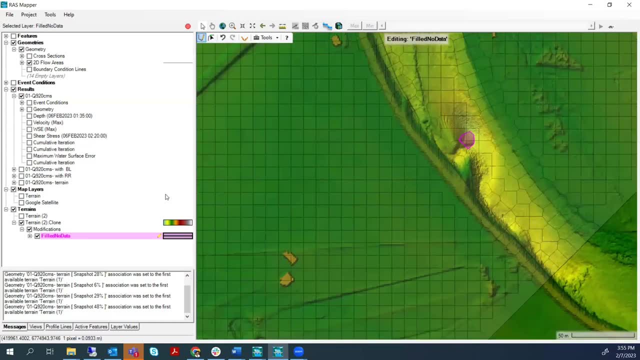 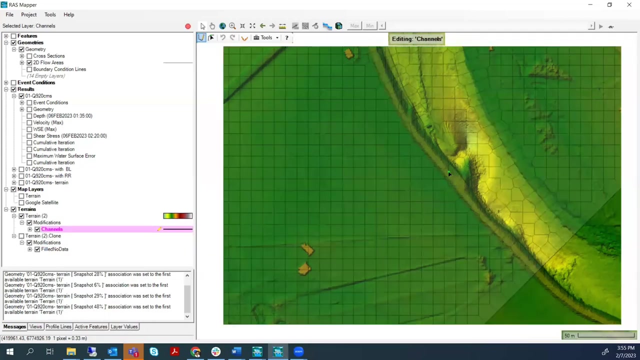 Default values and you can also always check by press F1.. What is this? parameters? So now I would like to run the model with the make a channel, so I just go to Train, then right click at new modification layer, go to lines and channels. 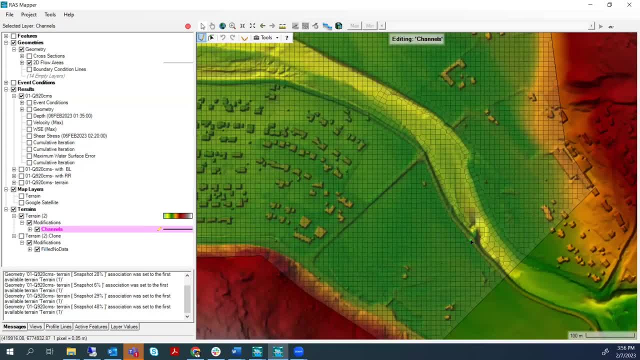 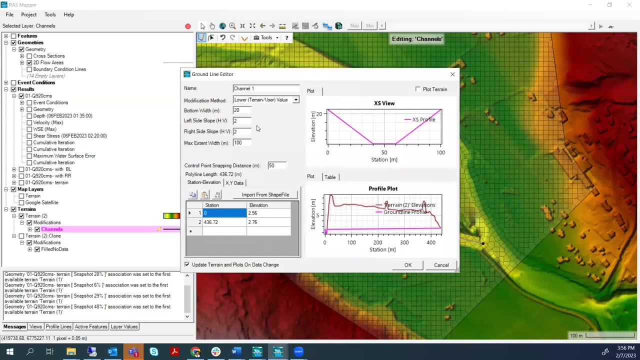 So, by a line, we would like to make a channel, so I would like to make it as here, So you can see the name and everything. for example, I like to change the with us 15 and make this as 3, 3, or this one as